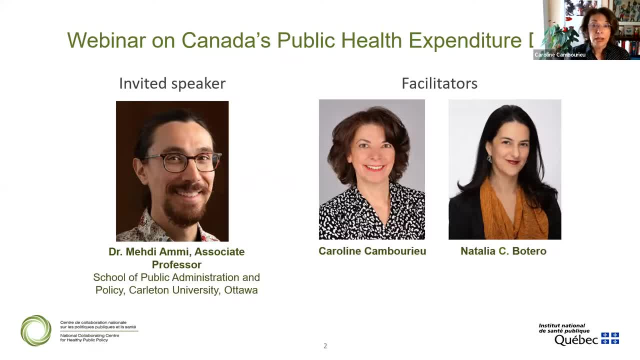 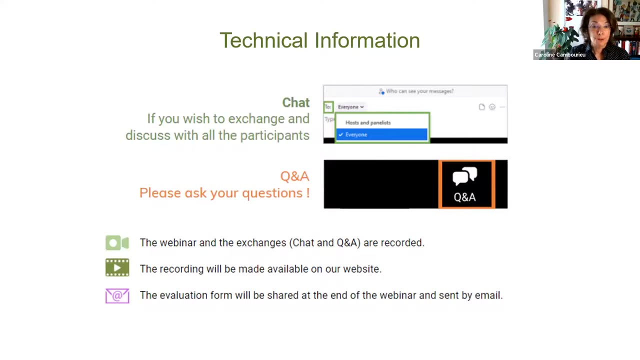 Mercier, who are also scientific advisors at the NCC-HPP and who will provide technical and logistical support. Before we get started, there are a few technical details I have to go over. First of all, the microphones and cameras of participants are. 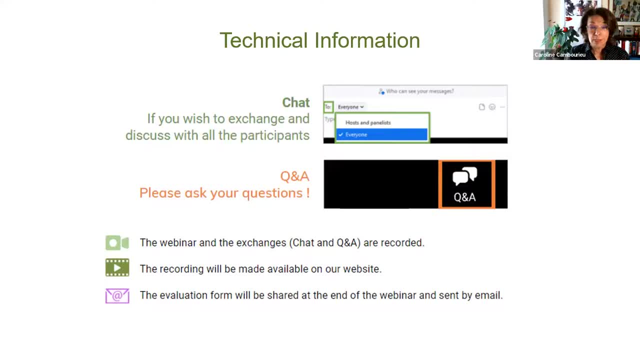 turned off. since there are many people attending this webinar To address questions to our invited speaker, we will ask you to use the Q&A function, which will also allow you to vote for questions you would like us to prioritize during the discussion period. You can also use the chat function if you want to share comments or resources with all participants. 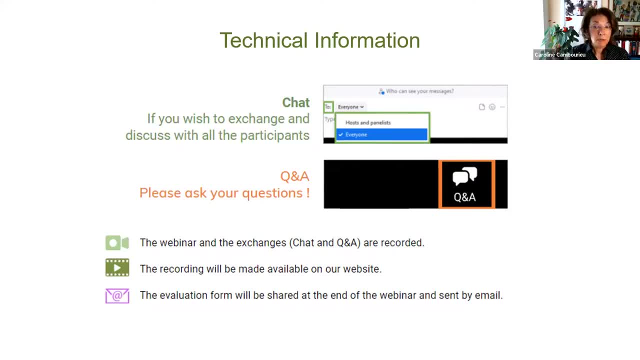 To do this, don't forget to select send to everyone, as shown on the right side of the slide. I want also to mention that this webinar is being recorded and that the recording will be made available on the NCC-HPP website within the next few days. 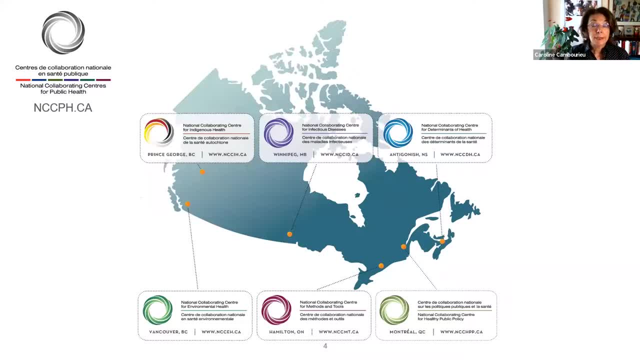 To begin, I'll just say a few words about the National Collaborating Centers for Public Health. a program of the Public Engineering and Public Safety Program of the National Collaborative Centers for Public Health. of the National Collaborating Centers for Public Health. the program of the Public Engineering and Public Safety Program of the national collaborative centers for public health. 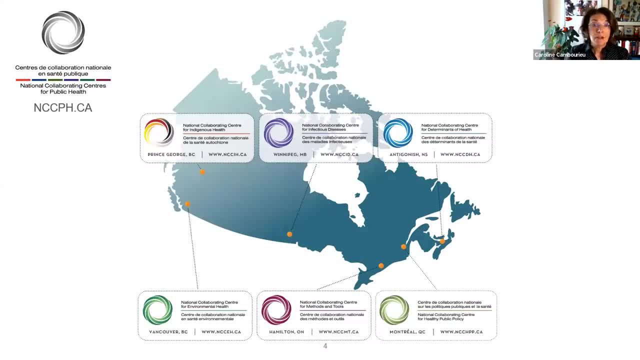 Health Agency of Canada. This program finances six national collaborating centers focused on key areas of public health, which are hosted by different organizations across Canada. The NCC HPP, for its part, is hosted by the Institut National de Santé Publique du Québec in Montreal. The mandate of the NCC- 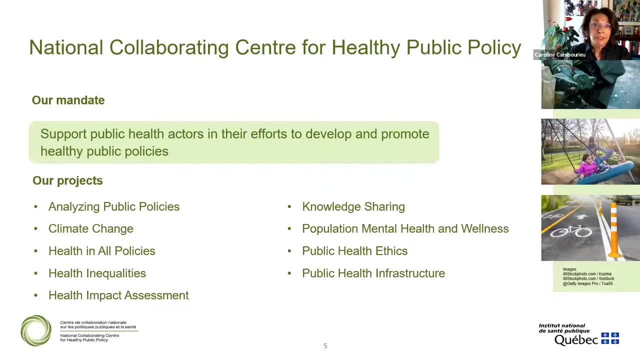 HPP is to support public health actors in their efforts to develop and promote healthy public policies, financing and funding of public health systems and, more specifically, public health spending, as we will see as an important role to play in that regard. On the slide you can see our main. 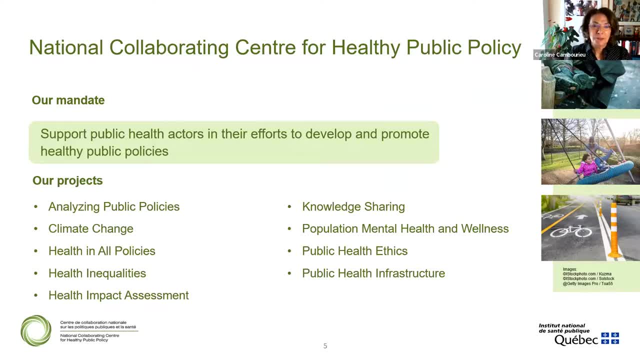 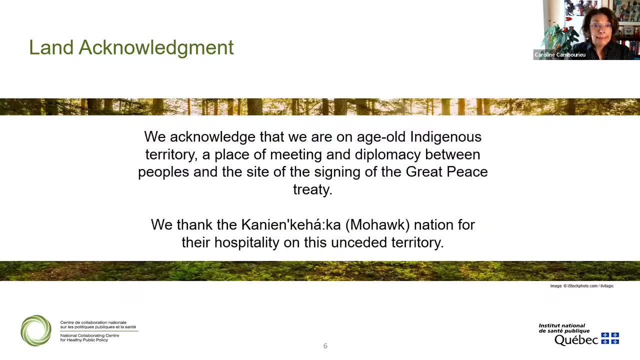 active projects. I will give you a few moments to review them. Since the NCC HPP is located in Montreal, we wish to acknowledge that we are on an age-old Indigenous territory, a place of meeting and diplomacy between peoples and the site of the. 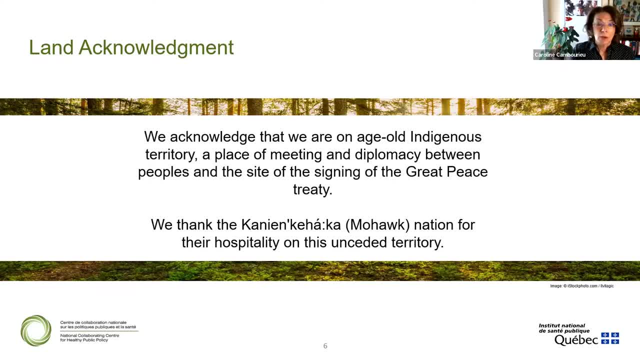 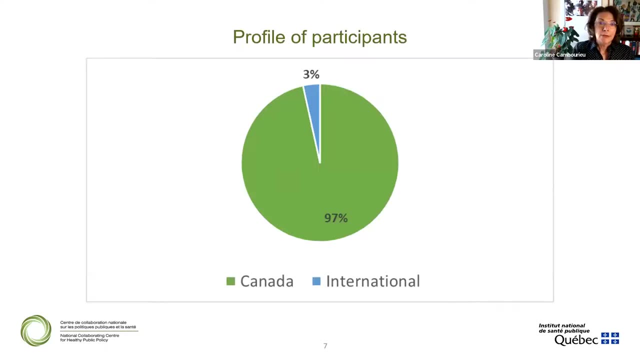 signing of the Great Peace Treaty. We thank the Kanien'kehá'ka Nation for their hospitality on this unceded territory. To give all of you an idea of who is attending the webinar with us today, I will just say that we had over 260 registrants. So 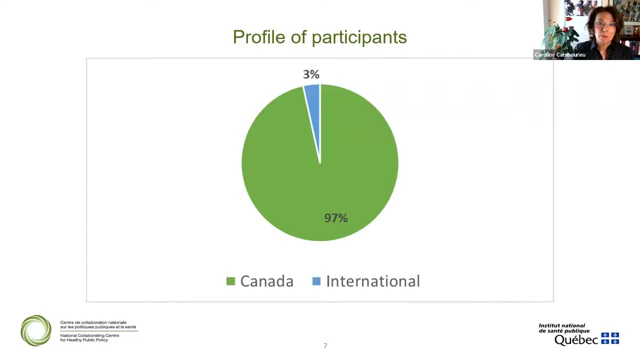 clearly there is an interest in the topic. Most of you, as you can see, come from Canada and we have very good representation from across the country and from different organizations. I'd like to take the opportunity to welcome all of you and to thank. 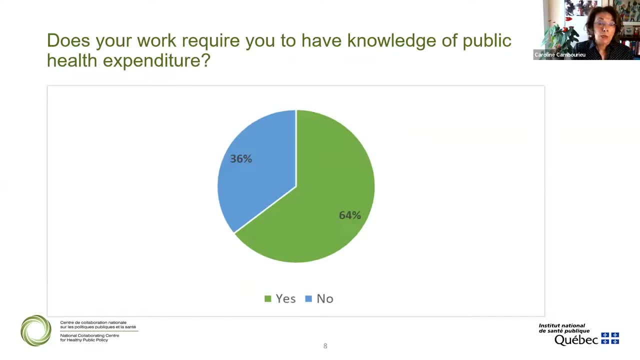 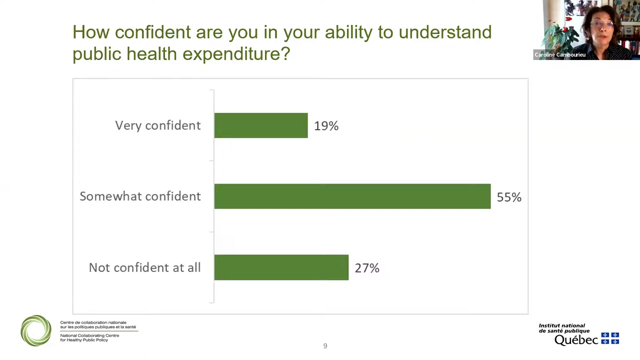 you for your participation. Thank you for joining us. When you register, we ask you if your work requires you to have knowledge of public health expenditure- And, as you can see, almost two-thirds of you are required to have it. We also ask you how confident you were in your ability to understand. 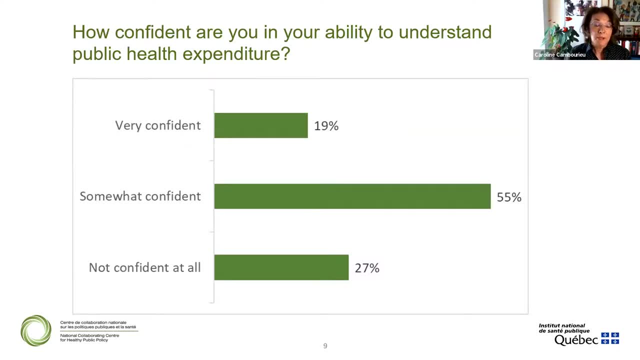 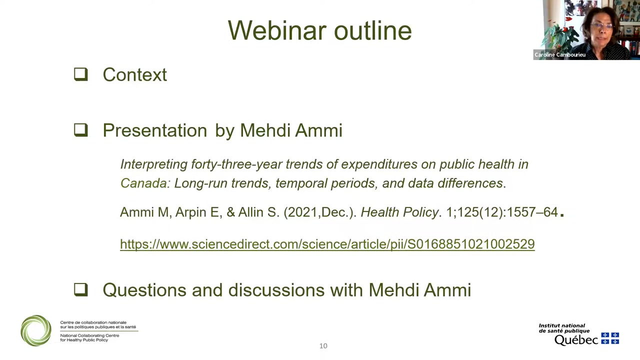 public health expenditure. The majority indicated somewhat confident And almost a fifth responded very confident. We thus have with us today people who are interested and who are knowledgeable about public health expenditure, So the conversation should be very interesting. This slide presents an outline of the webinar Following my 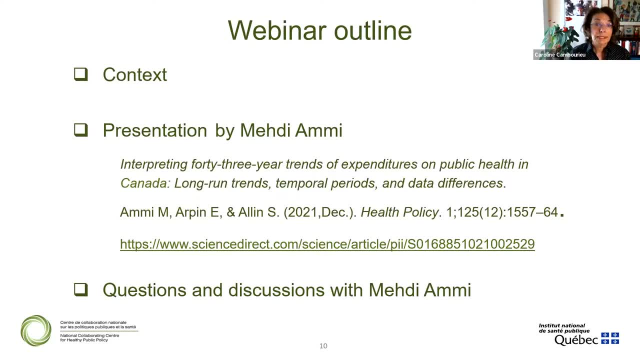 introduction to set the context. Dr Mehdi Ami will present key findings from his project conducted with COVID-19.. He will present key findings from his project conducted with COVID-19.. Dr Mehdi Ami will present key findings from his project conducted with COVID-19. 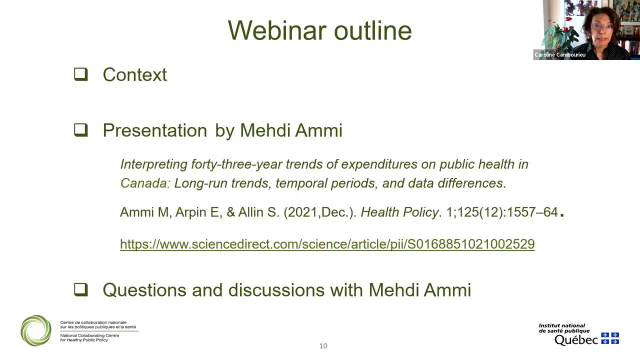 And he will present key findings from his project conducted with colleagues Emmanuelle and Sara Aylin, which was published published in health policy in December 2021.. This presentation will be followed by a question and discussion period during which we will ask Dr Mehdi. am I to respond to some of the questions? 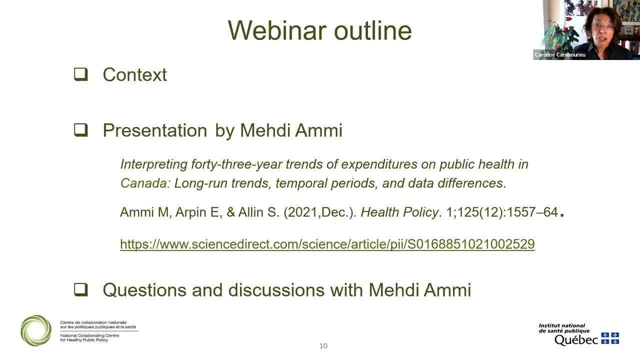 you propose when you register and to some of the questions you will put forward in the q&a During the webinar. so Please participate in the forum is to Ashanti. So please don't hesitate to submit these as they come to mind. 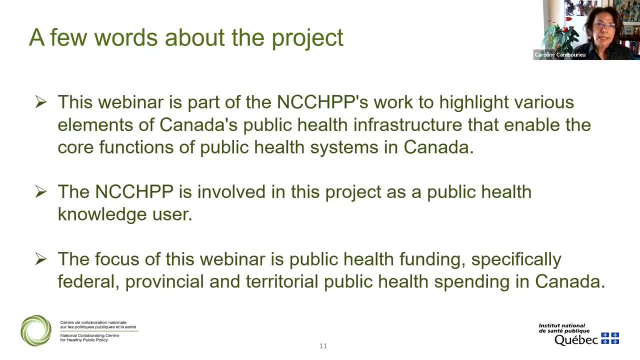 By way of context, today's webinar is part of the NCC-HPP's work to highlight various elements of Canada's public health infrastructure that enable the core functions of public health systems in Canada. The NCC-HPP is participating in this project as a public health knowledge user. 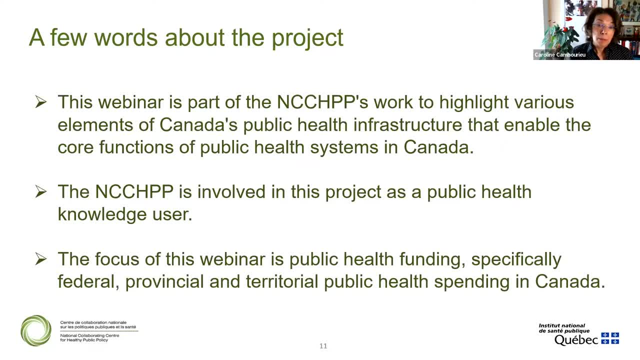 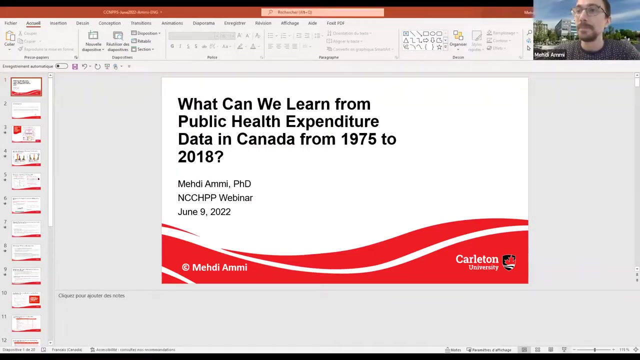 The focus is on public health funding and, more specifically, on federal, provincial and territorial public health expenditures in Canada. Without further ado, I will turn it over to Mehdi to tell us about it. Mehdi, please, Okay, Hi. Thank you, Caroline. I'm just going to share my screen. 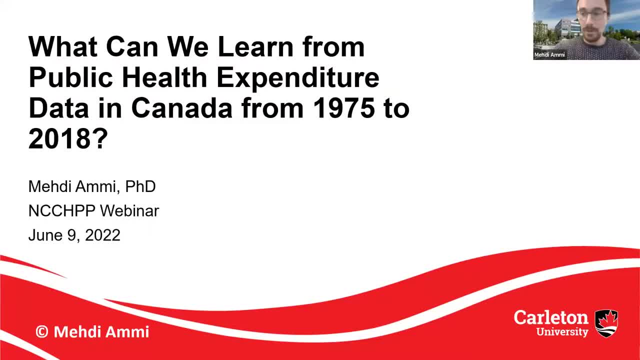 Okay, So you should normally all see my screen. I'm just going to set my timer. And well, thank you for the invitation. Thanks to the NCC-HPP for the organization. I see you. I see there is a good turnout today, so thank you for attending. 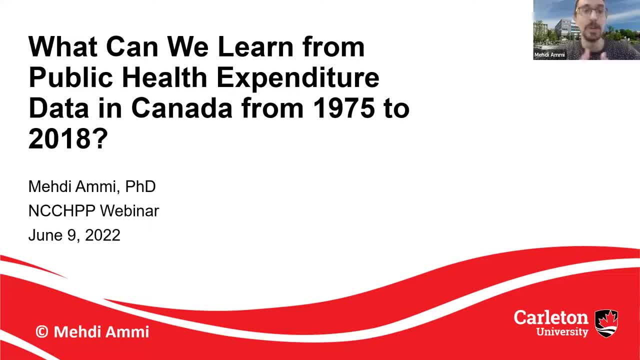 I'm Mehdi. I am an Associate Professor of Health, Economics and Policy with the School of Public Policy and Administration at Carleton, which is in Ottawa. So I'm not at Carleton right now, even though my background pretends I'm on campus. 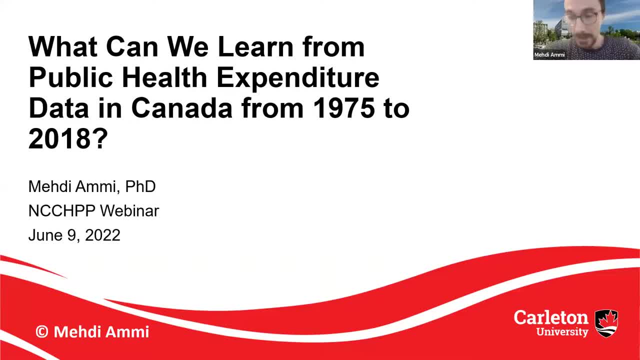 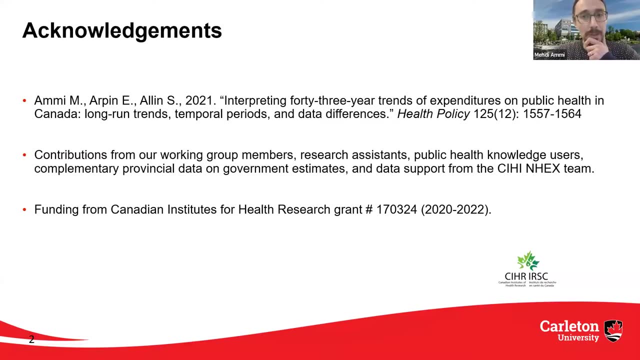 I'm, however, in Ottawa, which is located on the unceded and traditional territory of the Algonquin Nation, so I wish to acknowledge this. This presentation is really to try to give you an overview of one paper that has been recently published, which you know Caroline already mentioned. 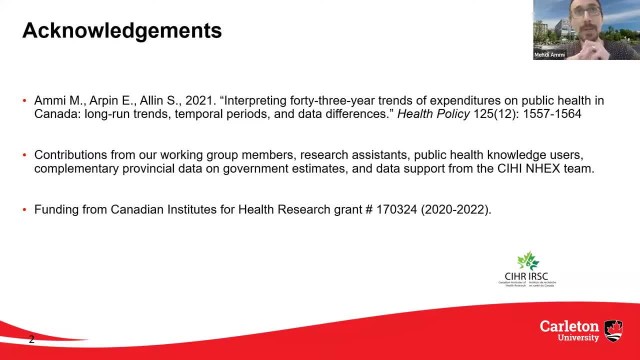 This paper, joined with Emmanuelle Harpin and Sarah Allen. It's an open access paper. I really invite you just to access, download and read the paper after this presentation if you wish to, And before I start the presentation. you know I have to go – I mean it's important that I go, It's not I have to. 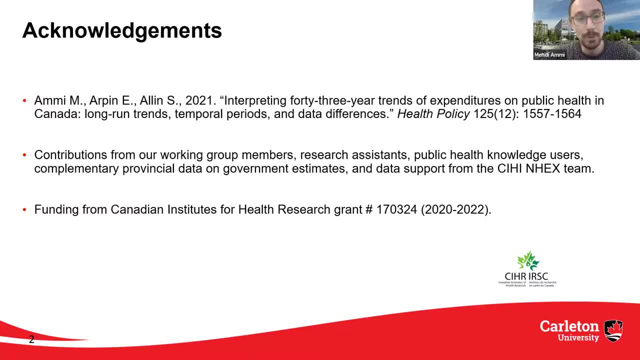 I wish to go through a round of acknowledgments And fortunately, to all the people who have been contributing to this project. So, more broadly, this is part of the research agenda about public health expenditure, public health financing, where there is a real need to build capacity, actually in Canada. 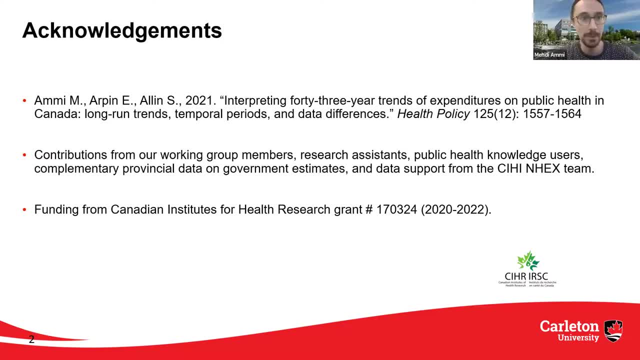 And I know there are not many health economists in Canada. There are even fewer that are just like looking at this question of public health And, as I was just trying to make a case in motivation, this is obviously something I believe is extremely important to do. 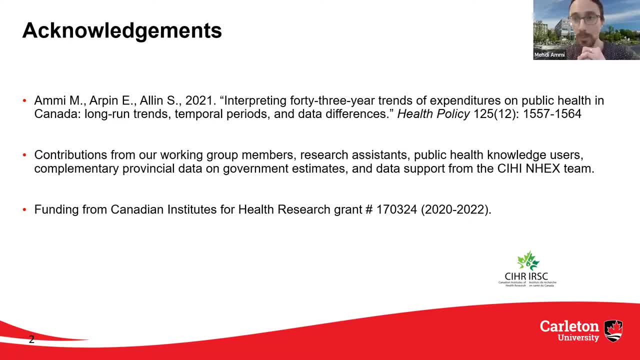 So, just looking at this question of public health, So just thanking all working group members, research assistants, public health knowledge users, So this includes the NCC HPP and, in particular, Olivier Bellefleur, who has been really, you know, a very consistent and helpful participant in this project. 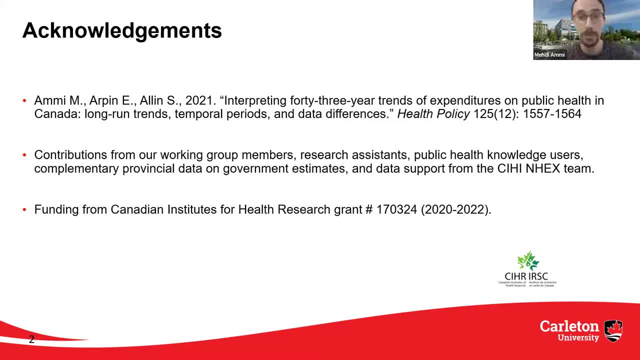 We got also some data from another group who is working on this question, and the data support from CHIA. So CHIA is the Institute of Health Information, And we have also been lucky in receiving funding from the NCC. Thank you, 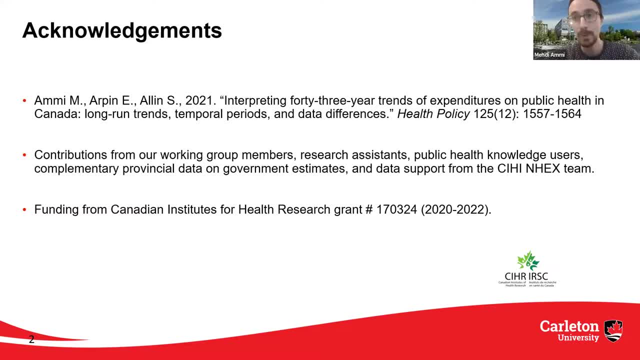 And there is also also a lot of additional funding from the NCC Health Research. The grant number is on the slide, which has helped us support and actually complete this project, and there's more to come. I will just talk about that at the end. 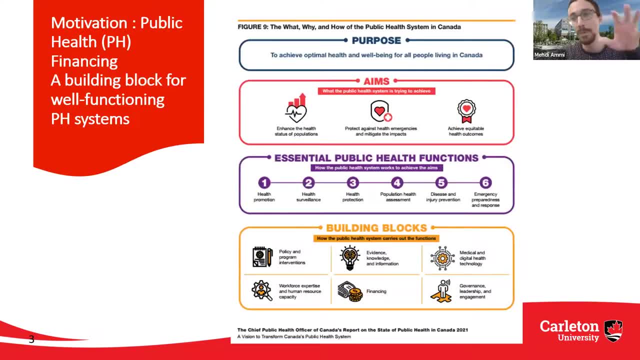 But first this paper in particular. I mean some of the highlights of this paper. And the first thing just to clarify this is a seminar from the NCC HPP. However, I feel it is important. there is frequent confusion between public health expenditure and expenditure from public source. 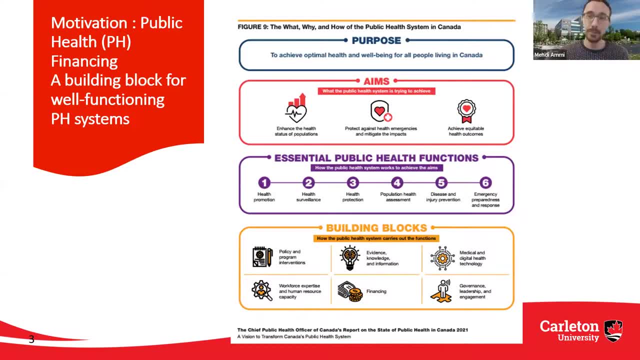 So health expenditure from public source. here we talk about public health expenditure. So public health broadly speaking. you have this on the slide there. it's a diagram that comes from the CPHO report. so the Chief of Public Health Office of Canada from 2021,. 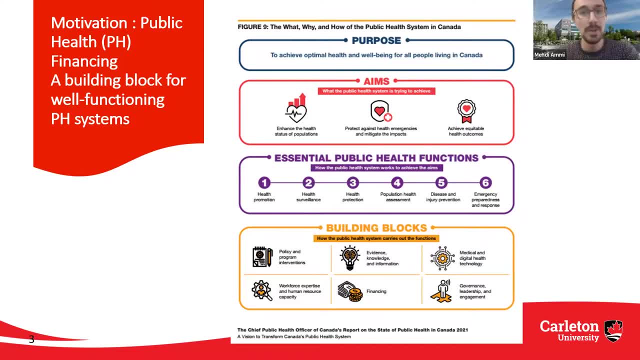 December. so the latest report, which just essentially says the mission of public health is enhance the health of the population, achieve equitable outcome and protect against health emergency. There are, like five functions in Canada, six main functions for public health. they are: 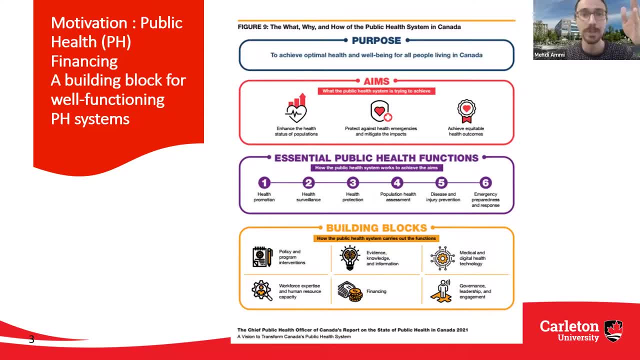 listed there: health promotion, health protection, health surveillance, assessment, disease prevention and emergency preparedness. So that's what public health is about, And what the report was just trying to highlight is this kind of renewal and a vision for the renewal of public health systems in the future and what they were in Canada. 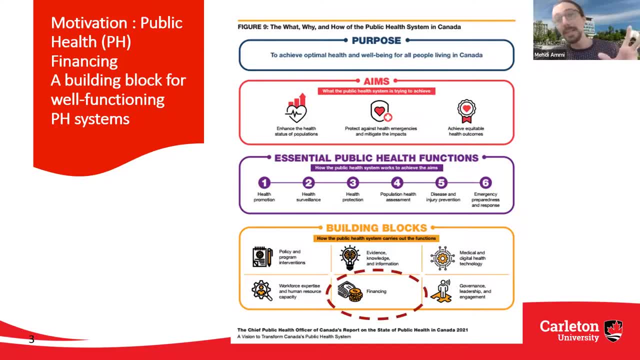 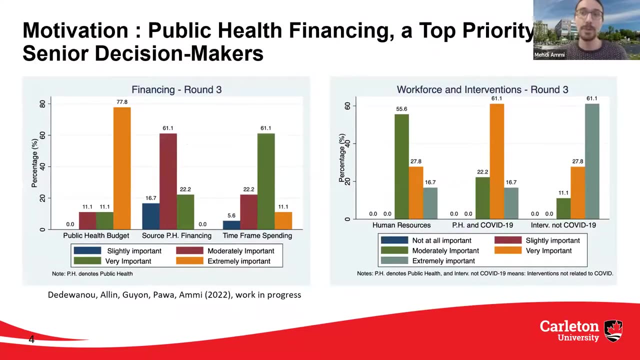 Obviously this is a Canada report, but what they were highlighting is one of the building blocks that we need for this public health system to function well- is financing. And just to further this motivation, this is part of a Delphi exercise, so a kind of 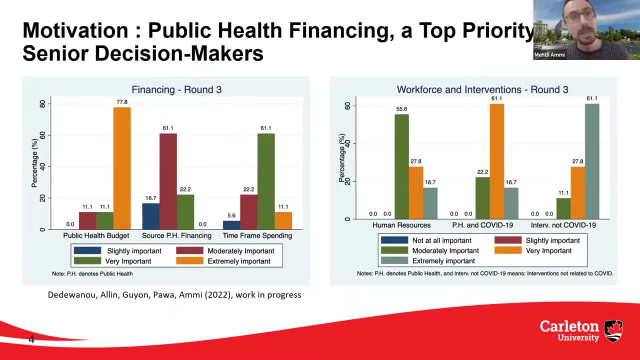 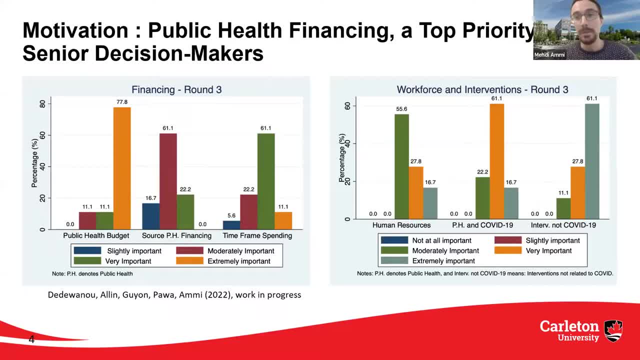 So let's say, managers who are in positions just to affect the health of the population, What do they think are top priorities? And you know, after three rounds we're just like not going to go into the gist in the details of it, but the gist of it is: after three rounds, we like we see this consensus. 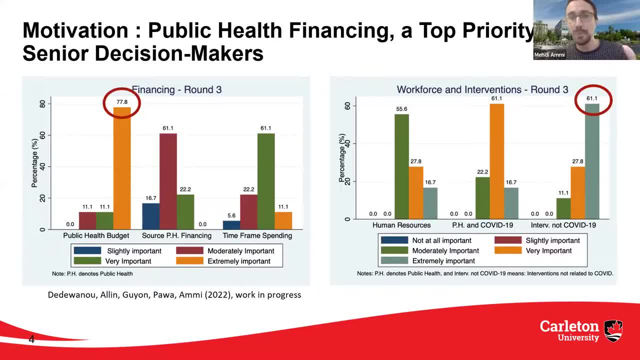 And what was very clear is, you know, this consensus of extreme importance of the public health budget, like the large majority agreed, And it's even higher than looking at something that is a major concern for public health practitioners- I mean the one I'm, at least. 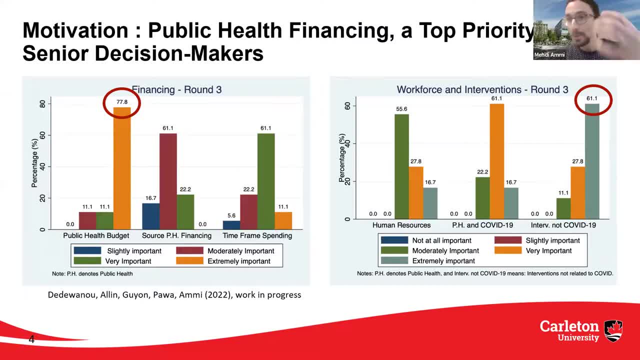 from the one I'm regularly talking to, the commentaries I've been reading, which is essentially being sure about the public health system: doesn't become a system focused on chronic global disease, you know, and emergency preparedness, but all the function of public health. 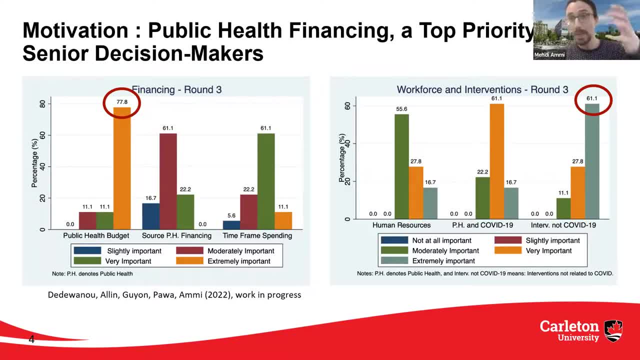 and to be protected. So even that is trumped by okay, we need budgets, you know, public health financing, to do what we are, to achieve our mission. essentially, That's what the message is. So some background about public health funding or spending. 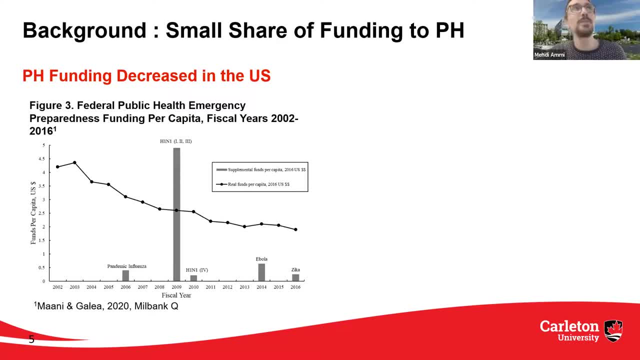 What one important feature. so I was not able to find a good translation from what we call in French, which is essentially saying that this is the one that gets the least. you know, but the point is that there is a small share of funding. 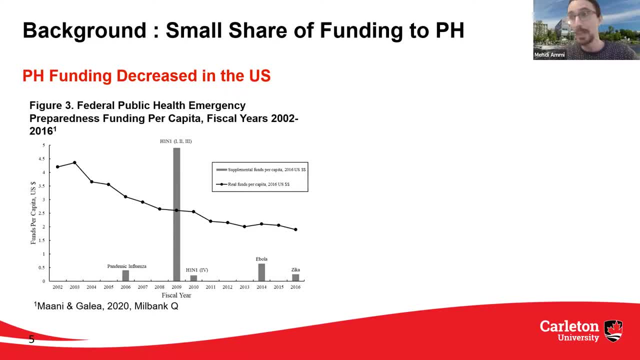 that goes to public health across the board. So in OECD countries the average is about 2%. so 2.3% in 2019, but about 2% just. you don't need to remember the decimal. that goes in public health. 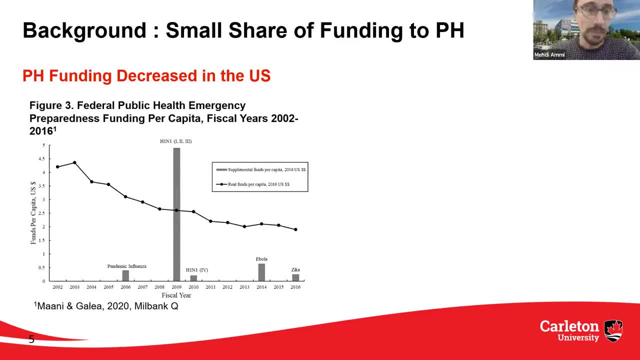 So really tiny bit when you think about the health system in general. But what has been a cause for concern in different countries- so there this is the example of the US- is that this already small share was actually decreasing. So you see that, coming from the federal level, 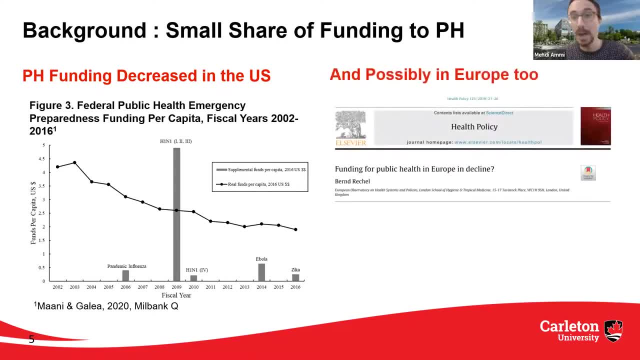 in the United States. So there are some evidence that it's possibly the case in Europe as well. So this paper by Ben Trinchel possibly. I'm going to clarify why in a second. And what is really interesting is that in Canada. 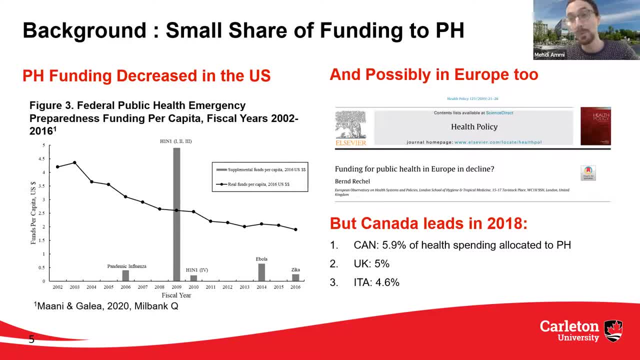 we're actually the top spender in terms of allocation of health resources towards public health, And what you see on the slide is like: so, when you look at the comparison, 2018 is the last year that has been like validated for international comparison. 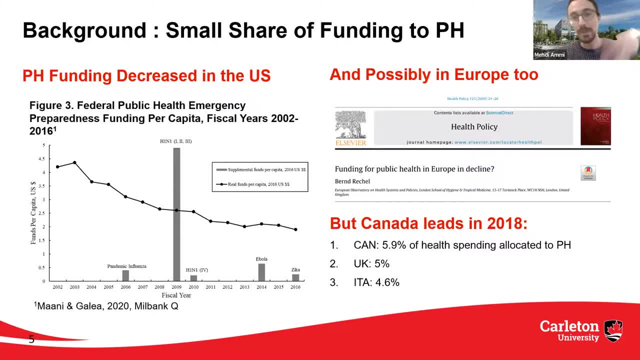 But if you look at Canada, you see that it's like you know, like Canada, we can go up to 2020, but the studies use 2018 data as the last year, So I'm just going to talk about 2018 as the last year. So Canada, about 6% of health spending goes to public health, which is one percentage point higher than you know, the UK, where it's 5% And you know also higher than Italy, 4.6%. So there are like the top spenders there. 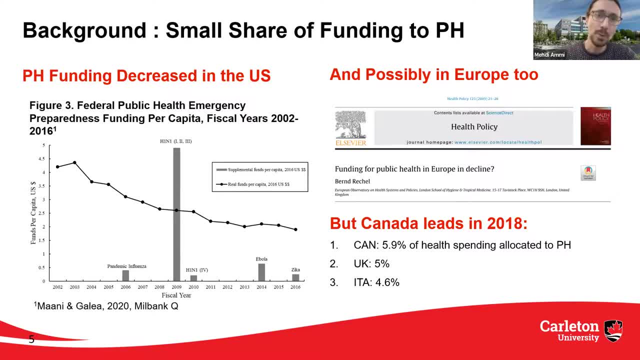 Again, obviously the average 2%. So what we are really trying to understand is: well, how did we get there? You know, how did Canada manage to be, you know the well- the country that allocate most of its resource? 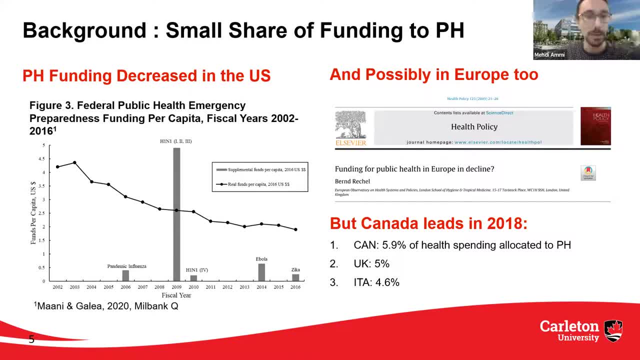 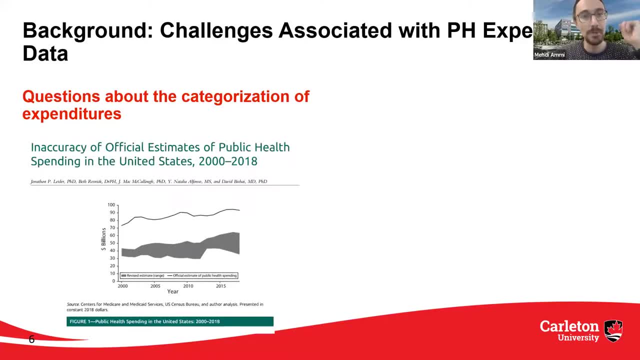 of its health resource to our public health, compared to other industrialized countries. Then there is this question of you know well, okay, that's the first part of the story. The second part of the story is that it looks like there are some difficulties. 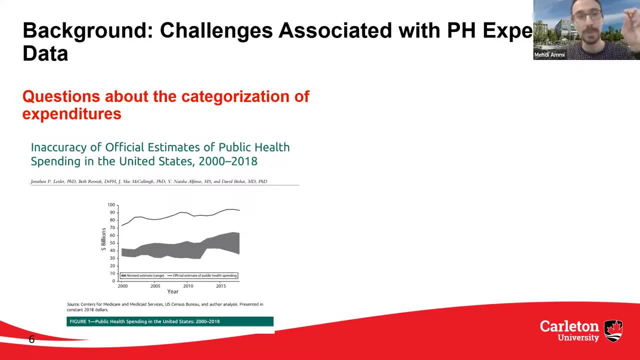 You know, when you try to measure public health expenditure, you know what is the most important thing. So the left panel there is just talking again about the US and it's still at the federal level And what Lader and colleagues there have been doing. 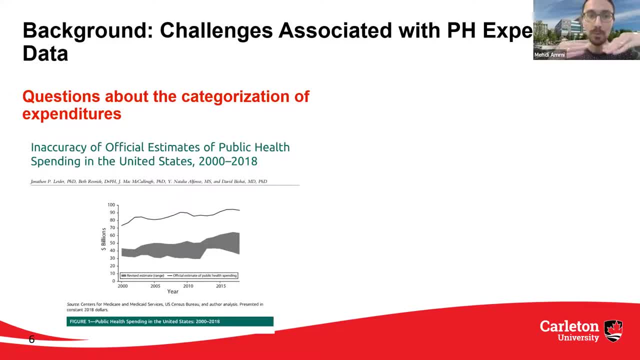 is they're just trying to see you know whether what is reported as public health is public health according to them, And there is some discrepancy between you. know what is officially reported and what they estimate there. you know, with this kind of margin of error. 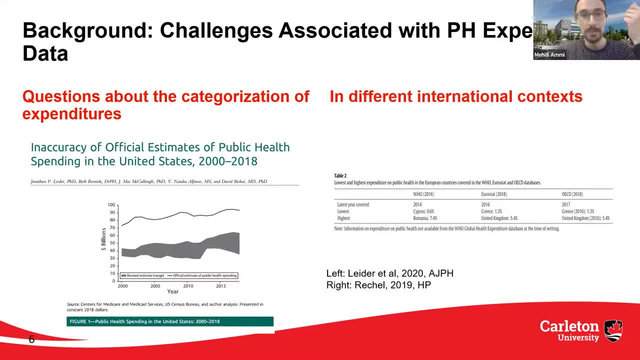 If you look at Europe- so that was this point of Rachel, and particularly like the first two column for illustration- if you see there, you see that the country that spends the less on public health is Cyprus, but according to the EU, but according to Eurostat. 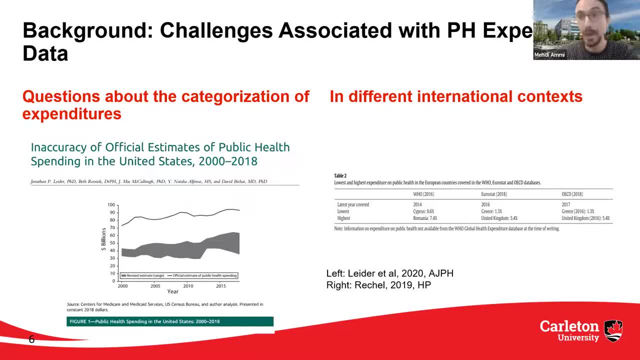 which is, you know, the European agency of statistics. that's going to be the easiest way to describe. it is Greece, And then the top country according to the EU is Romania and according to Eurostat is United Kingdom. So we just see that there might be some difficulties. 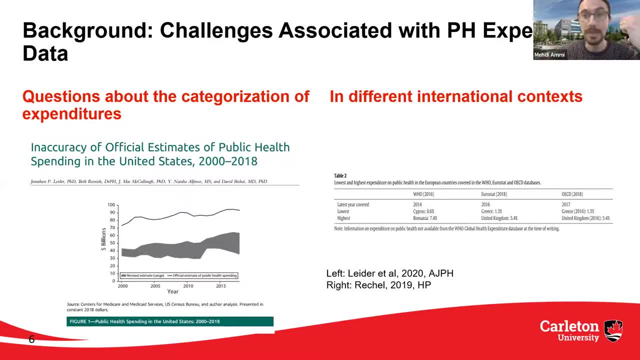 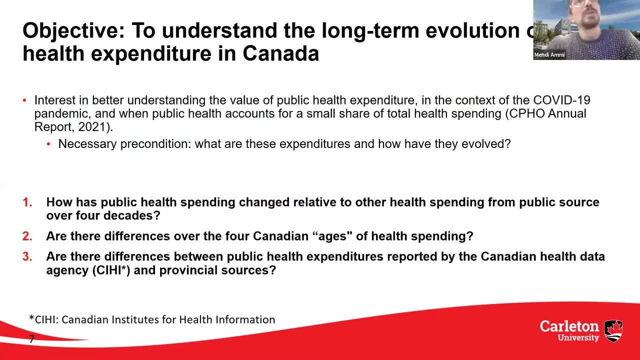 in the classification of what public health entails from an expenditure perspective. So, again, this is a first project in a broader research agenda. but in this project what we aim to do was understand the long-term evolution of public health expenditure. okay, Clearly there is a momentum, you know. 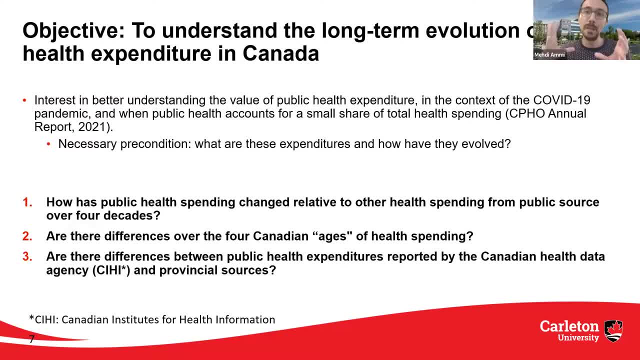 because of the COVID pandemic. just that we put a zoom in on public health and the importance of public health, And what the CPHO on our report was arguing is essentially like: this is this window of opportunity and we need to better understand the value. 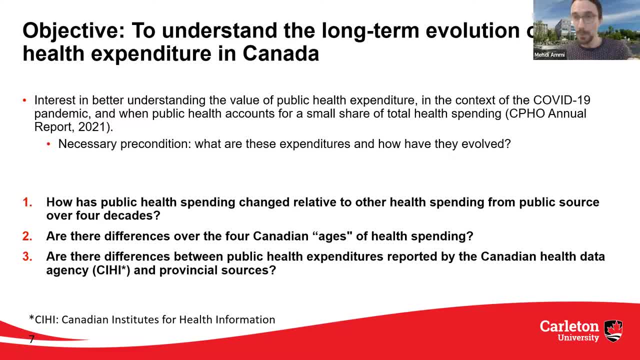 of public health expenditure just to argue for like more resources, in case there is a need for more resources, especially given public health accounts for a small share of the health spending in general. But the first stage there, the first step is really to say, well, what are these expenditure? 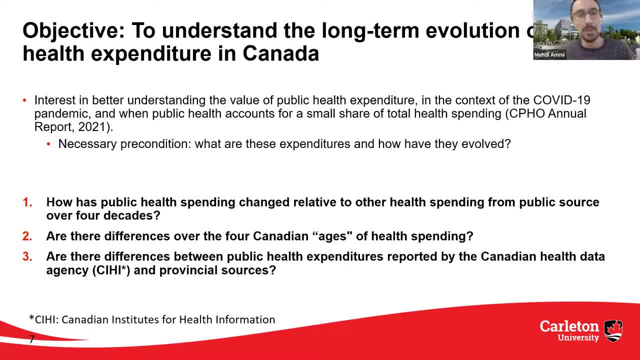 and how they are. and this is what we're doing in this paper, And we ask three questions, All as public health spending change relative to other health spending from public sources over four decades. So we look at physicians, drugs and hospitals- everywhere. 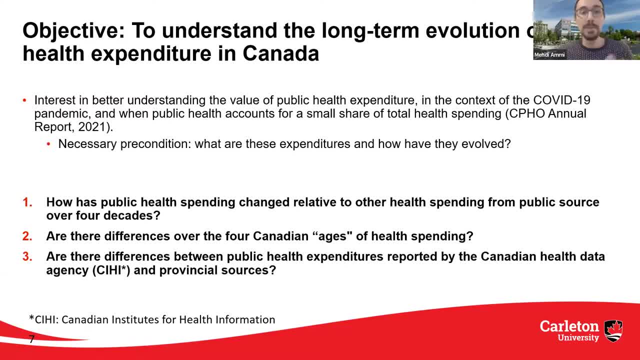 everything sorry from public source? Are there differences over the 14 in ages of health spending? So I'm going to explain more what I mean by that. And last, are there differences between public health expenditure reported by the Canadian Health Data Agency? 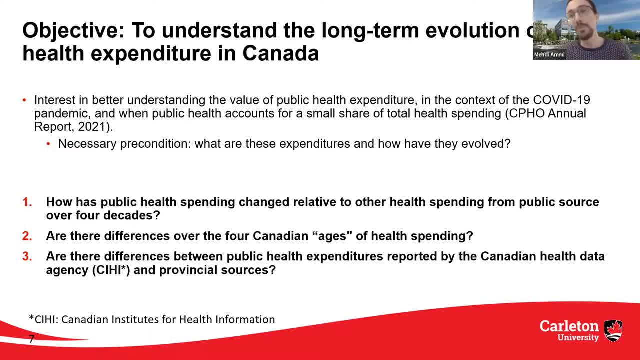 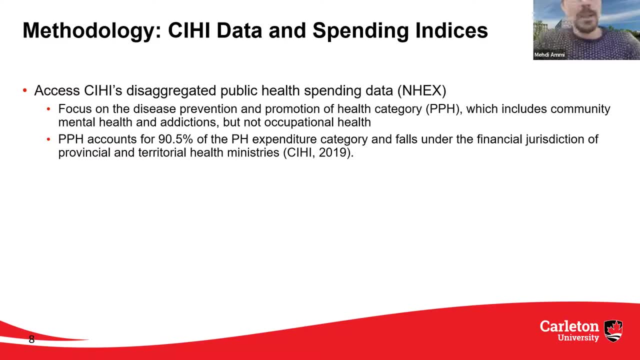 CHI-HI, the Canadian Institute for Health Information, and the provincial sources, Again keeping in mind this idea that in other jurisdiction this difficulty in classification have been raised. Yeah well, So a little bit of a methodology what we've been doing, you know. 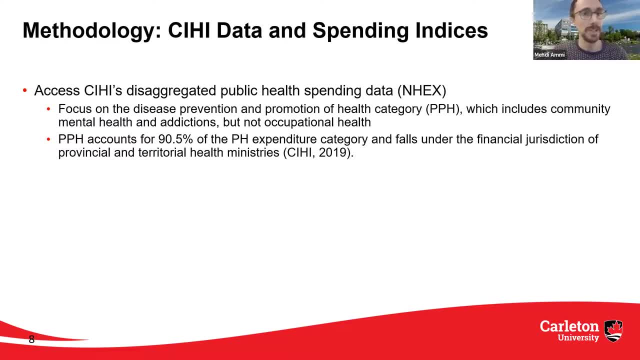 to try to answer these questions, you know, to the best of our capacity. The first is we accessed CHI-HI disaggregated public health spending data, So the NHX team essentially shared with us the data that they have that separates out what they call disease prevention and promotion of health. 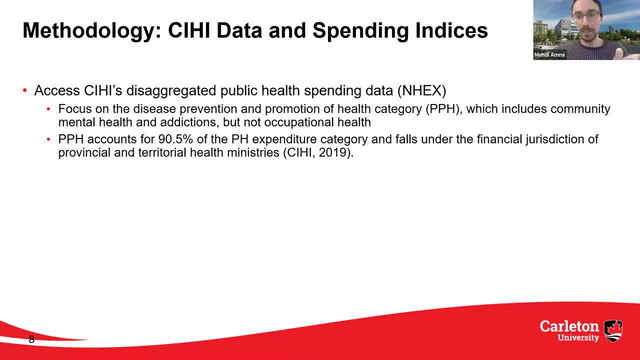 and occupational health. So the PPH category. there it includes community mental health and addiction, which is not something that is always done in international context, but we are, you know we are not going to do that. Obviously, there's very limited information. 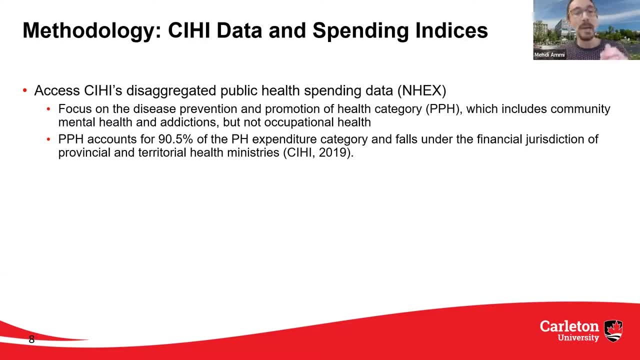 about the health of individuals and how they are going to deal with those discussions. And we're not able to tease all this out in the data, So they are not able to separate those Occupational health same thing. It is not always considered to be part. 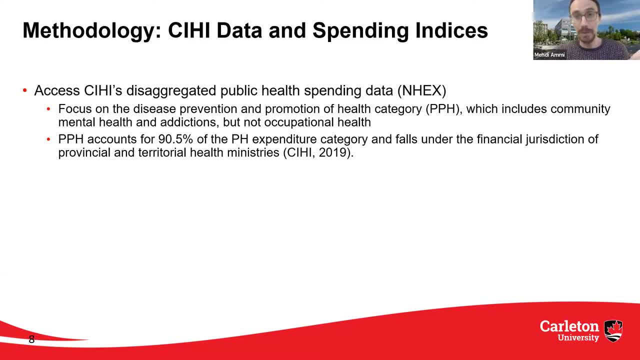 of the main public health functions, For example, if you look at the WHO classification of what public health entails. So we decided to be as conservative as possible and to take to focus only the PPH category. This PPH category is actually the large majority. 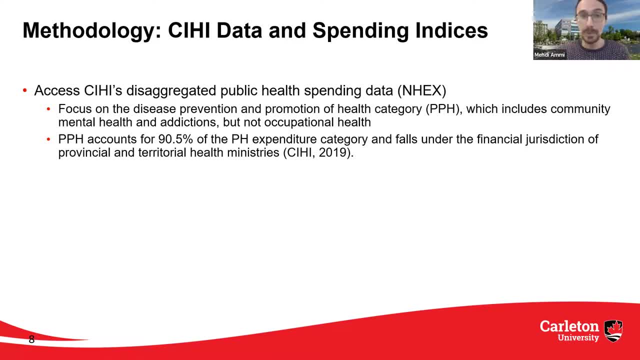 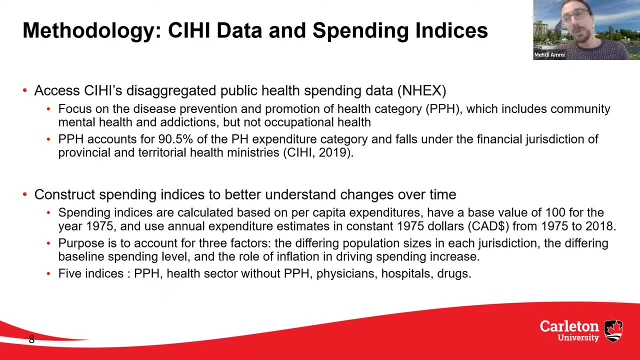 of public health spending in Canada, because it actually accounts for about 90% in 2018.. 90% of the public health spending- sorry, in 2018.. And it falls under the responsibility of provincial and territories. And then I've been trying to come up. 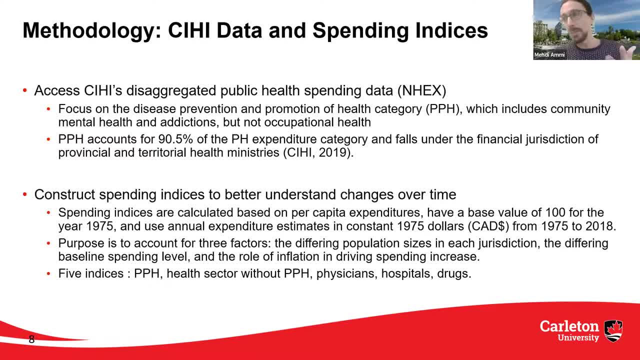 with a metric that is going to give us kind of an idea, a summarized idea, of how trends have been changing over a long period, Because that's what we want to do. We have, like about 40 years, 43 years of data. 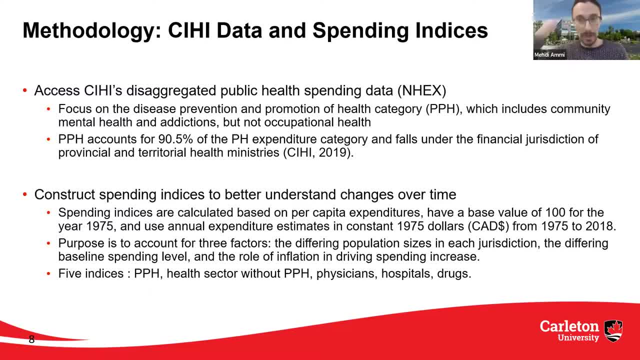 And we really want to have a sense. okay, look at this long period and not like short run evolution. So we just choose what is standard use in financial econometrics, just like indices, like analogous to something, but like the consumer price index, if you want. 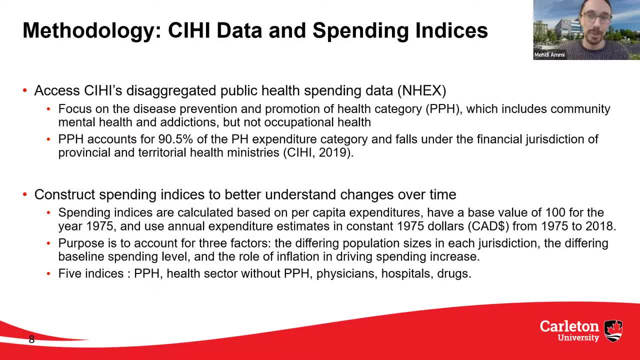 And the spending indices. we are calculated based on per capita expenditure. We have a value of 100 for the base year, which is 1975. In the general analysis, And we use annual expenditure estimating in constant $975.. And again, we cover the growth from 1975 to 2018.. 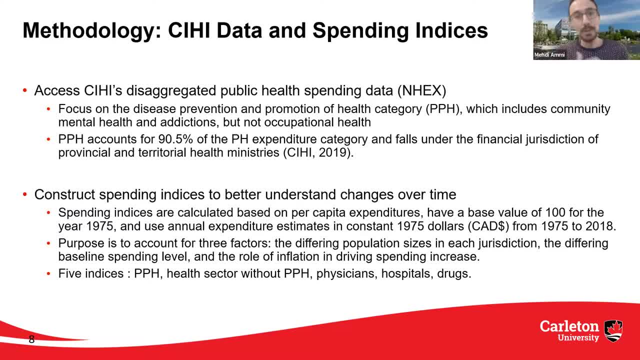 So that's 43 years. The purpose of the indices was just to account for three factors: the differing population size in each jurisdiction, the differing baseline spending level, because we don't focus on the trends- and the role of inflation, because we just want to be real growth. 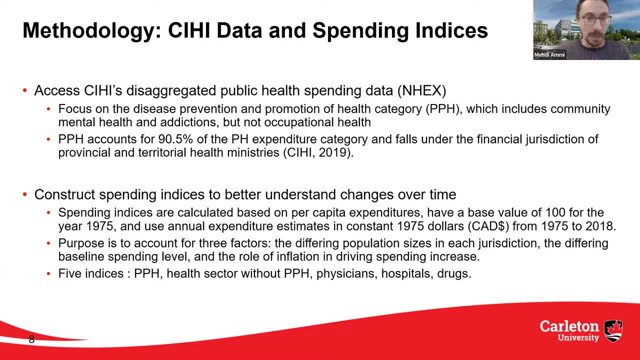 and not like nominal growth And we have five indices. We wanted to get a sense of how the public health sector grew compared to other main sector in the Canadian health system. but are paid from public purse. So physician and hospital, but also not whole drugs. 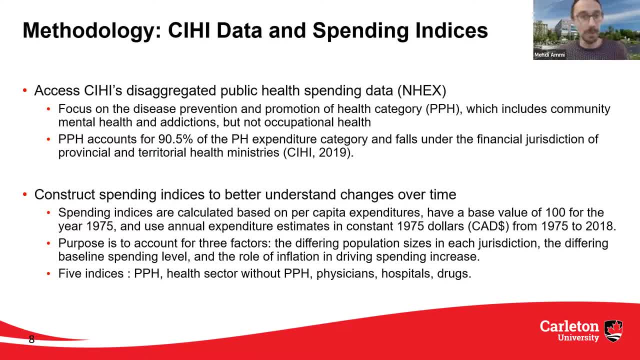 because drugs is also covered by insurance, private money or out of pocket. So just the drug portion that is paid by the public health, So the public purse. We took these three because they are the three main spendings. You know when you look at health. 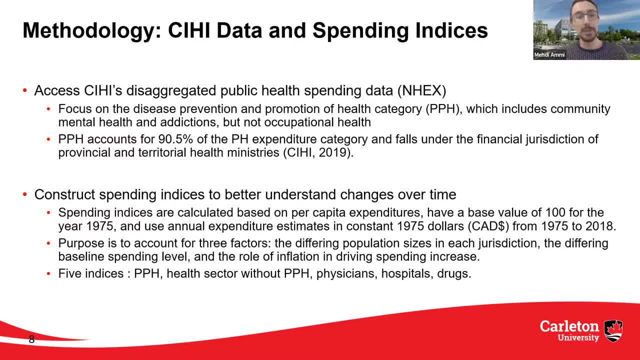 from public source in Canada and we also look at this health sector without PPH. we just say, well, let's look at everything that is not public health and see how it goes From the public purse. Again, everything is public funds. So this idea of, well, this idea of four ages, what So? it was again saying, okay, 43 years is good because we get this for public health Over to the other sectors. And the last part was this comparison of CHI data. with publicly available provincial government health ministry budgets between 2012 and 2018, because it was just like too many years to look at. Otherwise, 43 years is not something that is reasonably feasible. And there I want to really acknowledge, know that contribution of Robert Smith's. was just doing this work of data creation in the frame of another catalyst grants. So this is a good example of research beloved trying to be efficient with public research money. And now this work has been part of a publication of the NCC HPP with NCC HPP on the public health systems. in Canada. I really invite you to read those because you know public health systems are actually quite complex. They are really really helpful- these reports, And also Julie Fizel-Agnel and team for sharing the M3S data that they got from their CGPH publication. So we took this and then we just say, okay, we're going to estimate a kind of difference between the provincial estimate and CHI estimate. So the provincial important disclaimer: this is the budget. okay, This is not the expenditure. So this is what has been voted. 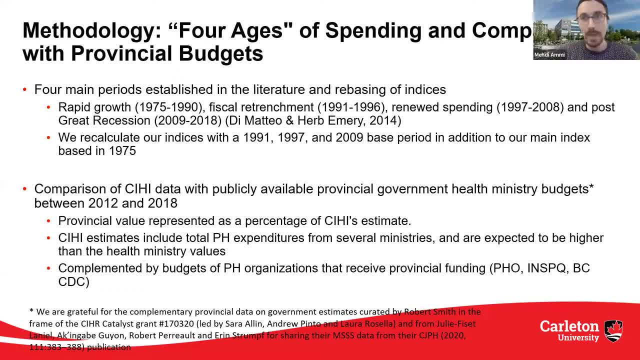 but this is not what has been spent. This is what has been spent, Which is an important nuance. So the provincial value is represented as a percentage of CHI estimate. The reason we do that is because we expected that CHI was going to be higher. 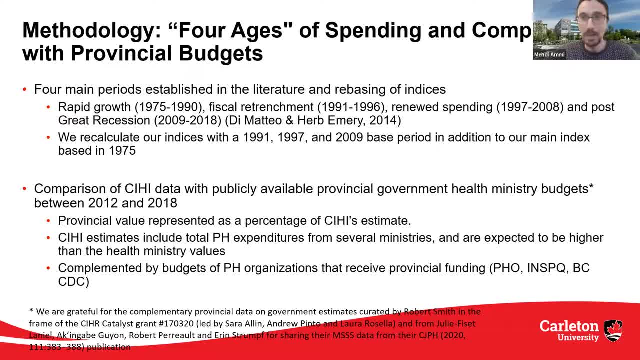 because CHI, when they just compile information but they receive the combined information they receive from different ministries, including the ministry of health, And we also tried to include, you know, some organization that that clear public health mandates that we're receiving from provincial funding. 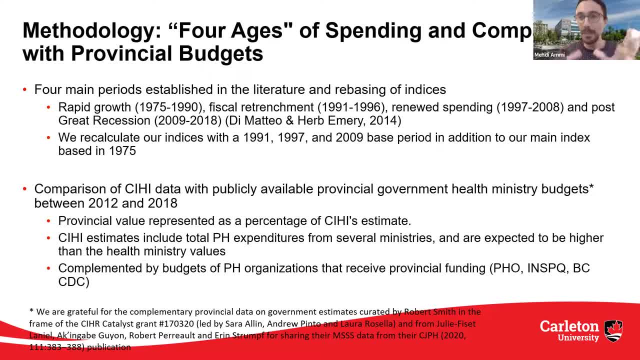 And that are going to be captured by CHI but not going to directly appear in the health budgets from the ministries. So this includes public health Ontario, ENSBQ in Quebec and BCCDC in British Columbia. Okay, Another view of the findings. 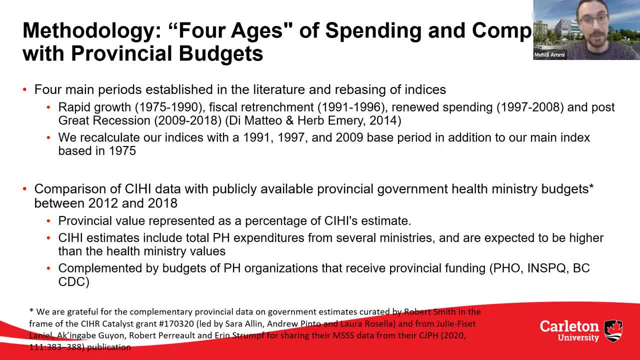 We're not going to go over the results of the paper Again. I reiterate: there's a little bit of infotainment there, but I reiterate that the paper is upon access, So I encourage you just to go and read it. 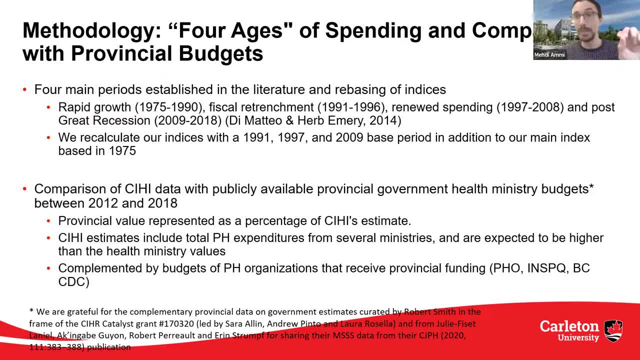 But what I think are three key findings from the paper. The first key finding is that there is, overall, a substantial growth in long-term public health spending in Canada, And that came a bit of a surprise for us because we were really not expecting that when 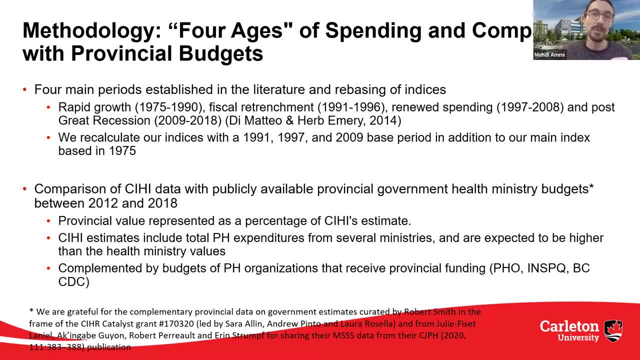 we were starting the analysis. That's over 43 years, 1975 to 2008.. I didn't put everything on the slide there because there are like the 10 jurisdictions, 10 provinces, plus we have two territories We had to put together: Northwest Territory and Nunavut. 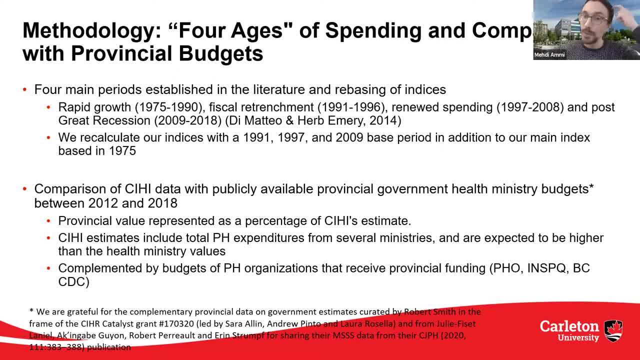 because before 1999, there were like one entity plus the federal direct. So that would be way too much for one slide. But I wanted to highlight the most populous province and the Nova Scotia, because it's also a bit different from the rest. 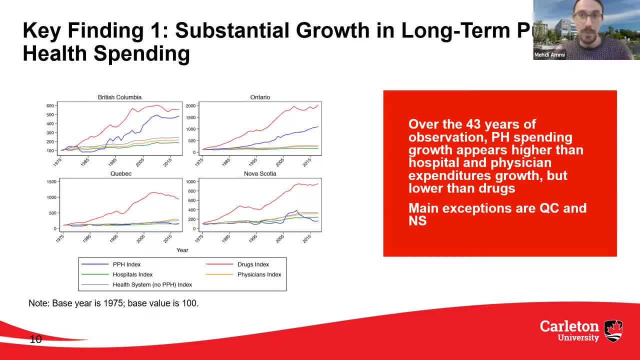 What you see on the slide there. I think what I want to highlight is the blue line. The blue line there is our PPH index, So you interpret this as a measure of growth over the 43 years. that adjust for inflation, that adjust for different population size. 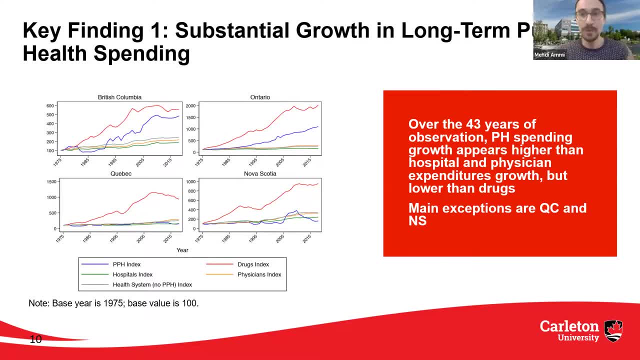 and that adjust from difference in the start year 1975, across BC, Ontario, Quebec, et cetera, et cetera. But what is particularly striking when you look at BC or Ontario is that you see, so the scales are not. 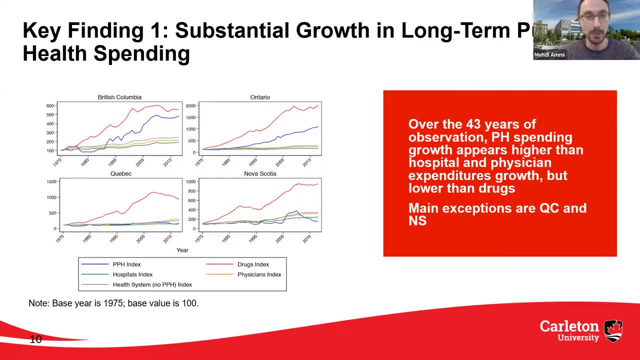 exactly the same on each graph, just mind that. What is particularly striking is that the growth in public health is really higher than if you look at orange, the growth in physician spending, In green, the growth in hospital spending And the gray there is like. 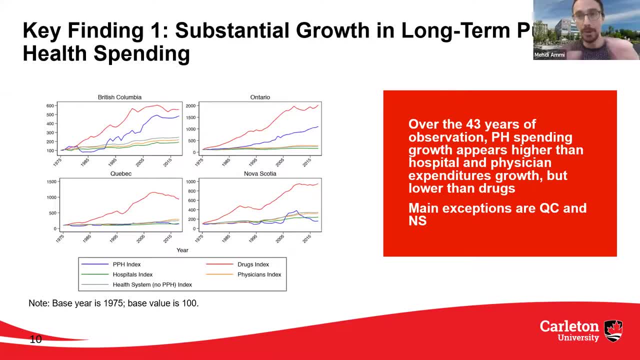 Every other public spending. that is not public health when you look at Ontario and at BC. But it's below the growth of drug spending. So drug has been really the area where spending growth has been the largest, far and large. But PPH is- I mean public health- is really just behind. 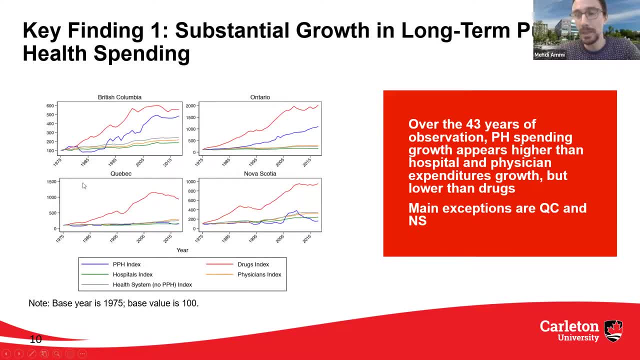 And that's what we see in most jurisdictions except this two guys there, so Quebec and Nova Scotia. If you look at Quebec, so it's a bit hard to see because it's just like in the part there, But if you look at Quebec you can see that the PPH index is. 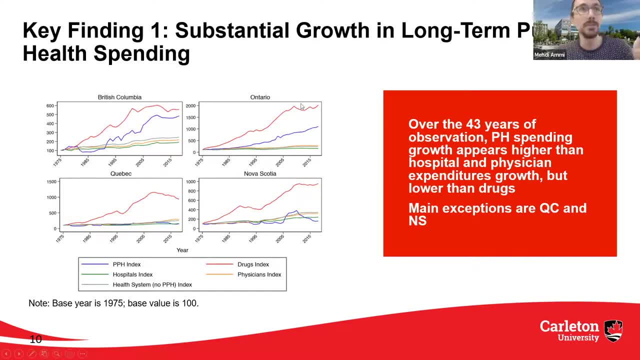 really flat and not higher than hospitals. I mean about the level of hospitals, not higher than physician, not higher than the health sector, Almost- I will show you a number after, but almost like nothing really changed over this period. And Nova Scotia, well, you see, it has been really flat up. 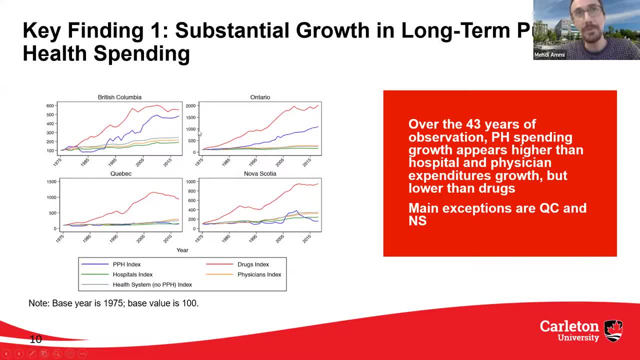 to 2005,. and then it's increased, But 2010 back and it's almost like it went not exactly to the initial level, but really low. So the story really there is: we see a substantial growth pretty much across the board, higher than other health sectors. 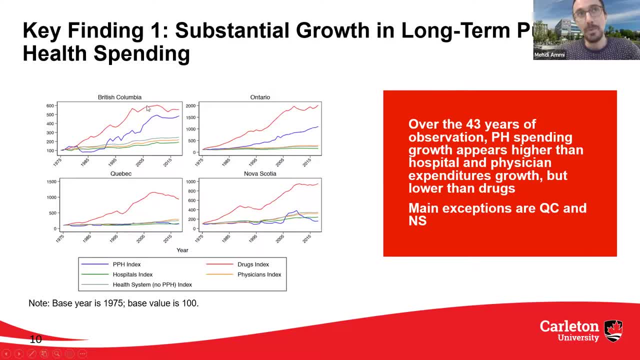 except drugs, but not everywhere. Quebec and Nova Scotia seems to be some of the main exceptions. So then, But That was over 43 years, but a lot can happen in 43 years. But that tells us something about how Canada can be the top spender. 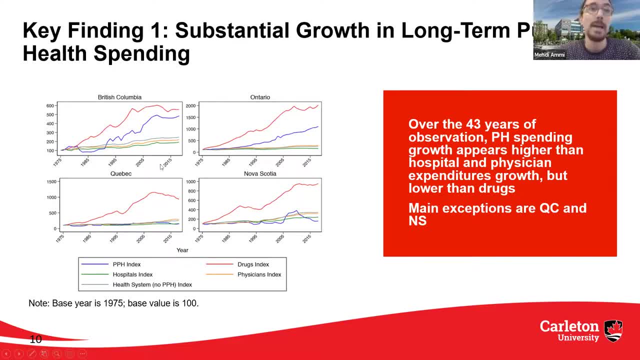 I mean allocating the highest share of its health spending to our public health. Now we look at the last age. I cannot put a table with a four against in the paper. Please feel free to look at it. But looking at the last birth post recession, 2009 to 2008.. 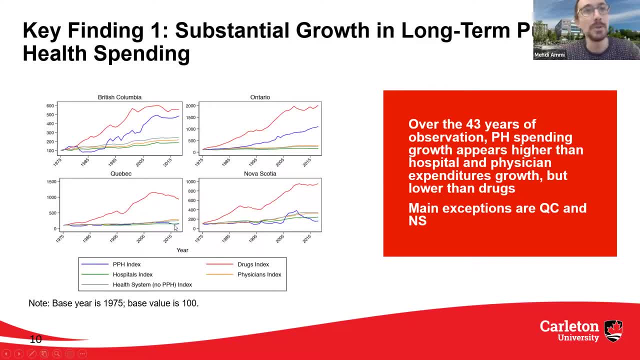 And what I've been doing on this slide is just like trying to make it as visual as possible. In green is when you see that the PPH index is about 10 points higher than the health sector index, so no public health. And in red is when it's 10% below. 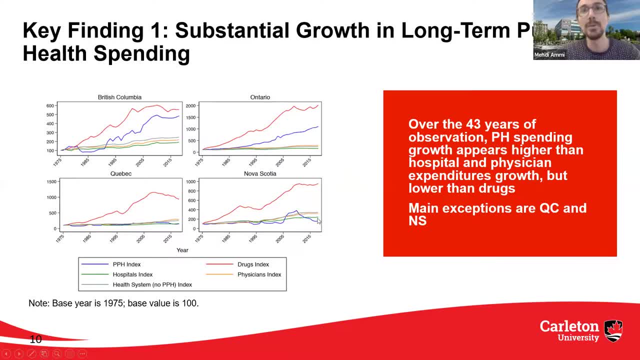 I mean 10 percentage point below. It's just, it's arbitrary. with 10 points, OK, I can take anything, but that's just really help. just see part of the story. Well, you see it. No, there is quite a. 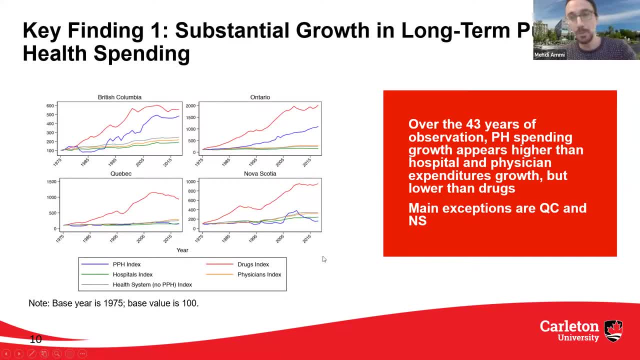 Some greens here, So that means that there are still some places like Ontario where there is an allocation. The growth in public health spending is higher than the growth in other sector. You can see places like Alberta or PR where it's roughly the same growth. 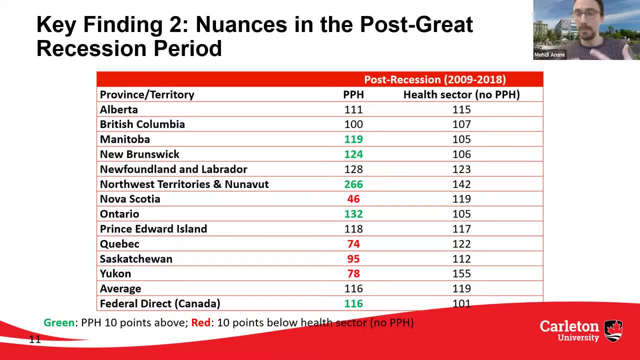 So public health is not really different than the health sector and type of growth. And then you see places where it's just lower and there is actually a retrenchment in public health spending. So that's what you see in red, which below 100. 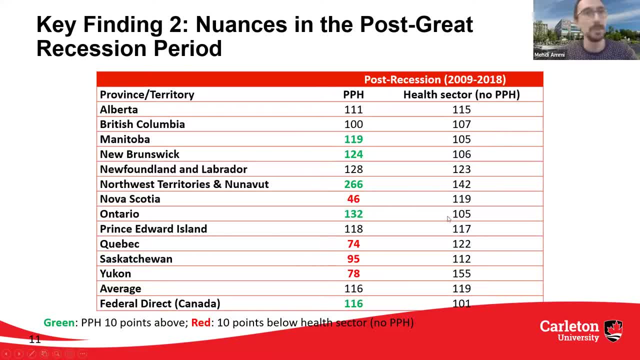 That means that the public health expenditure in the real term has gone down, And you can see this in Saskatchewan, but it's even clearer when you look at Quebec and Nova Scotia. So Nova Scotia: what it says is essentially between 2009 and 2018, it has been cut in half. 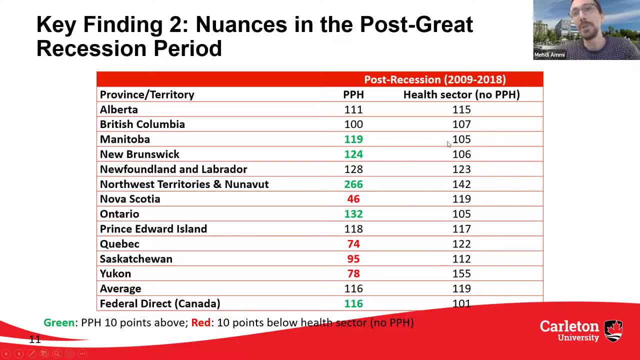 in the real term, the public health expenditure, While the rest of the health sector continue to grow, and same story in Quebec. So that's this part of OK. We need some nuance. Overall, it seems like there is a lot of growth. 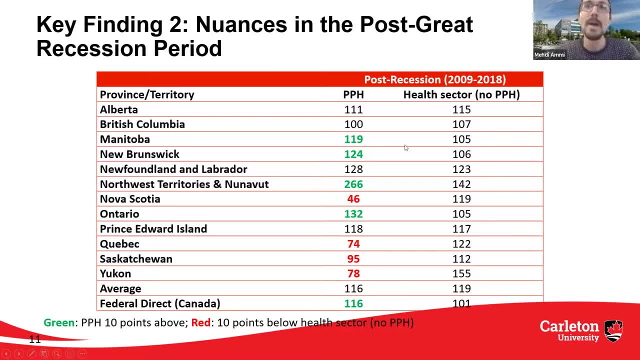 except Quebec and Ontario. But while you see, Quebec and Ontario are still there. Saskatchewan, Yukon might also see this decrease from 2009 and onward, But the rest, not a lot of difference between the health sector and public health in terms of growth. 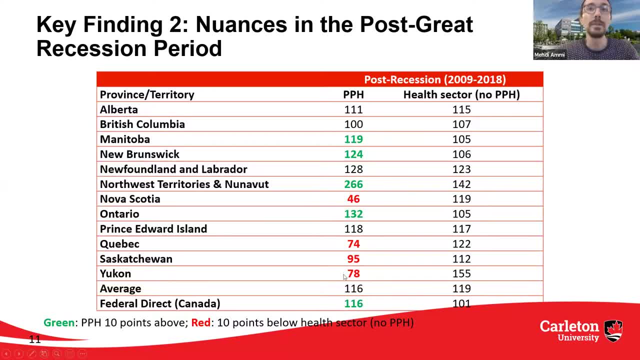 And the last one. this is one that is like, oh, inviting me reflection, this idea of OK recall. we just took CHI, We just said OK in the year, let's look at how much is spent in public health. 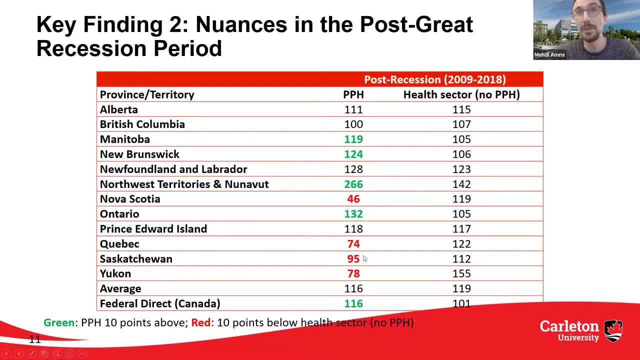 as stated by the province, And we just did the ratio. So the percentage there just tells you that there is a lot of differences between the province and CHI. So the closest is Nova Scotia, where it's about 80%, And then you have a larger difference, just like BC. 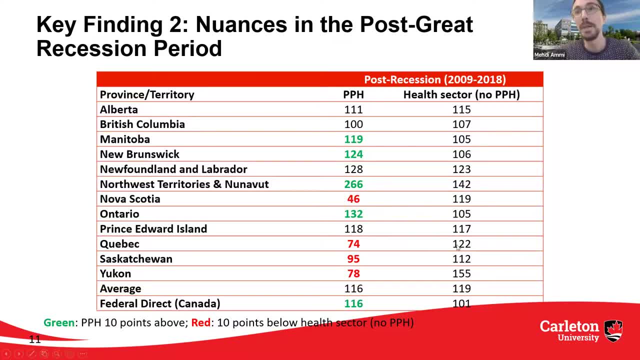 it's about 40%. Ontario, it's about 30%. Quebec, it's about 45-ish. So that's something that says that there is a difference in classification. However, the difference is relatively time-invariant. What I want to make clear is that you need to understand. 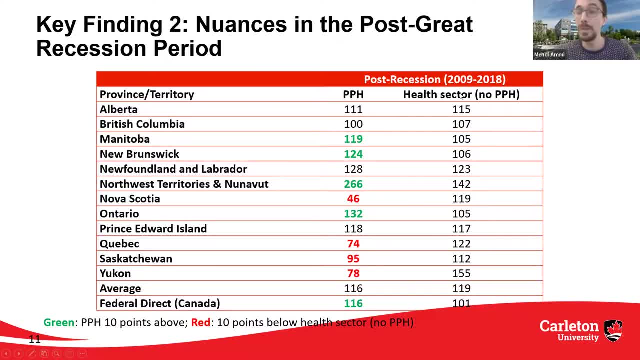 it's not like CHI has a specific data set and they do their stuff on their own, and province have, like this, other data set and they do their stuff on their own. The province communicate their data to CHI, their expenditure data to CHI, and CHI does the classification. 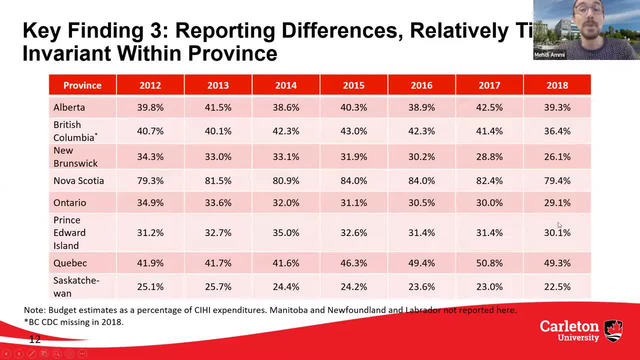 So this is essentially the same data but that is classified differently. But I guess the difference is important to keep in mind. But the kind of silver lining is that, at least for the period that we looked at, seems to be relatively stable over time the difference. 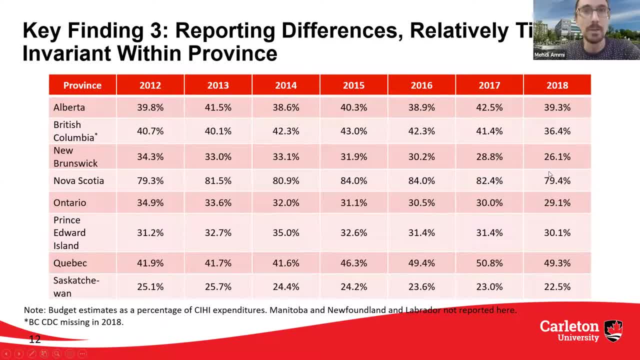 So now can we reconcile these findings? The first thing is what we find is, looking at the very long time period, we have a strong growth of public health expenditure in Canada, while what we tend to hear is that the public health system is not receiving enough funds. 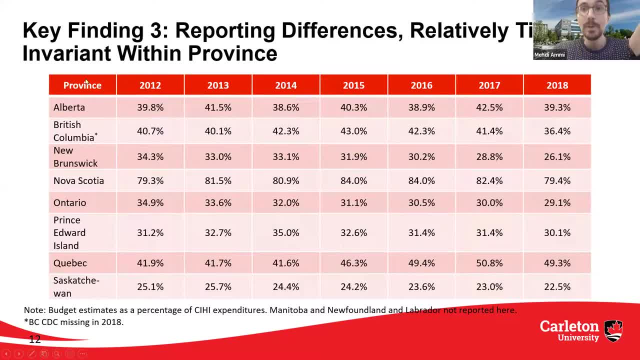 And I'm just mentioning that. I'm just mentioning that. I'm just mentioning that I'm just mentioning these two papers because they have been important in this very recent and very important in this field. The first is by Fisalania and colleagues on Quebec. 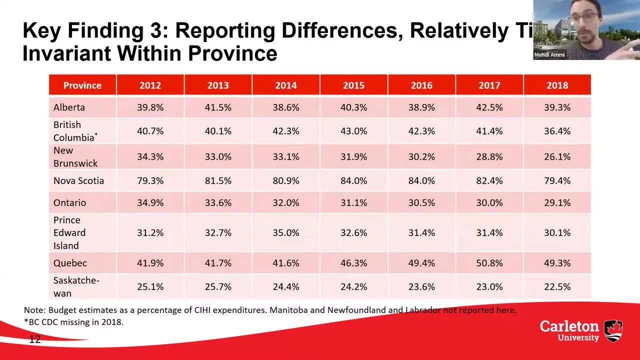 And the second is from sorry by Caldwell and colleagues and on Nova Scotia Sorry, And they are both published in the Canadian Journal of Public Health. What Fisalania and colleagues found is, in a nutshell, a reduction of public health expenditure. 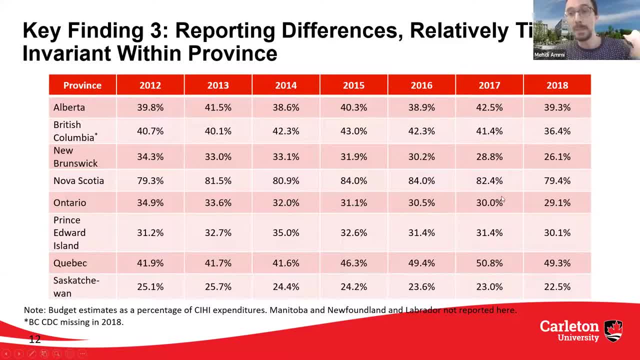 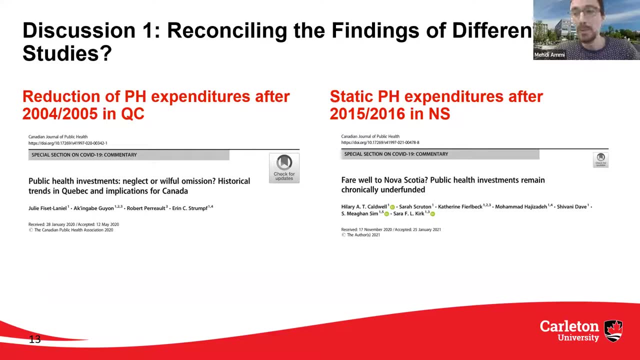 after 2004 and 2005 in Quebec And Caldwell. what they found is that the public health expenditure have been static after 2015 and 2016 in Nova Scotia, So they are just telling us: well, something is not good. 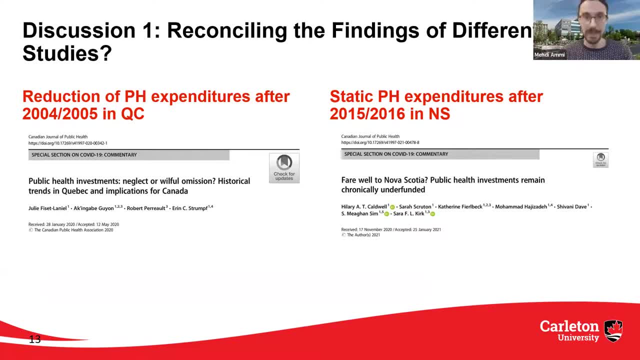 They maybe have slowed down. They are decreasing the growth of the public health spending in these provinces. That's also what we find. This is consistent with our finding. Our finding were really showing that Quebec and Nova Scotia, to a lesser extent, Northwest Territory and Nunavut. 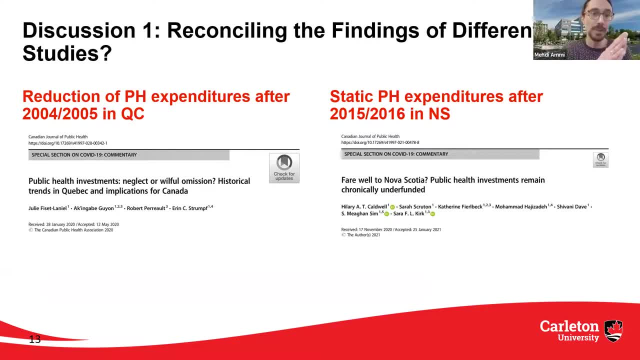 were really standing apart. So they may be saying that, OK, we are, and they are using the provincial data to be clear. I forgot to say that They are using the provincial data, not the national CAI. They are using the provincial data to be clear. 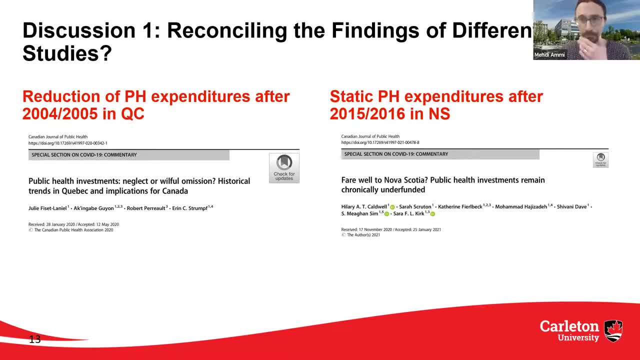 So there is some consistency, Even though. so the story about public health system growth- I mean public health expenditure growth- declining or being stable is. we see that in Quebec and Nova Scotia as well, But we don't see that in other jurisdictions. 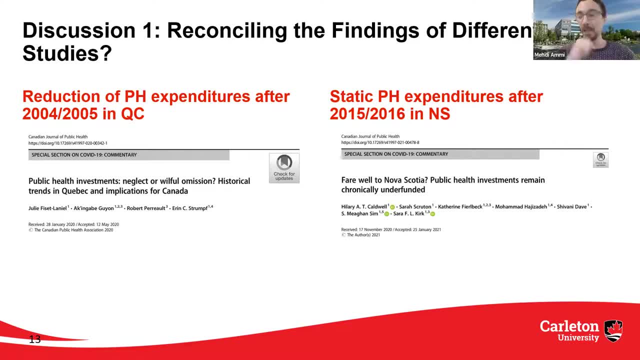 This question of classification. OK, that's a very central one. What, What, What do we mean when we say public health expenditure And this is not? this may seem an easy question, but it's not at all an easy question. 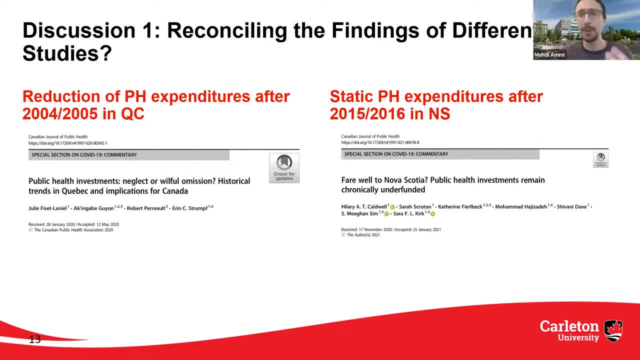 And what I'm trying to show you there is that there are different standards on how you can classify expenditure as being public health, as being something else. The left column is CAI, So the two categories are already mentioned And remember our focus was on the three. 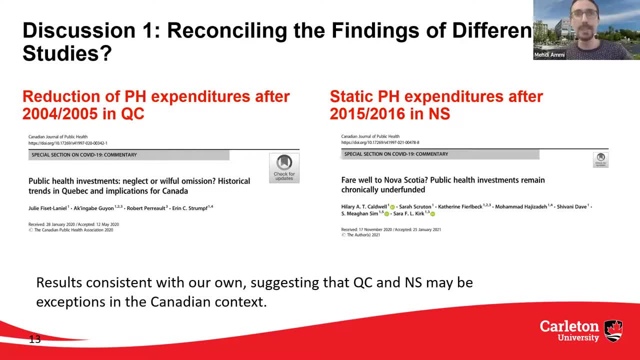 On the first- this one- I don't know if you can see the cursor there- Then you normally have an international standard, the system of health account which is there to help make comparable across OECD countries the health expenditure. Then you see there are like six categories. 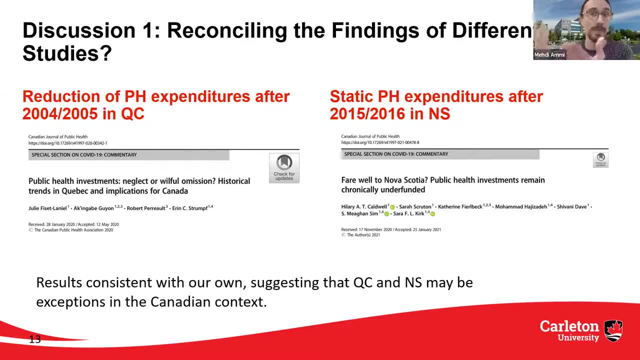 but they are relatively aligned- not fully aligned, but relatively aligned with the public health functions. If you look at Australia, they go down to 12 different categories of what is public health And if you look at the UK they have like five categories. 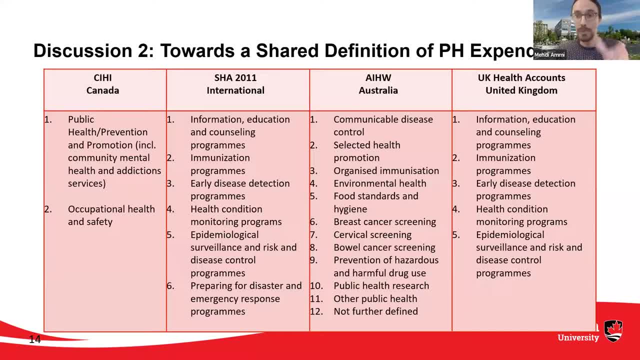 And this one is really like they separate, for example, disease detection and immunization, which is part of prevention, And they have information, education, counseling, which can be seen as also somewhere between promotion and primary prevention. But no, that's. 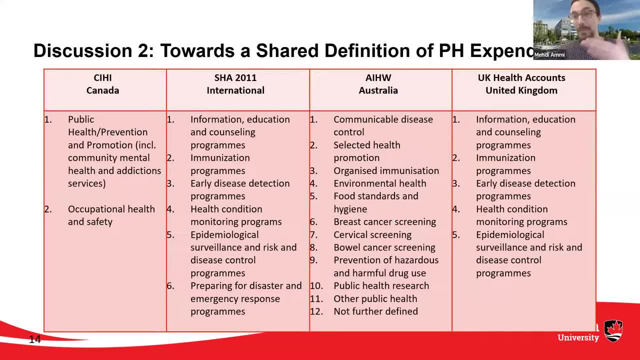 If you have a different framework to classify, you are likely to end up with different results. That's what I'm trying to communicate, And it's not something that is only happening in Canada. So what we need is to be able to get towards a shared definition. 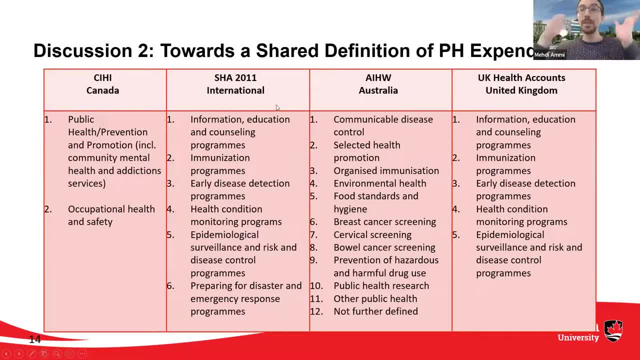 of what public health expenditure is, but doing so in a way that can be classified from the data that is currently available, at least if you want to have a sense of the trends. So well, what can we do with the public health expenditure? 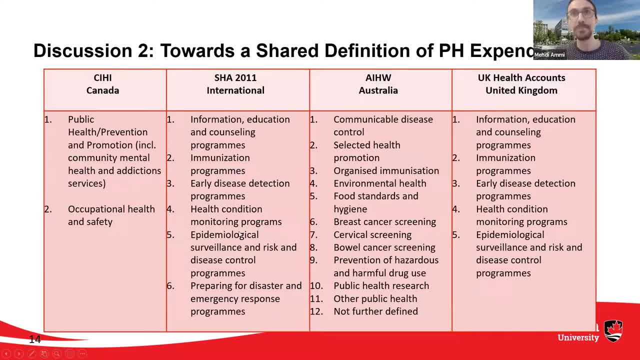 data currently available. What I think is important is that we don't end up, and especially out of this webinar, and think, well, you know what This data? we can't do anything with it. I don't think it's true. 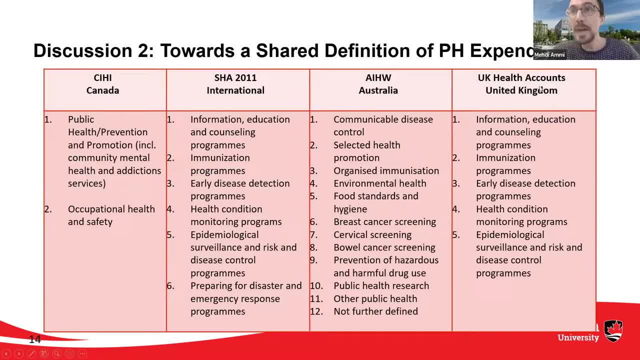 Again, I'm trying to highlight that this is not a Canadian-specific question. This is like a question that applies broadly to public health expenditure. And well, it's a free translation of this quote from Voltaire: It always looks good to have an Enlightenment philosopher. 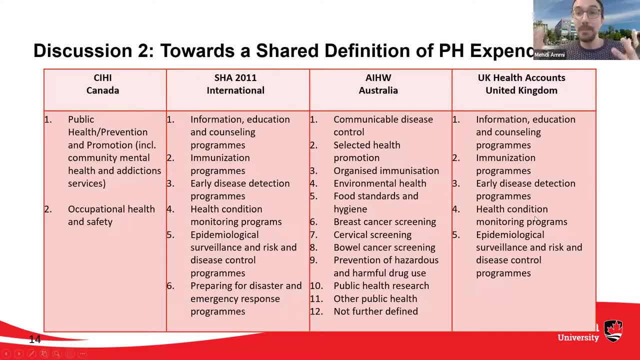 The best is the enemy of the good. We just have to say, well, OK, what can we do with the information we have now, which does not prevent from trying to get to this shared understanding of public health expenditures, As I mentioned, as I've been trying, 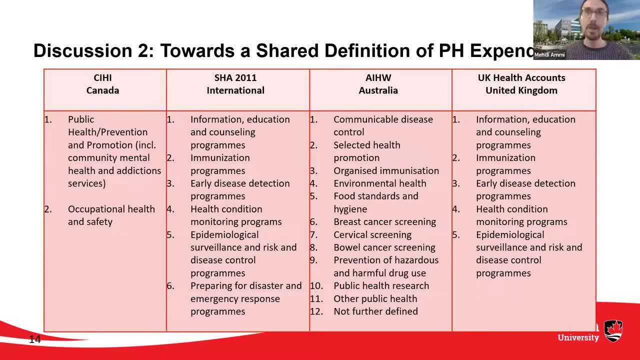 to reiterate this challenge of public health expenditure data is not unique to Canada and it lies in the categorization and definition of public health. First, there are some variations in how public health is defined. If you look at the definition from FAC, 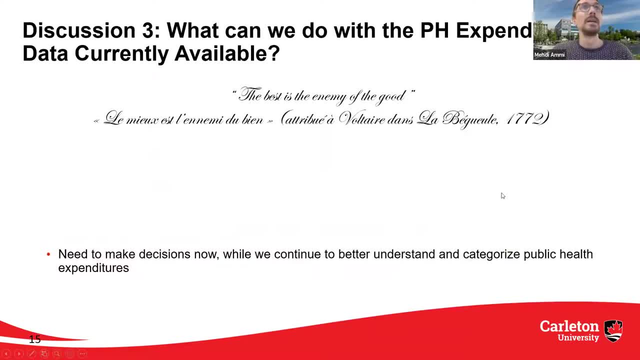 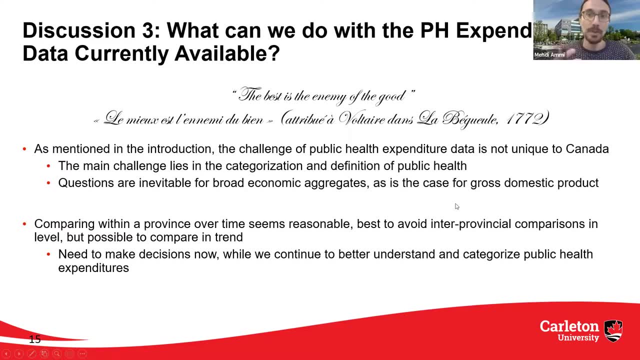 and the definition from BC CDC. it's not going to be exactly the same and not exactly the same as the definition of the WHO. And then when you look at inside the expenditure, you are going to see this classification. that was like two slides ago. 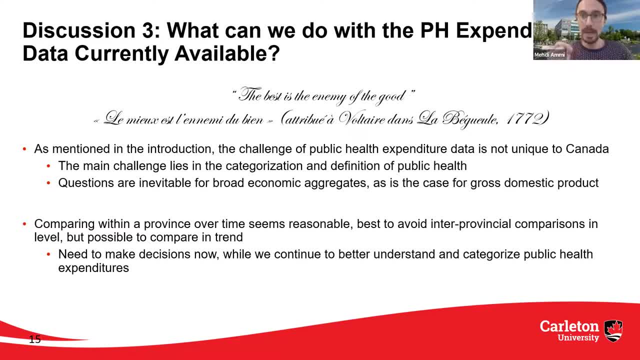 Questions are inevitable when you look at broad economic aggregates. This is the case from the GDP. That's going to happen. They're always going to have question marks and it's not like one party is correct and the other is incorrect, just like it's a latent variable. 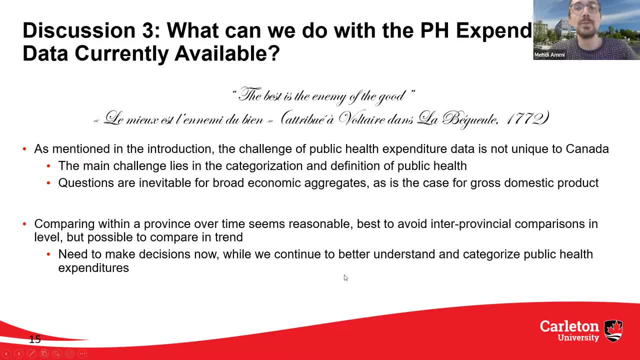 We don't know it for sure. We just try to approximate it From the data, from what we found in this little exercise of comparison, comparing within province, We found that province over time seems reasonable because this measurement error, or call it this way, 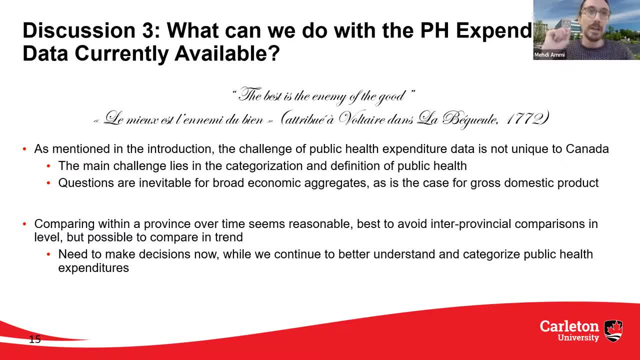 is relatively time invariant, But it seems preferable to avoid interprofessional comparison in level. OK say, this province is spending bad, this province is spending bad. compare the two. Well, maybe we're not talking exactly about the same thing, But in trend if they are relatively stable over time. 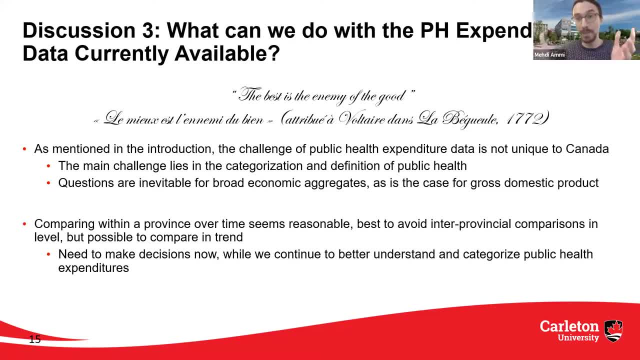 in each province. when you look at the trend, it's going to be something that is relatively comparable, And you can also compare in a province between public health and non-public health, Because we need to make decision now. OK, I come back to this question of a CPHO report. 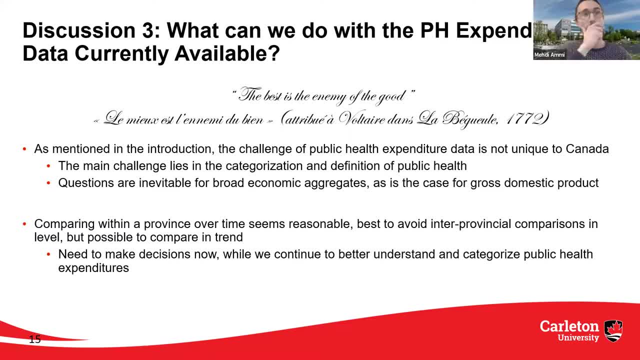 and that just says well, there is a window of opportunity And to make the case for public health, we just need to use the data and the information we have now and continue to work on. perhaps, in two or three years, get something that is more consistent. 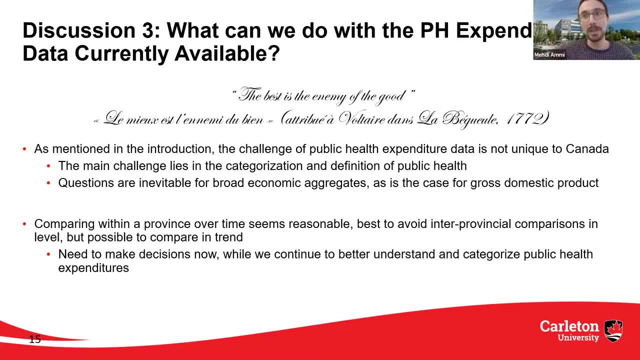 across different classifications. OK, So this is again a research agenda that is ongoing. This paper is done, but there are other papers ongoing. What we are looking at right now is in a paper with Emmanuelle, Sarah again and Antoine. 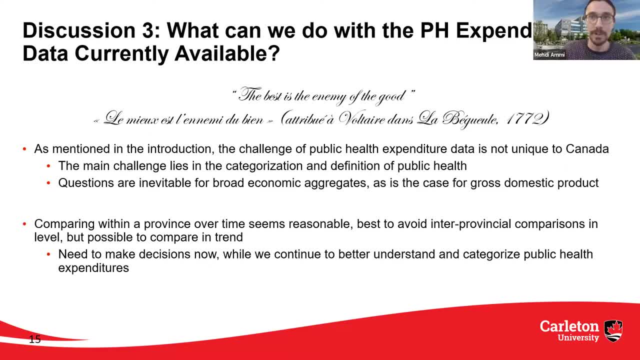 Dewan, who was just looking at the effect and the long-run relationship of public health adventure and health in Canada, And this is still a work in progress. We are also looking with Olivier, Jacques, Alan, Noel and also again Emmanuelle. 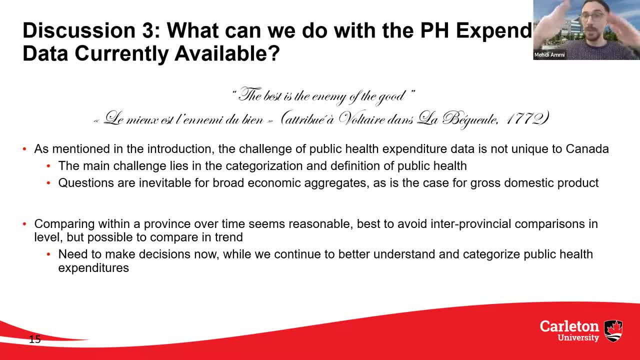 at the political and fiscal determinants of public health spending in Canada. We are going to get a draft soon, And this is going to be presented at a conference, And so that's what we are already doing And what we have started to do with another CIHR grant. 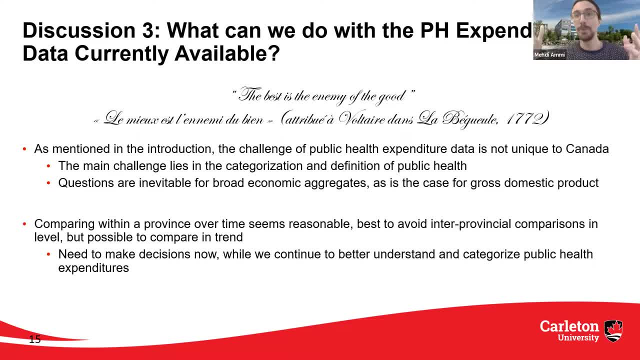 the number is there. Thank you, CIHR. Just to try to better understand what public health expenditure right, Right, Right, Right, Right Actually, and how they compare across contexts. So what is just classified as public health and whether something? what is public health in one country? 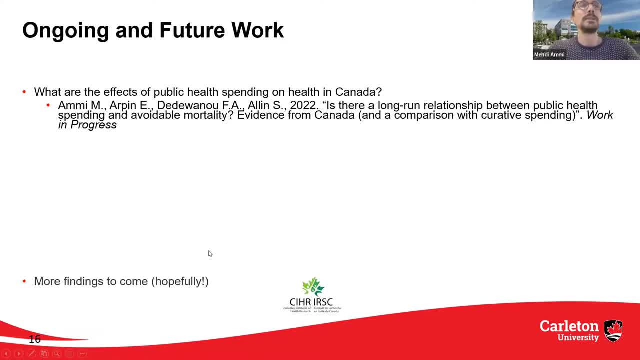 is not public health in another. So we just are looking at trying to do this mapping of the different items that enter in public health in different provinces, in different Australian states and in different English cities And we just try to see if there is an alignment. 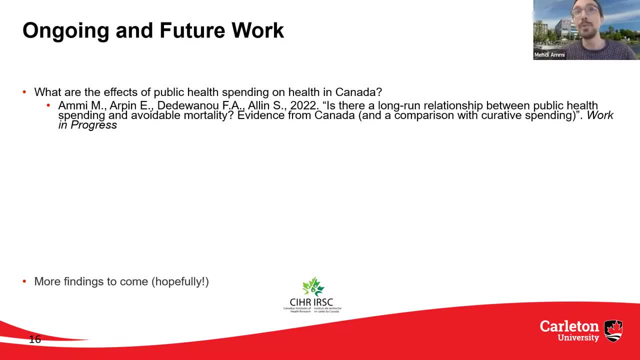 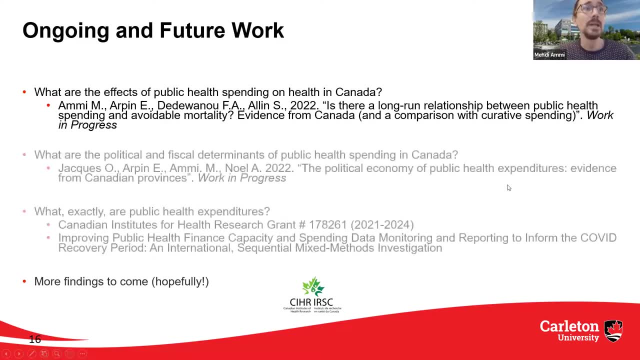 But the first stage, And after that we hope to see: well, can we just build a new data set that is just going to provide some consistency across these different jurisdictions? That's something that we have started a few months ago. Still work to come. 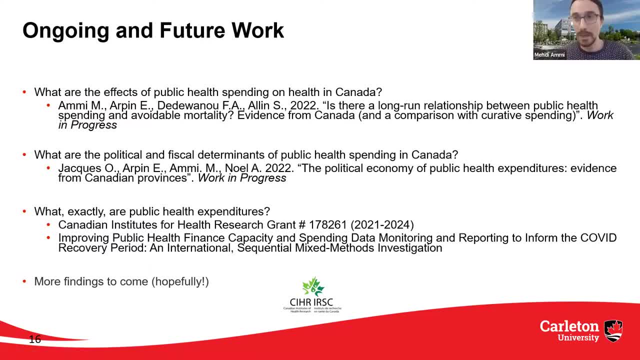 But we hope really just to contribute to this better understanding of public health systems in particular looking at the expenditure and financing side broadly, And to contribute to really understanding the determinants and strengths and effects of public health. So that's, hopefully it's exhaustive from the talk. 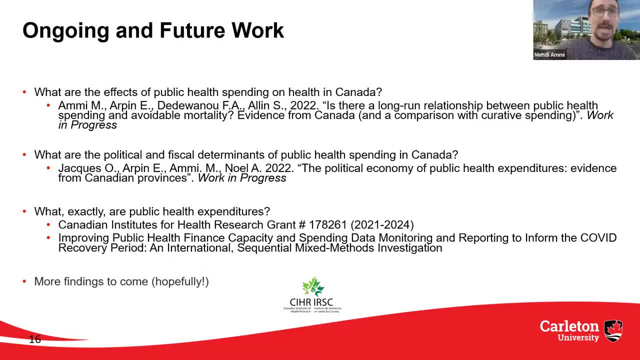 And I'm just going to stop there because my alarm is going to ring. Just stop it before it rings And welcome comments and questions. Thank you, Thank you, Mehdi. Thank you very much. All this information that you have presented make us very cautious when we talk about public health. 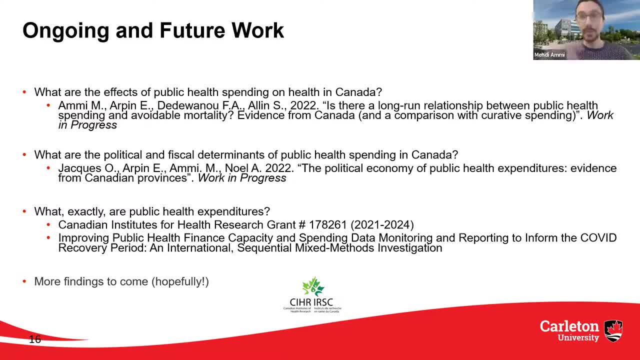 expenditure And it was really interesting. Tomorrow. I just want to let you know that we will send you Dr Zahmi's slide deck to all the participants. So we will send the slide deck Of Dr Zahmi to all the participants tomorrow. 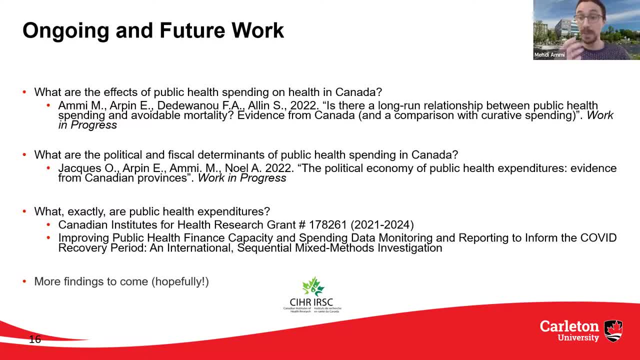 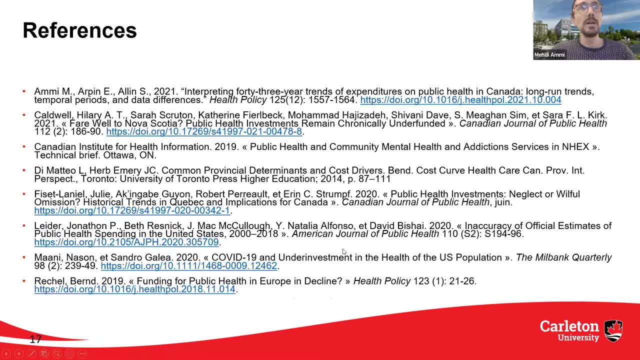 So don't worry, if you don't receive it today, We will do that tomorrow Without any further ado. I will give the floor to Mehdi to answer your questions that you sent to the Q&A box And we will go to Natalia for this question from participant. 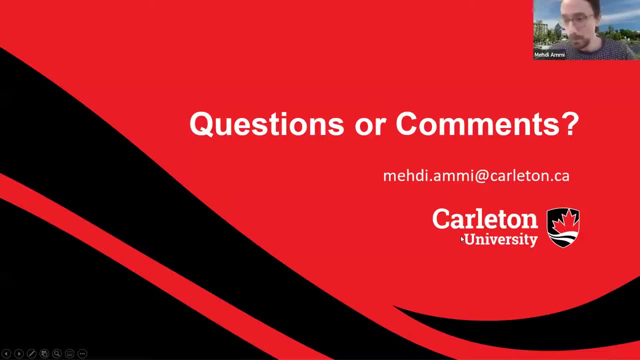 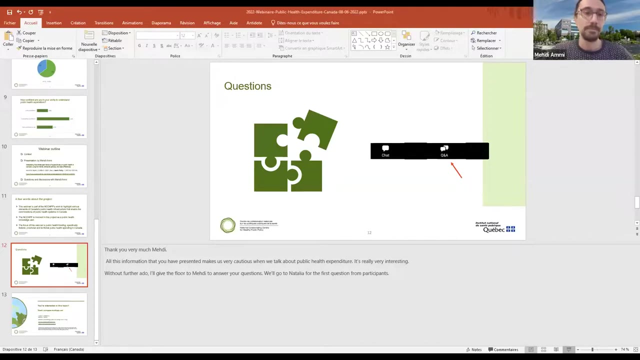 Natalia. Thank you, Caroline, And yes, We have quite a few questions, So I'm going to start The first one. our participant wants to have some clarification about the numbers used in the presentation, So he's asking in terms of public health expenditures. 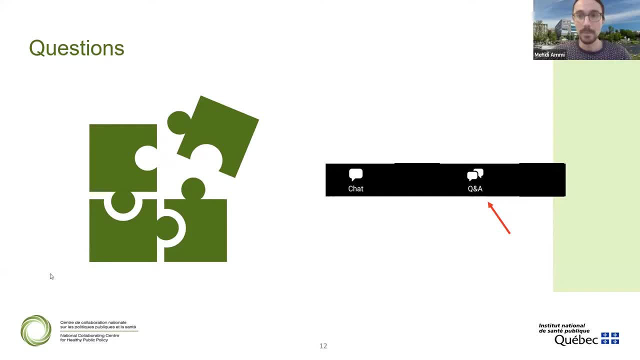 is an aggregate of all expenditures, from all orders of government or only from one public administration, For example, in the case of Canada, the federal government. In other words, in the case of Canada, do public health expenditures include those made by municipal public health units? 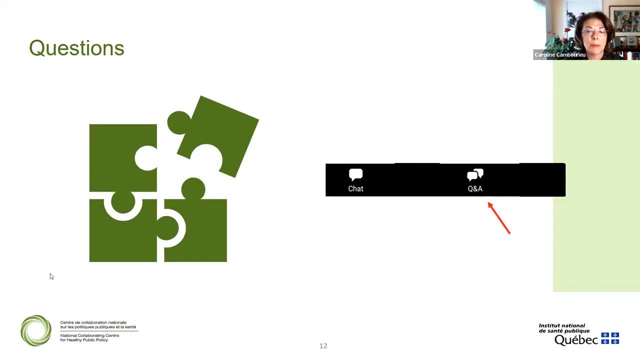 OK, So what we are seeing is the money that comes from the provincial government, But this money is including the transfer from the federation, And this is also including the money that the province is transferring to the municipality. So that's this kind of mixed bag. 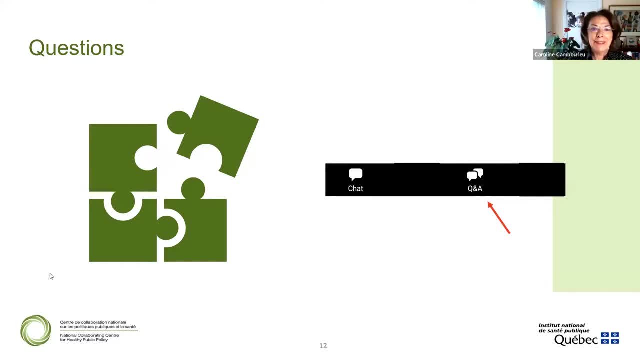 That falls under the responsibility of the province, But that's not directly. It doesn't need to be necessarily something that has been collected from taxation by the province. So this is yeah. So I think I see where we are going. We don't have, for example, the municipal spending. that is just. 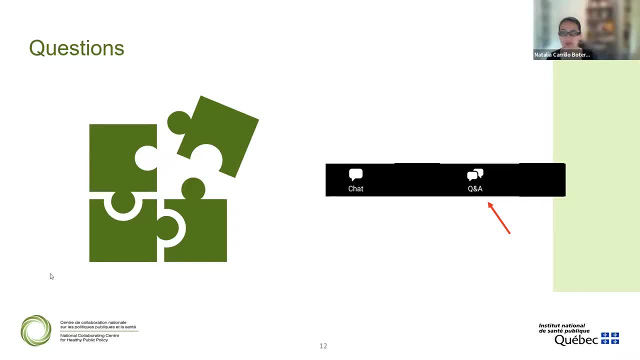 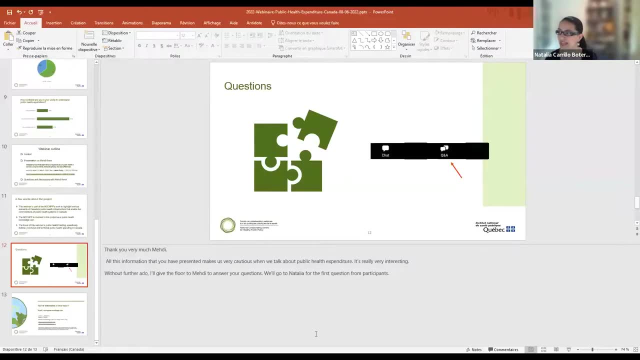 coming from municipal tax. It's not captured there. And one of the other thing that I didn't show you, but that is in the paper. we also look at the federal direct. So I mean there are special programs, OK For institutionalized population. 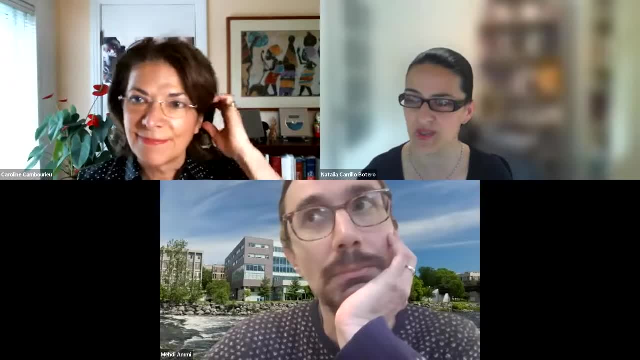 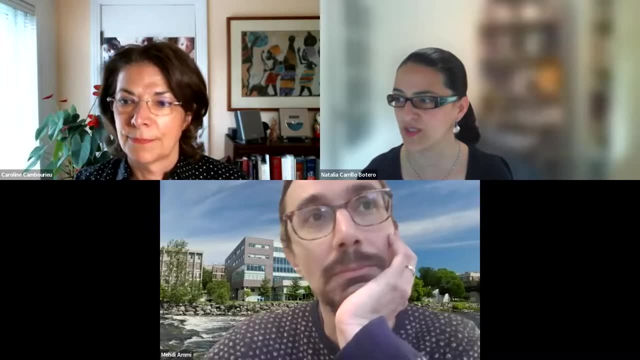 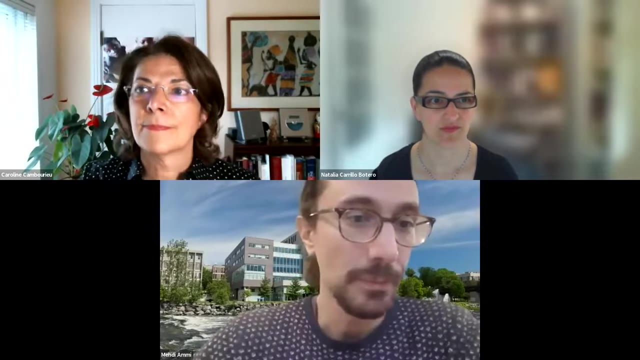 indigenous population, et cetera. But there it's looking at the provincial level. Thank you, Natalia. do you have another question? Yes, I do. I'm going to go in order first. So how do these findings in Nova Scotia and Quebec 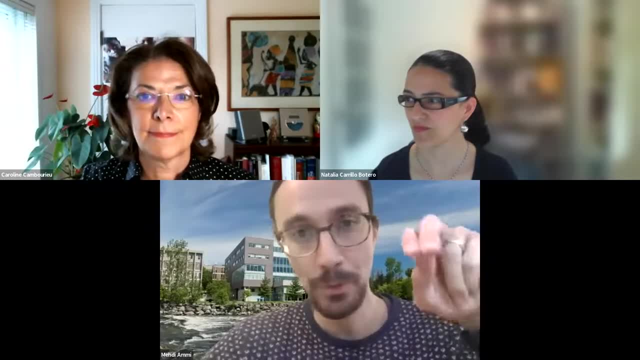 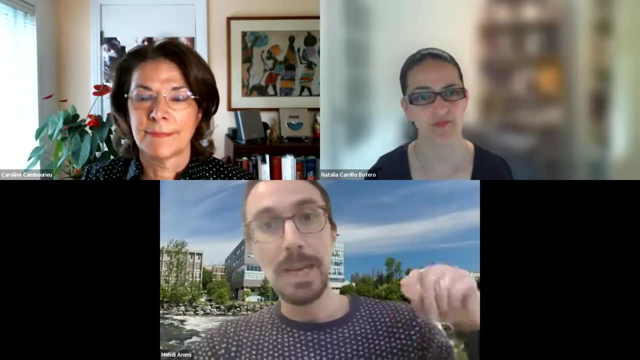 align with population health outcomes. Well, we don't look at the outcomes. Just to be clear. this is another paper that we are doing. looking at the outcome, We are just looking at how much is spent. We don't say there is enough money. 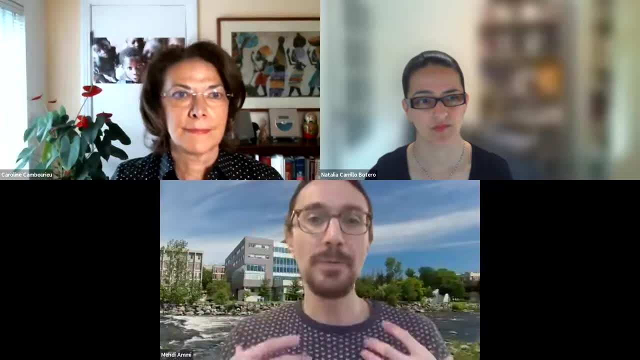 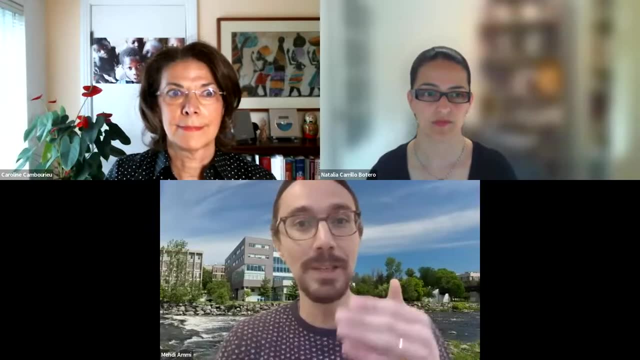 or there is too much money, We just say OK, that's how much is spent, And we don't adjust for the difference in populations beyond the fact that it's a per capita difference. But in Ontario there are like 40 million people. 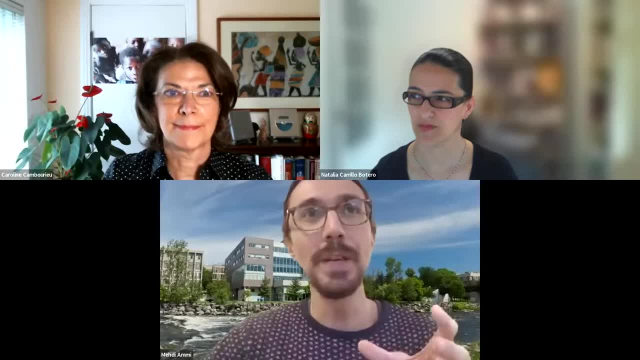 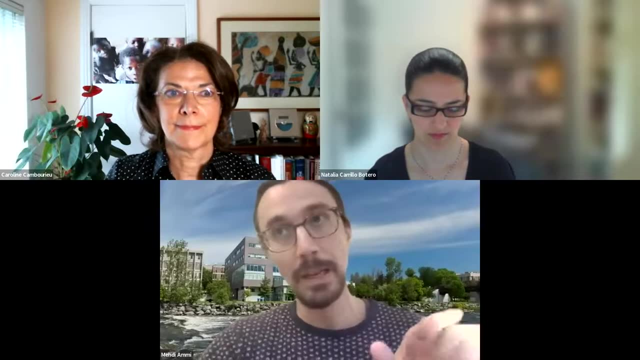 And in Quebec there are 8 million, et cetera, et cetera. So we just don't do that. Yeah, Yeah, We don't do that, And so that's going to be the short answer. We have another paper where I'll try. 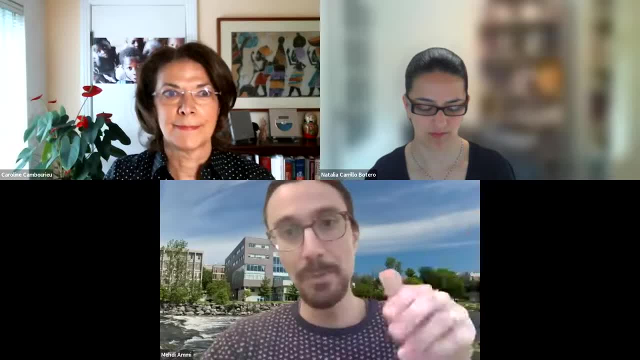 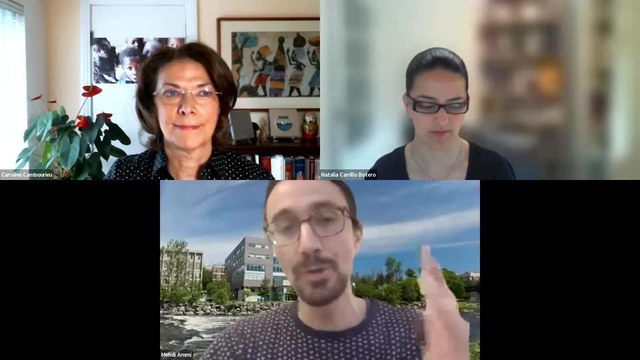 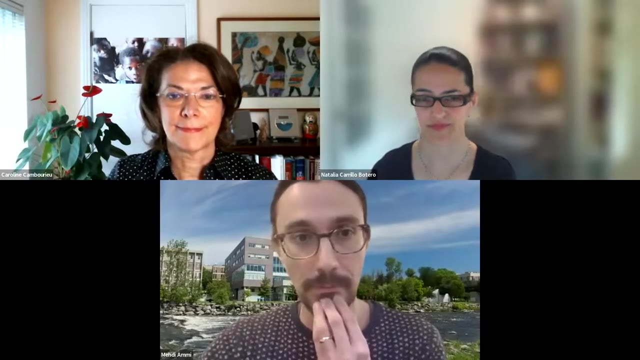 to link the outcomes with the spending, But in this paper that I presented today it's not there. Thank you, Another question, Natalia. Yes, I continue. So we also have another question about the numbers. Were numbers adjusted for purchasing power party? 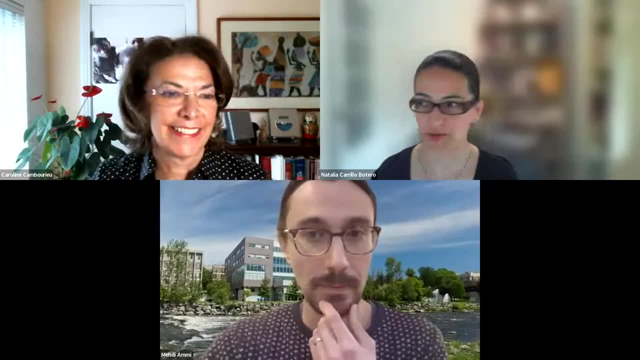 I've seen the data below. So, Dr Ami, there is a link in the Q&A. I don't know if you can click on it, I'm just seeing it. Yeah, yeah, OK, I see. On the World Bank. 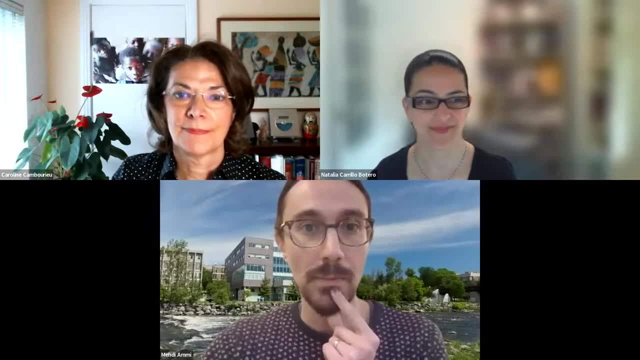 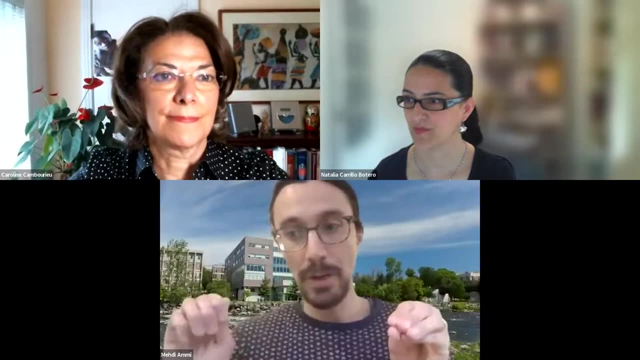 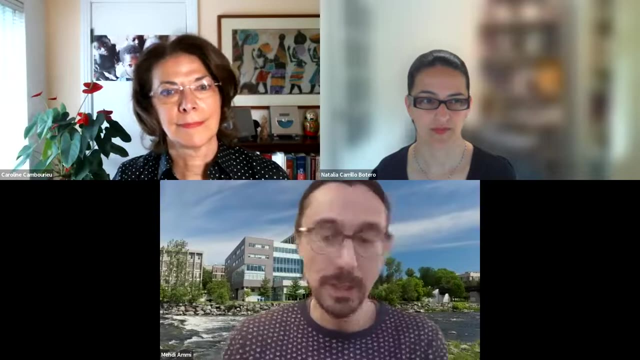 Yeah, but I think just yeah. but this is in Canada. OK, we are not comparing Canada to something else, We're just looking within Canada, different jurisdiction, So there is less sense of adjusting for purchasing power. We are seeing the difference using the CPI, the price index. 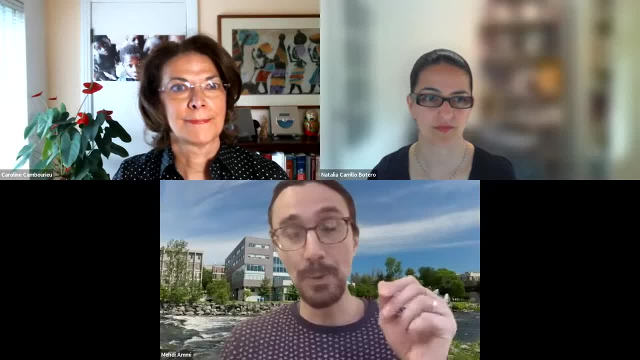 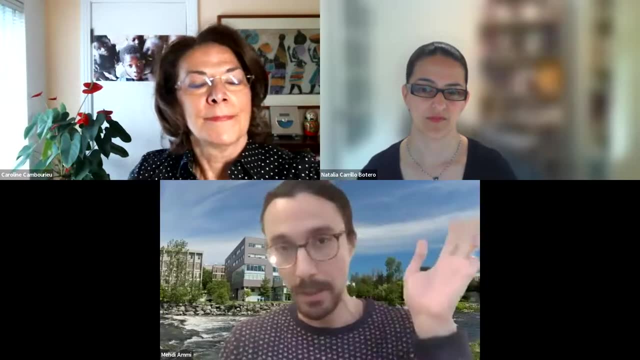 But that is just adjusting for inflation. But we don't try to say Canada, Canada versus, I don't know, Australia or France there. So that's not something that we necessarily need to do. What you say is for an international comparison. 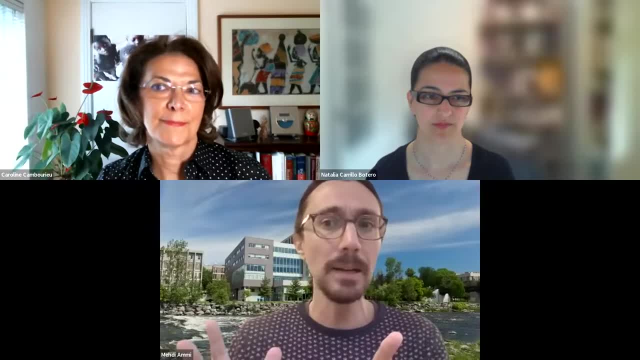 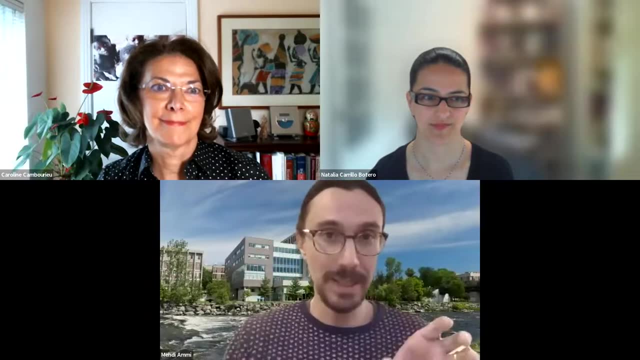 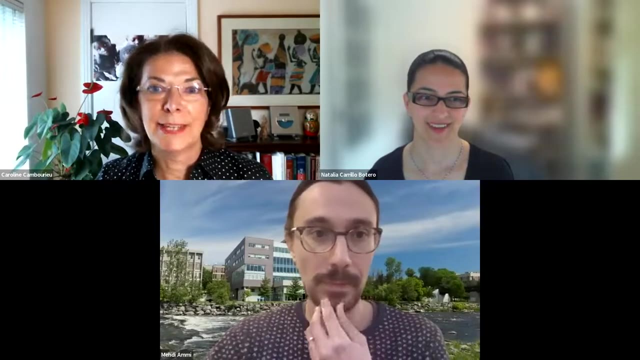 But here we are within Canada, different jurisdiction. All right, thank you, And I'm going to group these two questions in a two-part series of questions because they're related. So it seems to me that it's possible to have rising expenditures but still have this. 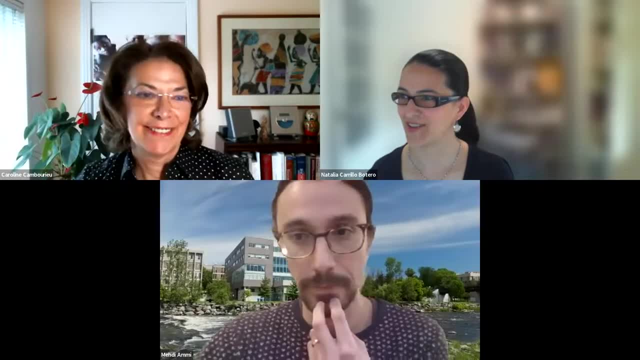 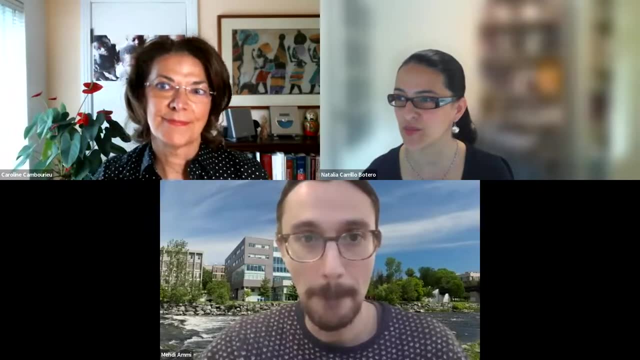 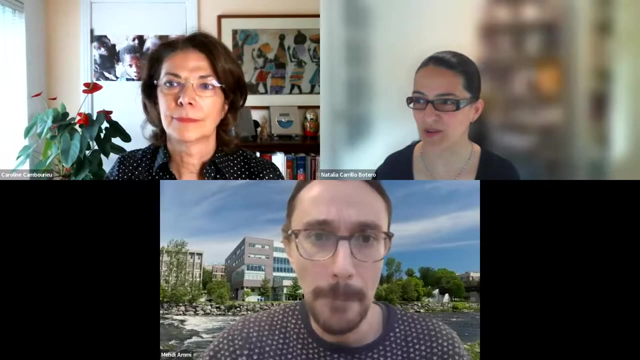 Expenditures being sufficient, particularly if you have a view of health promotion that focuses on the importance of investing in social determinants of health with more urgency than growing clinical or medical services? Would you agree with this? Will your work engage with these kinds of questions? 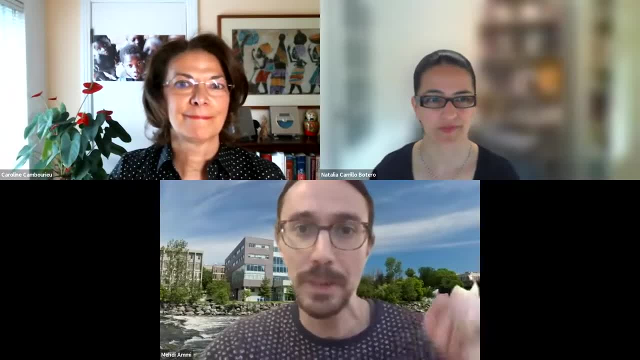 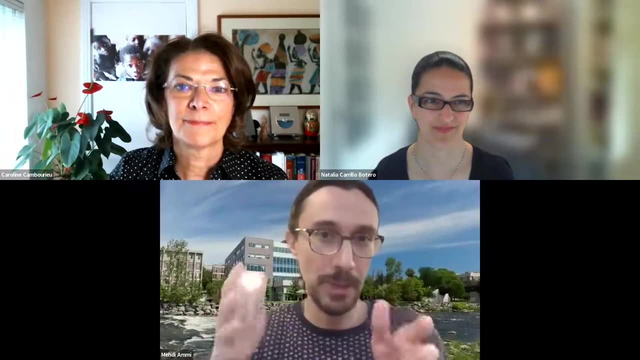 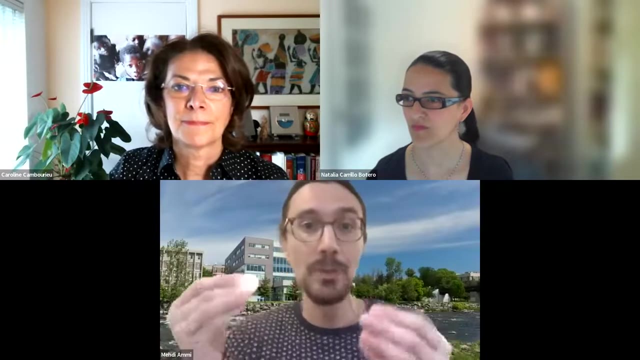 about relative expenditures. Arguably social determinants of health investments will be outside of health. Slash Public health Expenditures. Public health, that's a whole other expenditure discussion. Yeah, that's the next question. essentially, You're right. 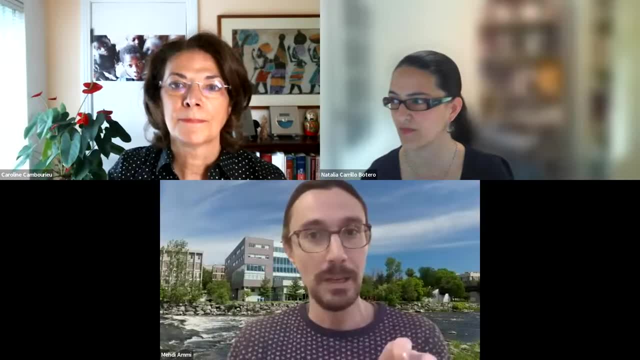 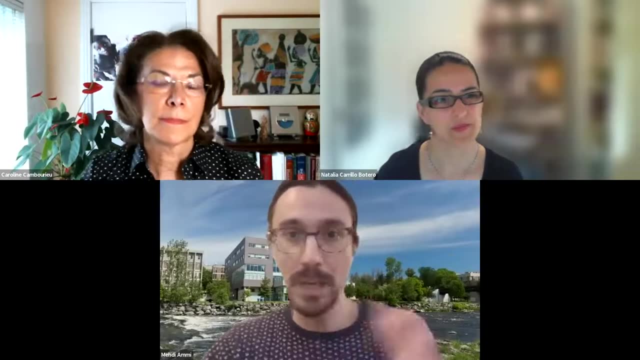 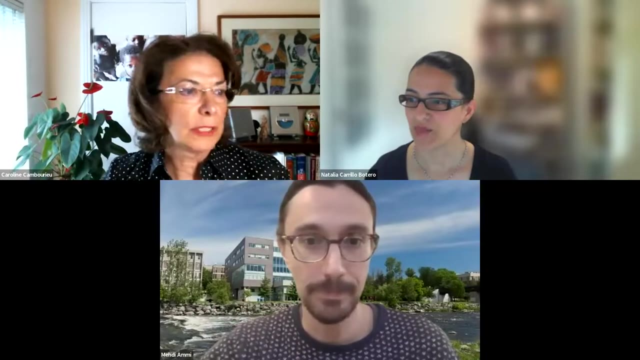 That's the question about value. The current question is saying how I mean. what the paper I presented today, sorry, is saying is: how has public health expenditure grew? But it's not pretending that this growth is justified or not. It's just saying we observe growth and it's, in a way, 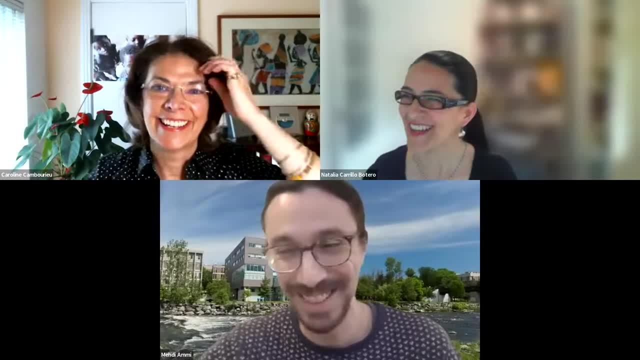 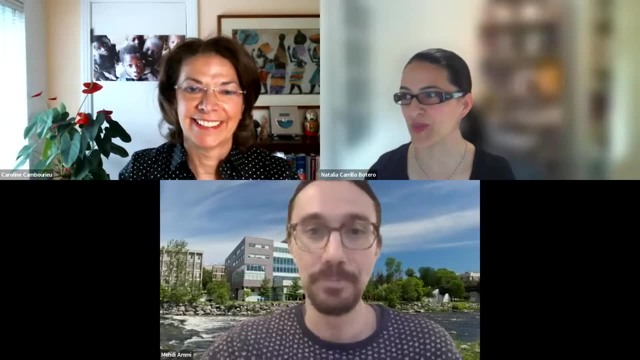 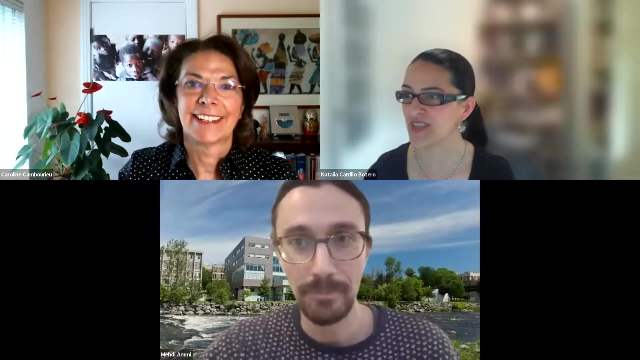 giving us some information about the choice that were made by government in just allocating the health resources to our different utilization. So we don't know if this is enough or if it's too much, And I'm not going to say because Canada is spending the most. 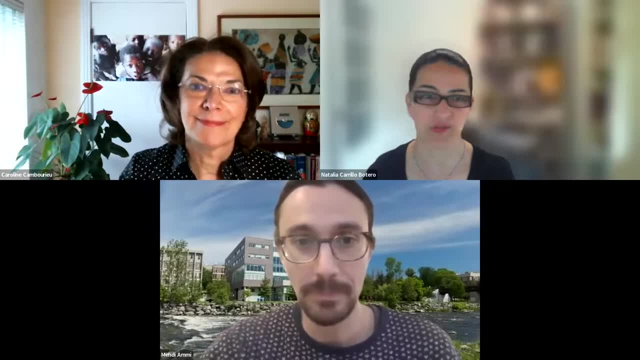 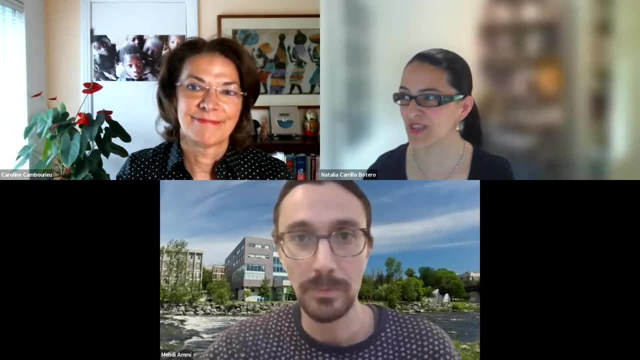 that means that we are spending enough, because we don't know the results in the UK, We don't know the results in Romania, We don't know the results in Greece. We just don't do that. That's the follow-up question And you're right, that's an even more important question. 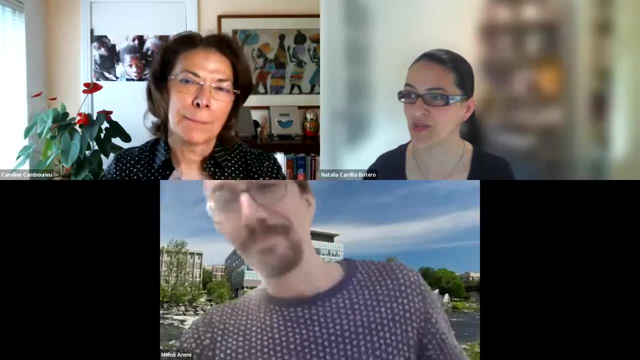 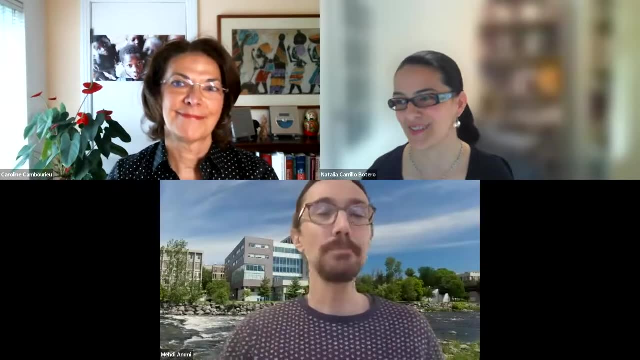 But our view was: let's start to do the first step- understand how these things have changed- and then look at outcomes. So we are looking at outcomes. This is the paper I briefly alluded to in the conclusion. We are looking at avoidable mortality. 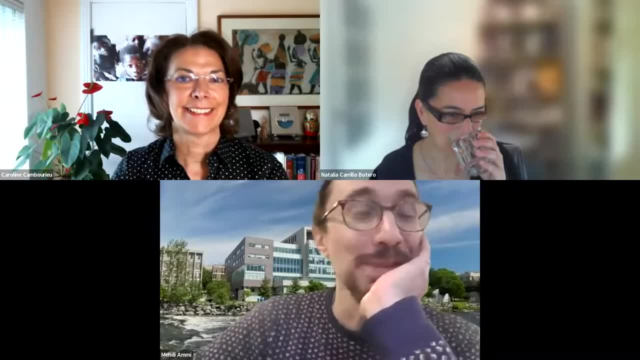 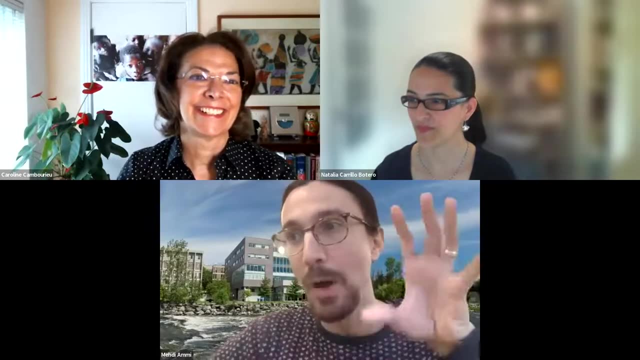 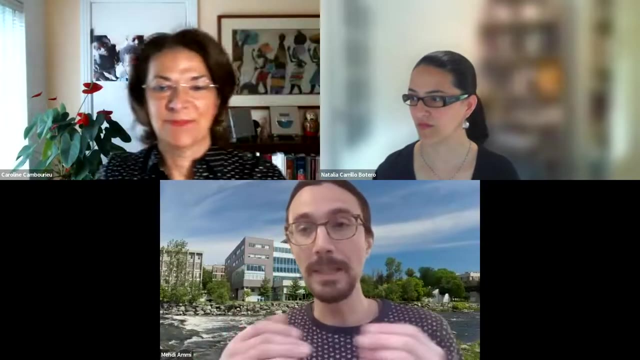 from preventable cause, because we're just trying to find one outcome where we think public health should have- sorry, a broad Effect. And we are also looking at this long-run relationship because we just are conscious that public health is just going to be a cost now but outcomes later. 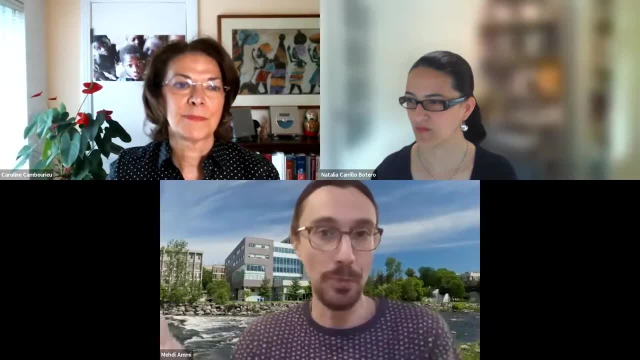 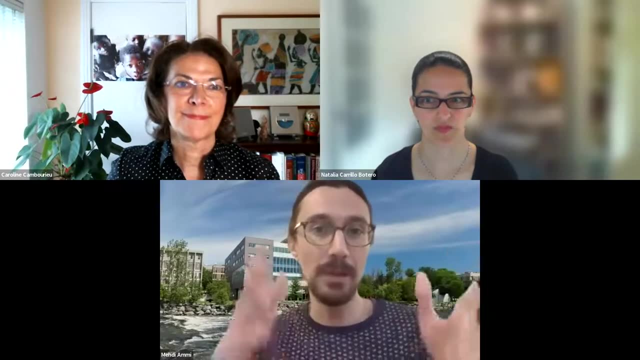 So we just want to allow this to happen. I'm not going to say more on that because it's still a work in progress, but that's what we are doing. And on your point on social determinants of health, you're right that we don't. 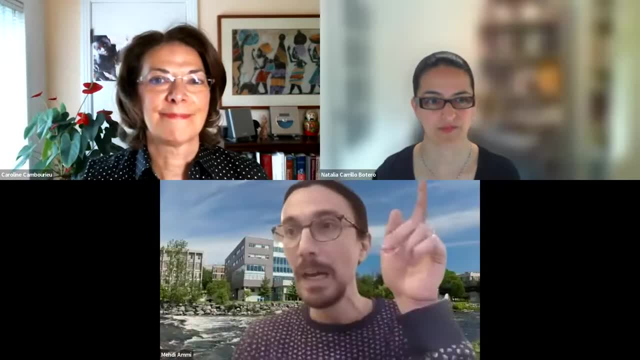 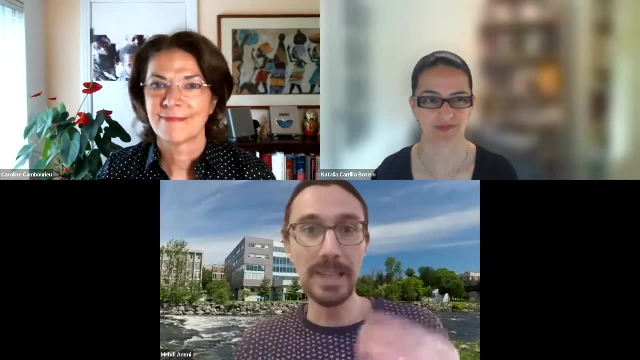 I mean, this is the way CAI collect the data. So in some sense we don't have the data, We don't have the data. In some jurisdiction they receive information, let's say from the Ministry of Education, and there's a school vaccination program. 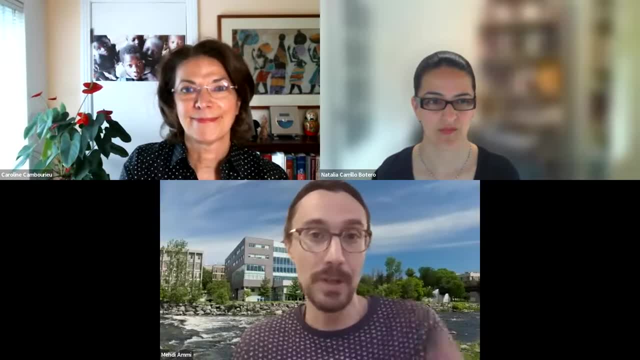 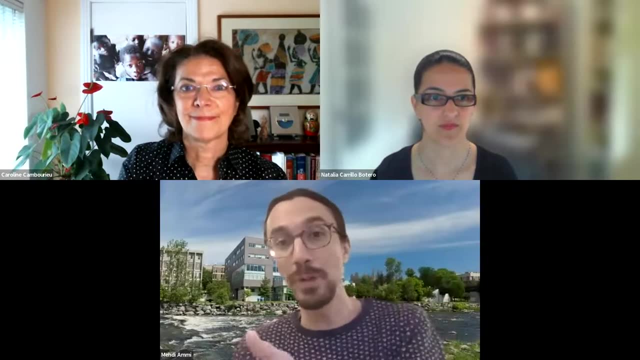 that is ongoing in education. So it's not exactly social determinants of health, but just saying, well, the money may come from another- birth, education or labor or environment. So we don't see this all the time. Our focus is really tightly on the health responsibility. 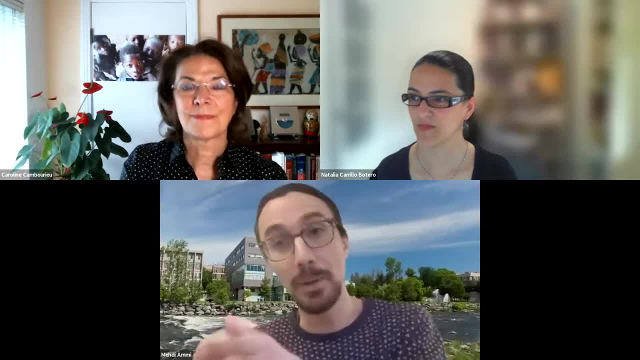 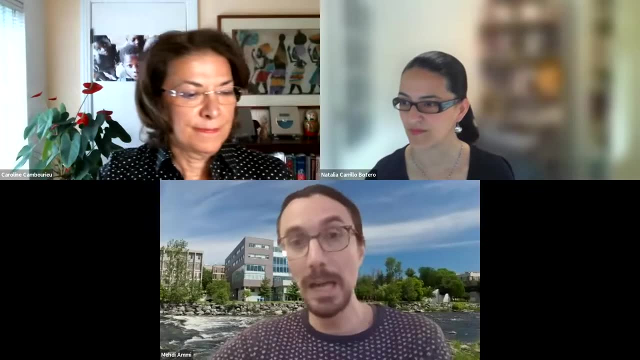 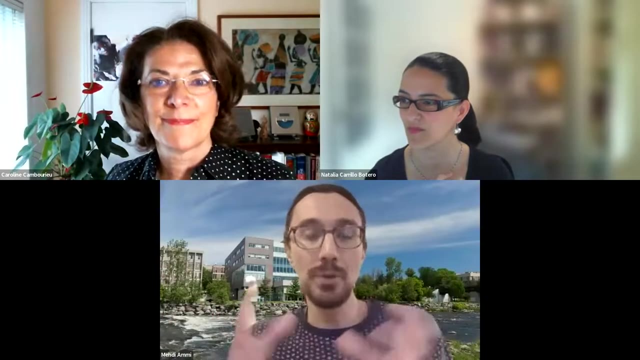 Sometime. there is a little bit else, And the first question is knowing what do we obtain from this public health expenditure that we are able to track from the data and health outcome. And the question after will be: well, how do we know if we need to account? 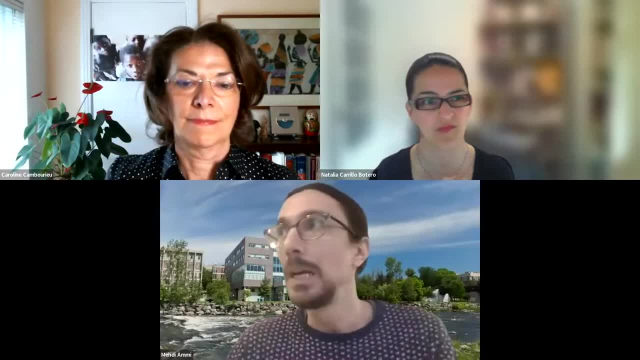 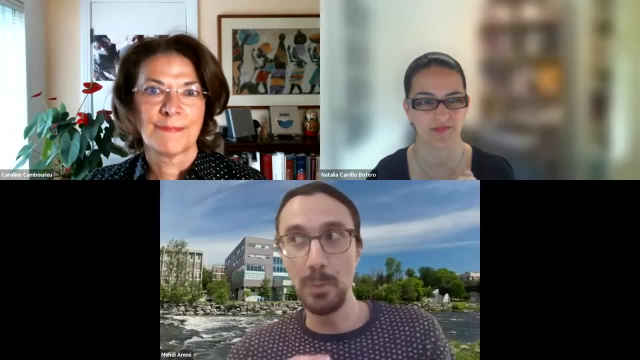 for like investment, I mean expenditure in education, expenditure in environment, et cetera, et cetera. Sorry, that was a long answer, Thank you. Thank you, Mehdi Natalia. maybe I could go with the question. 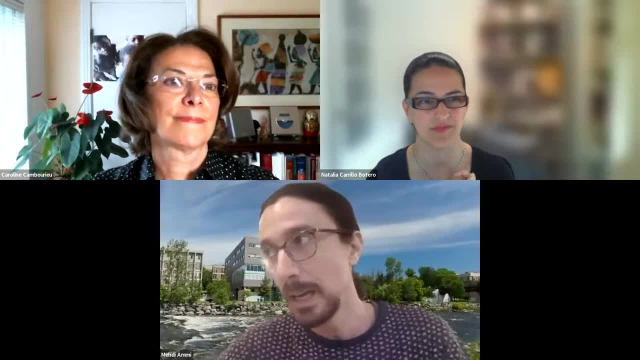 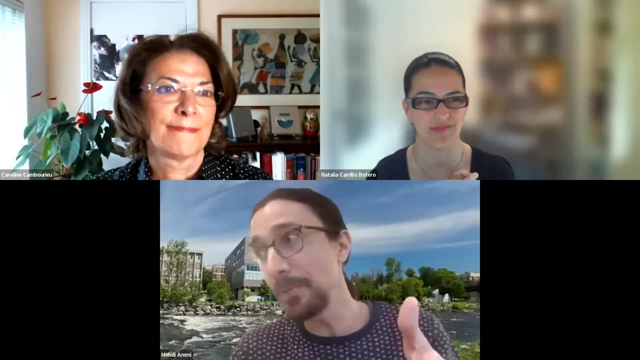 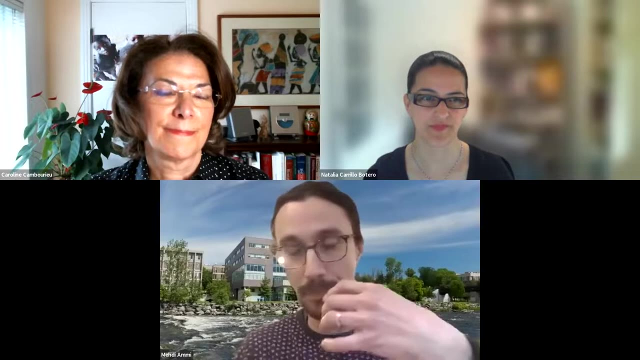 from a participant that registered. And there is the following question: Mehdi, Considering the trends from 1935, 2018, what do you expect to see in the next few years with regards to public health expenditure? Yeah, so this is a question about making a guesstimate. 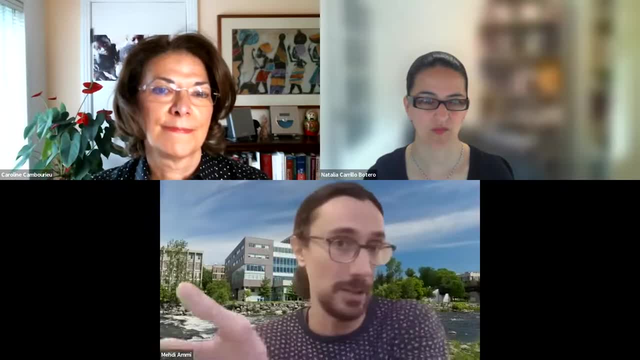 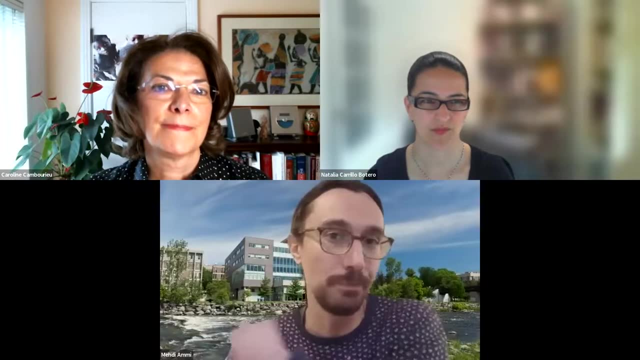 You know it's not the forecasting, it's just based on seeing. I've been trying to have a quick look about all the correlation of the public health expenditure, of spending and public health crisis and see you know if, because there is this idea of reactive spending. 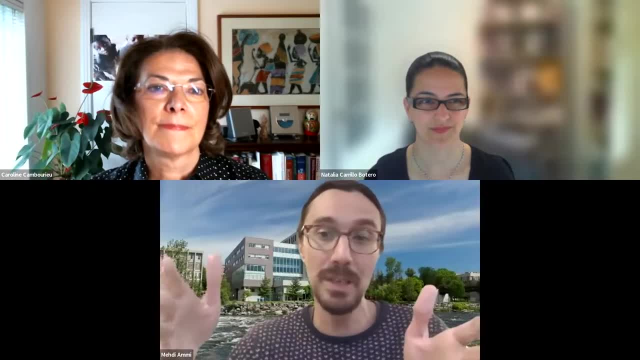 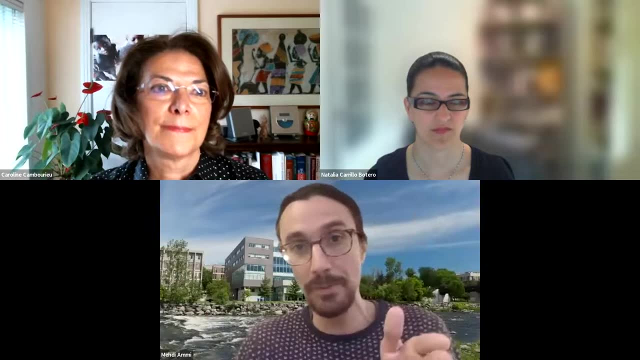 and that sometimes, if you have a crisis boom, a lot of money is spent in public health and then the year after falls down. And what I've been seeing, what I've been seeing there is just like we see the same kind of story as with SARS. 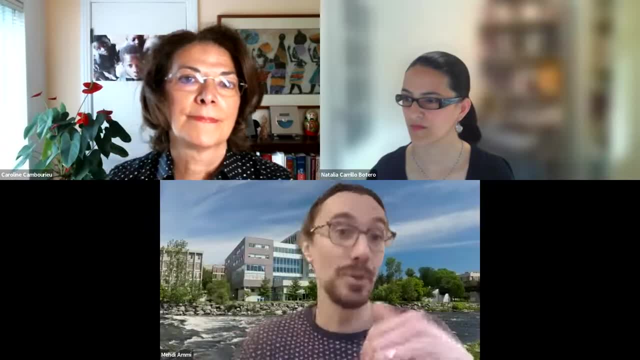 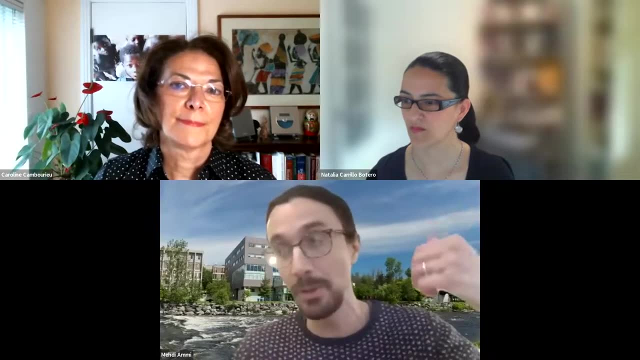 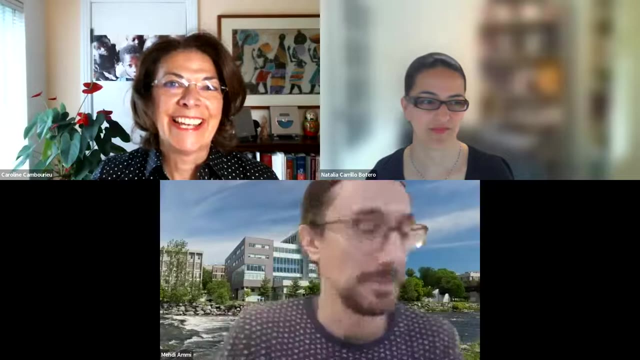 and with H1N1, where we are like this kind of small increase, small correlation between the number of cases and the increase in expenditure, Not everywhere, And then sometimes it's there at the level, sometimes it goes down, So that's just like for the public health. 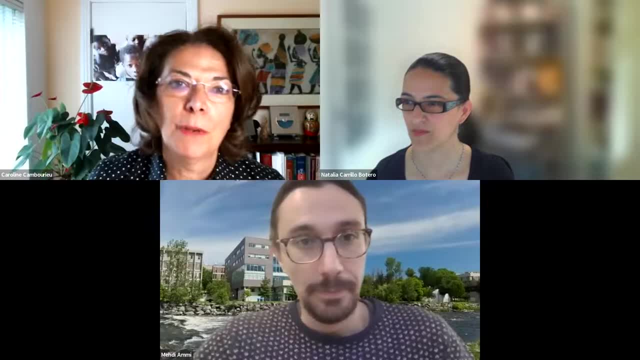 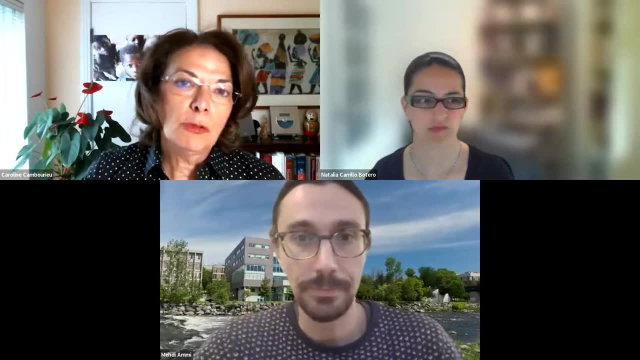 there may be a sense that's just going to go slightly up. but now the data has been changed. A new classification has been created for COVID spending, and COVID spending as some of the stuff that is public health and some of the other that is not public health. 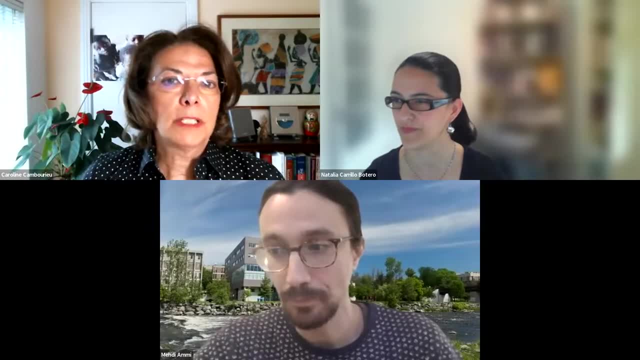 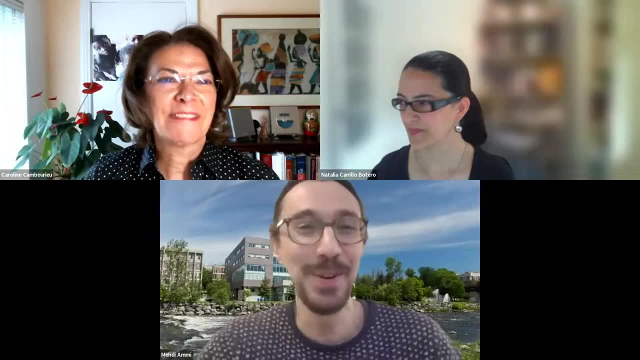 So that's going to be a new challenge to understand. The other thing is looking at. you know, when you look at hospital spending, if you remember from the graph how it was like pretty flat, I mean not super flat, but just growing very slowly. 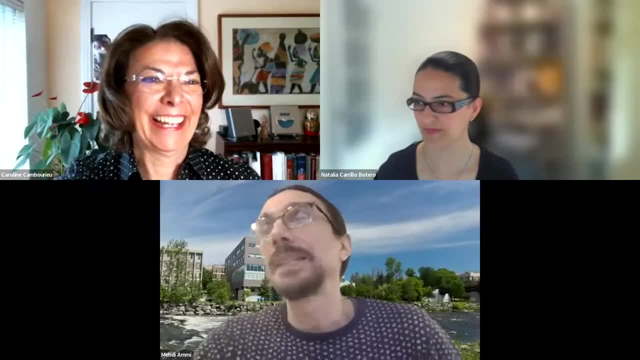 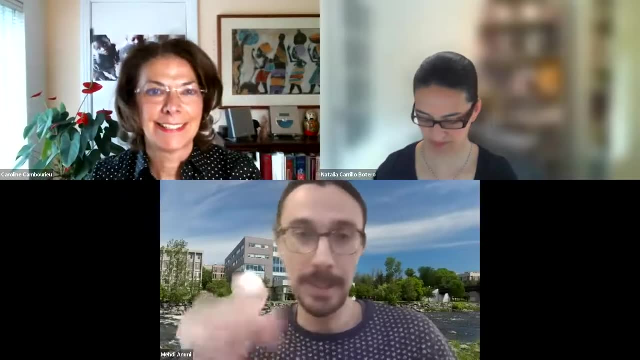 If you think about all this question- about, you know, not enough beds in hospitals, the workforce burning out, et cetera- you can imagine that there is going to be like more going to the hospital in the coming years. And the last part is: 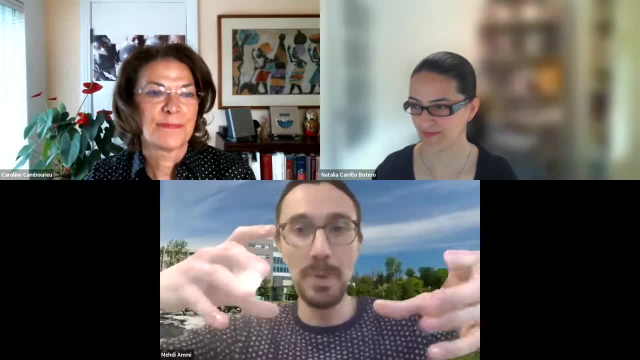 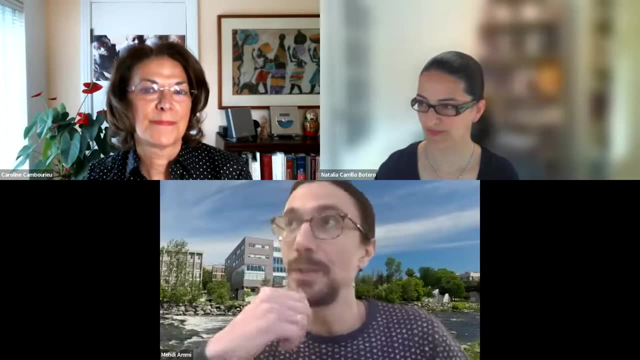 stagflation. So we don't know what the Central Bank of Canada is just going to lead to, but we have some, you know, we can foresee that. you know this idea of fiscal retrenchment that happened in the 1990s. 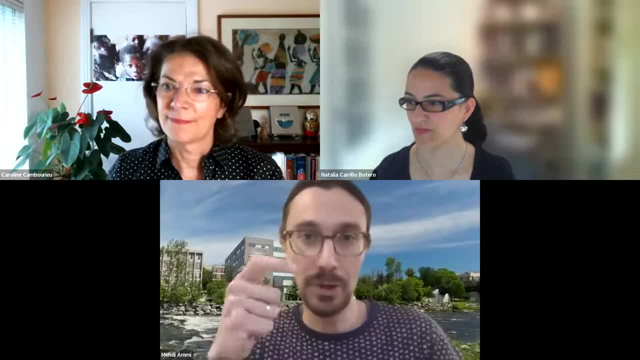 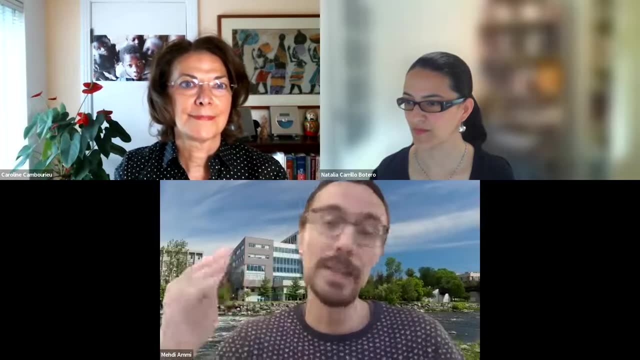 may happen in the coming years And if it happens, what is interesting? it looks like that public health has been relatively protected when you compare in the 1990s, compared to the other sector. So it might be like I'm just trying to say. 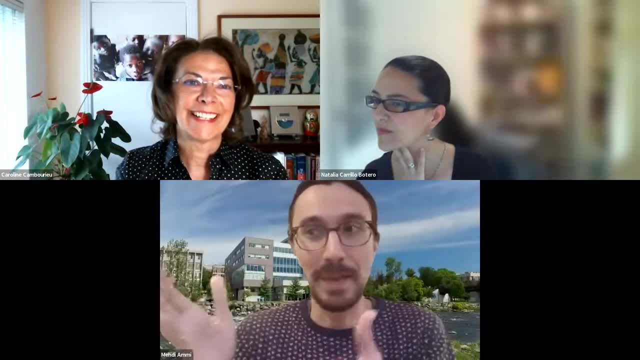 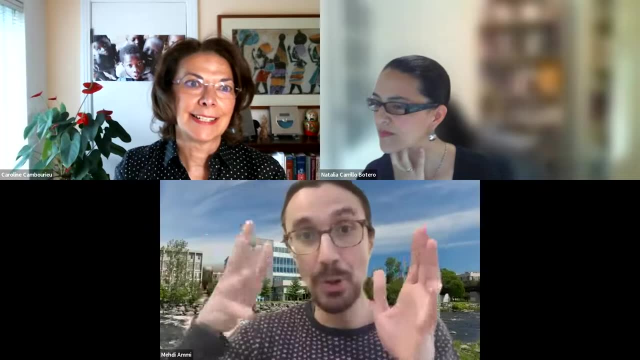 okay, but my guess in that is: public health is likely to be protected, especially because of COVID, But you can imagine that's not going to grow a lot, but the hospital is likely to grow more because of all the pre-existing, pre-existing issues that were there. 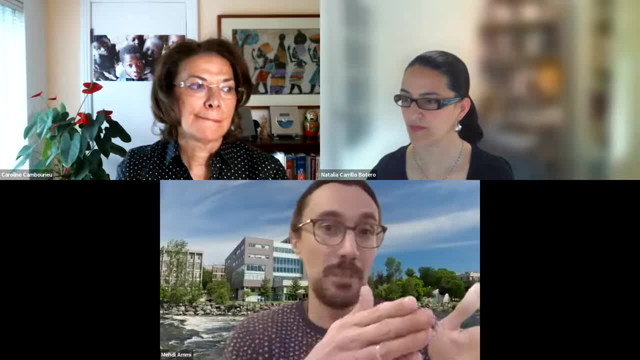 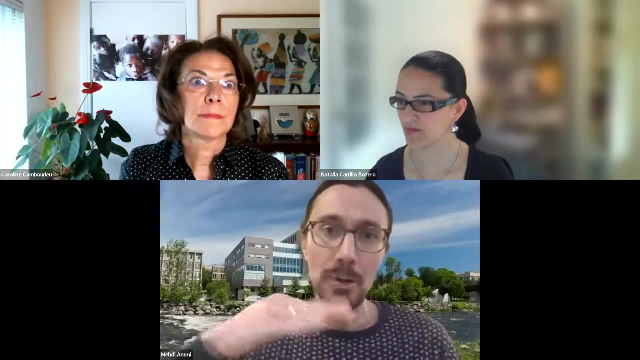 but has been like, made like front and center because of the past two years. So, thank you. Thank you, Steven. Yeah, thank you very much, Natalia. do you have another question from the participants? We do, we do. 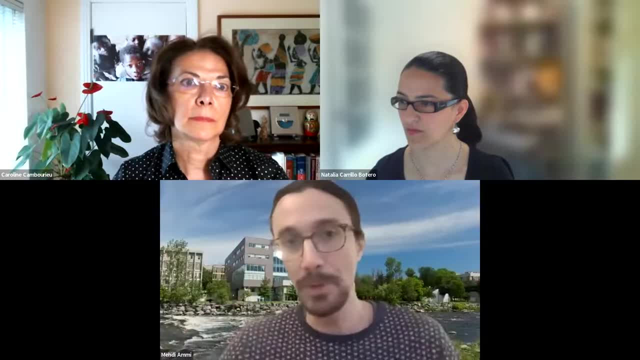 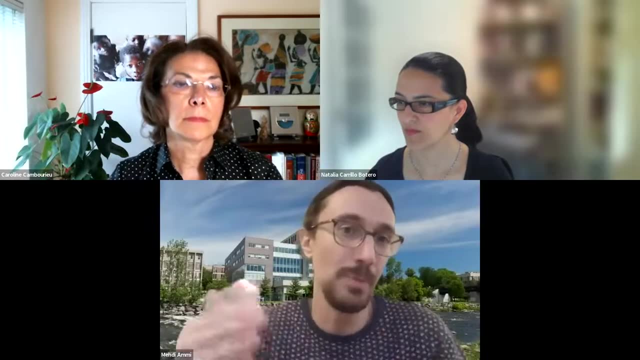 We have a lot. Thank you to all the participants And I think, Dr Ami, that we had at least two or three questions around the same idea of social determinants of health. Okay, I have to all of you. 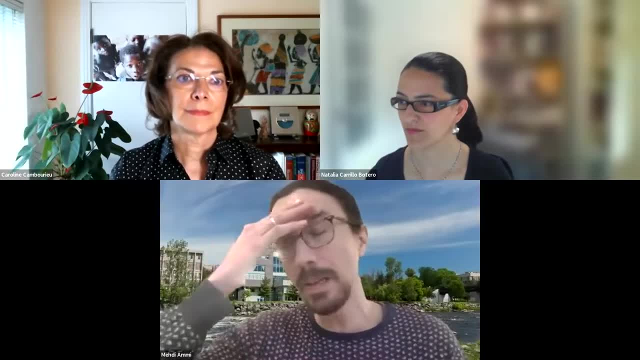 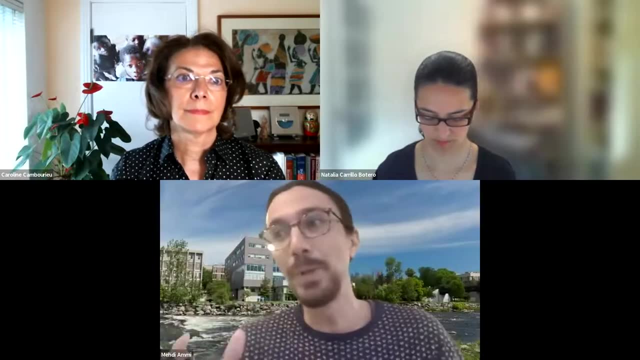 I have responded in the chat because I believe this has been answered. If not, just write back to me and we will follow up. So then, next question in the chat: do you know approximately how much of the public health budget is immunizations? I have worked in Ontario, Manitoba and BC. In BC, public health administers the majority of immunizations, including the infant series, which has expanded great over the past 40 years. Could the increase in BC expenditures actually be pretty much attributed? 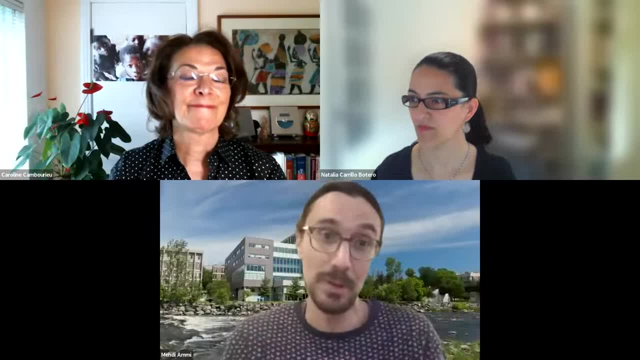 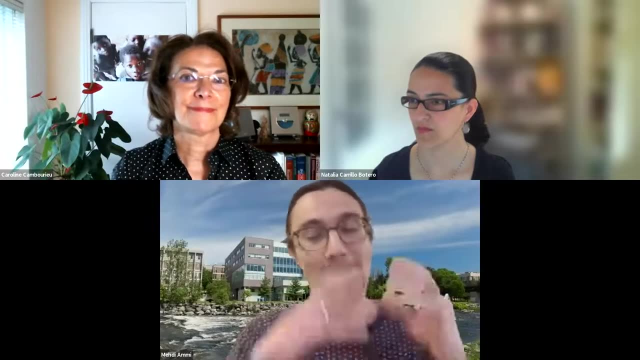 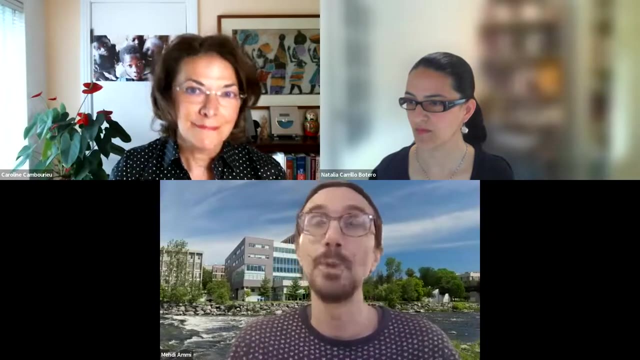 to immunization, purchase and delivery. That's a great question. I don't know for sure because what we observe is the segregate PPH category And actually we've been working closely with CAIA and recently we've been given access to what they have. 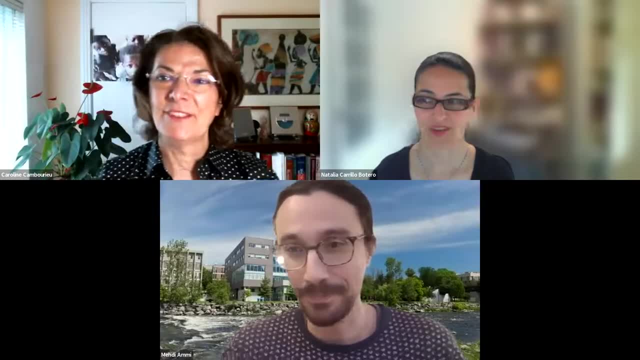 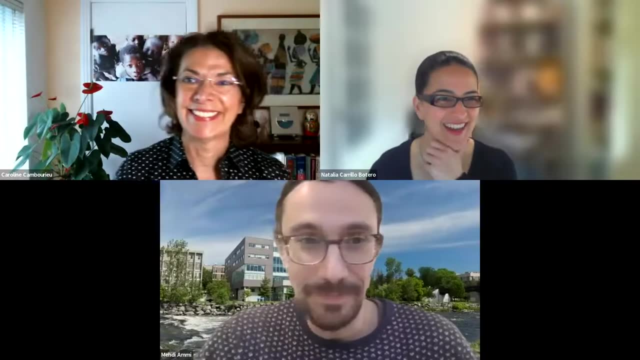 you know the detailed to the detailed level. So I would likely be able to answer your question in one, one year from now. but at this stage I cannot say for sure that this is the main driver. but if you have experience and you can say 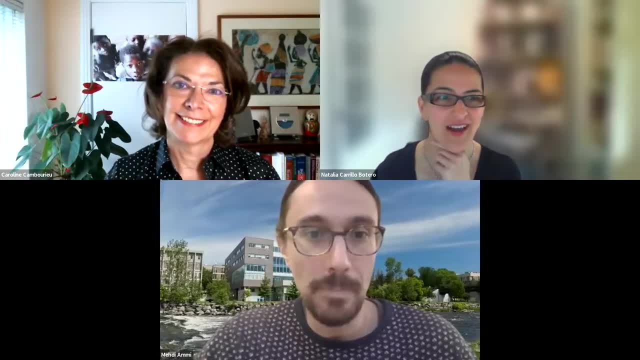 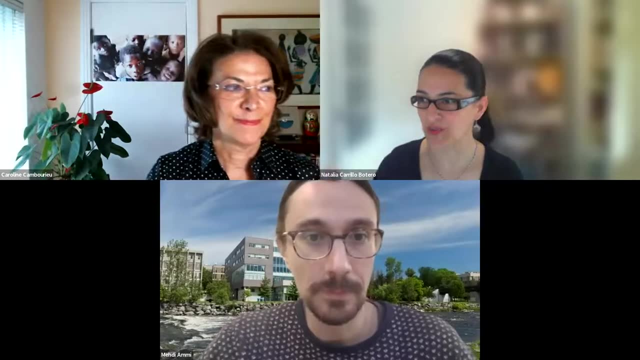 well, I think that's a contributor. I yeah, I honestly don't know, because we did not observe that in the data, Thank you. Thank you, Mehdi Natalia. maybe we could go with another question and then we could go back to a question. 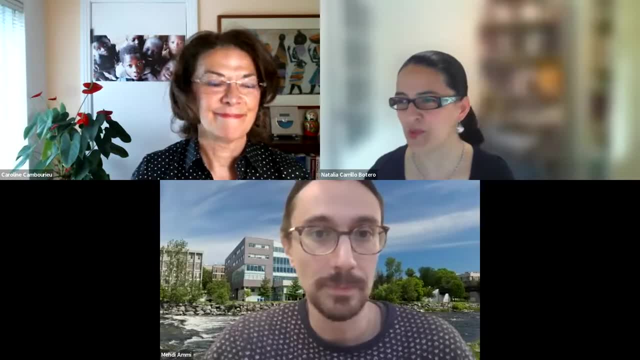 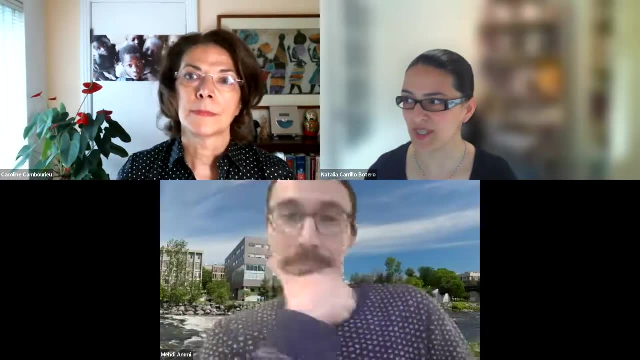 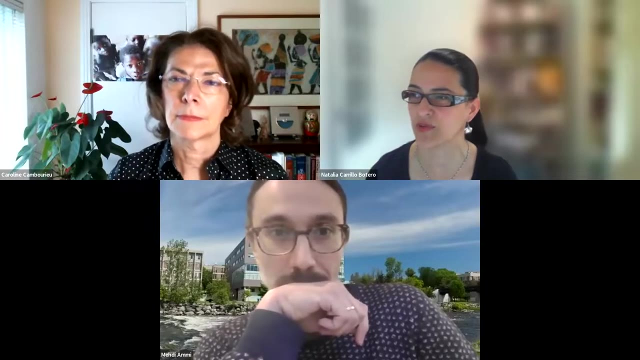 from the participant that registered, So I'll let you go with another question, please. Okay, Perfect, From the list of countries with public health expenditures. what is the quality of life and are there the life expense? wait, sorry, apologies. 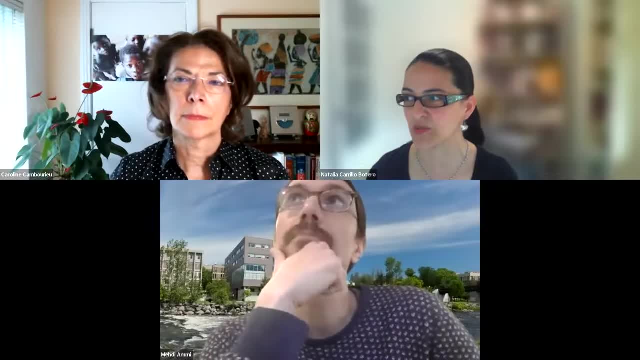 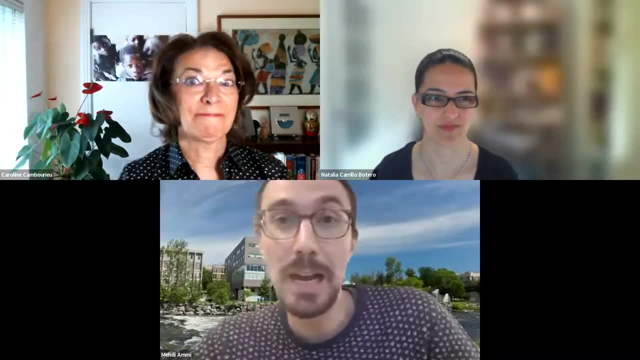 From the list of countries with public health expenditures. what is the quality of life and are the life expectancy the same? So what? I think this is the same question about the value, you know, the same kind of idea that you are just looking at spending. 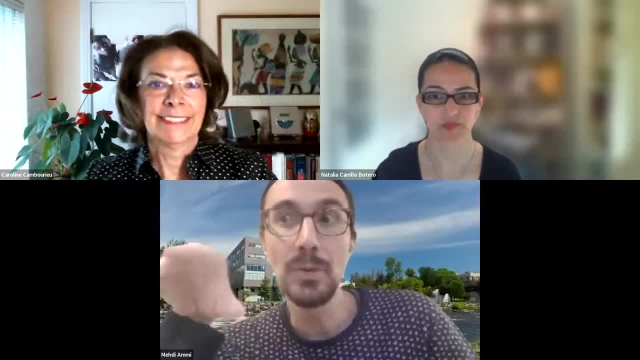 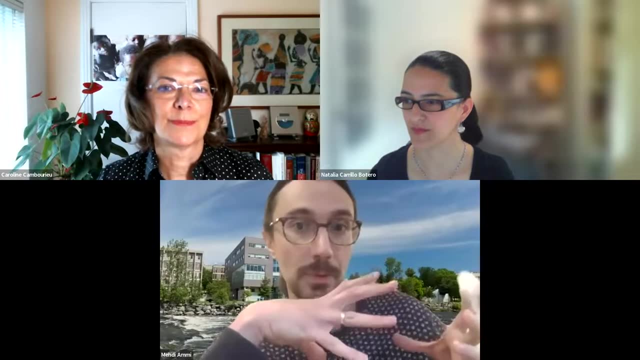 and we want to know what we get from that. So I'm going to make the same answer. We have not looked into it yet. If you want to know if Canada is doing comparatively better than because it's the top spender in public health, 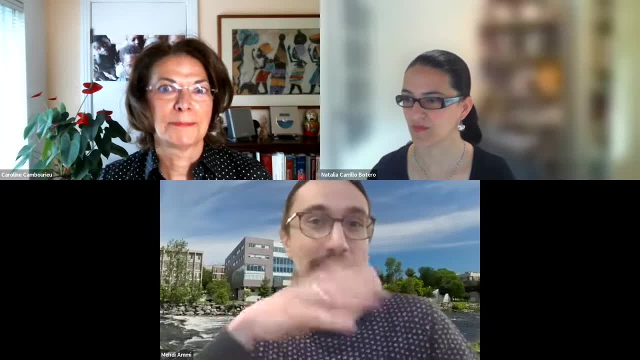 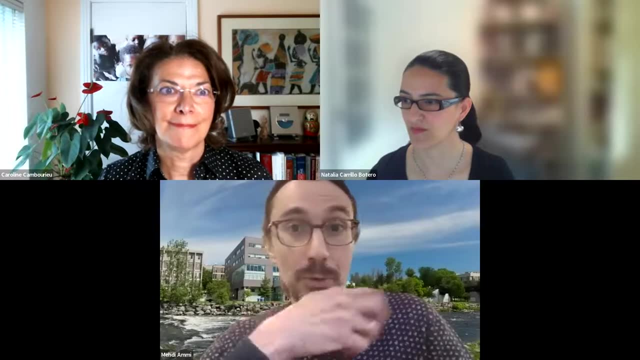 compared to the OECD. in general, the answer is no, it's not doing much better. It's the middle of the pack. So there is I. we cannot say that. okay, Canada is spending so much on public health. I mean the highest share. 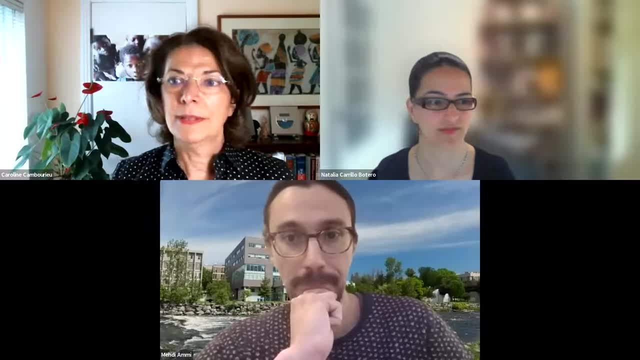 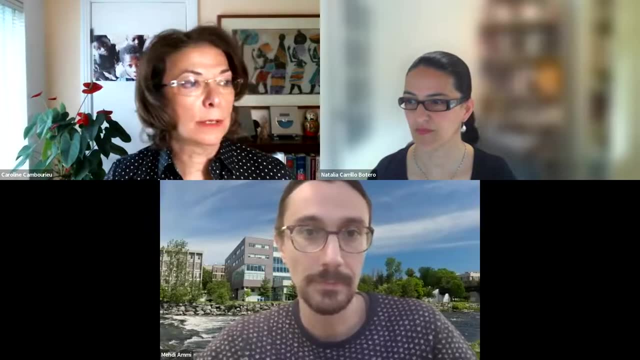 and that's something that we can, you know, immediately see in an adjust analysis, just simple comparison by better life expectancy or better quality of life, or better, yeah, better quality, or whatever you can think of Middle of the pack, really. 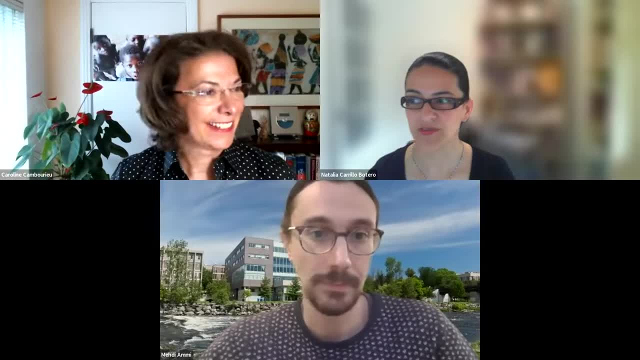 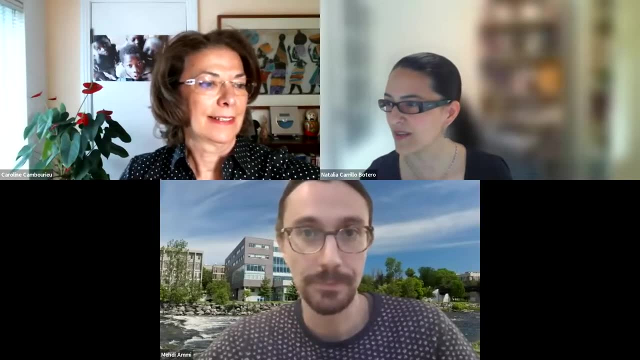 That's what where Canada is. It's not horrible, but it's not like awesome, Thank you. Thank you And Caroline, I wonder. just sorry to interrupt. I have a voted question, So I wonder if it's worth asking. 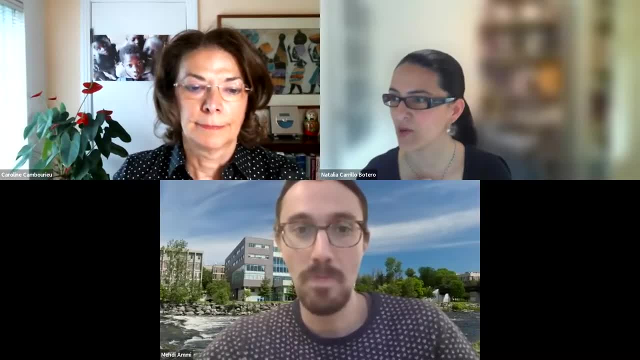 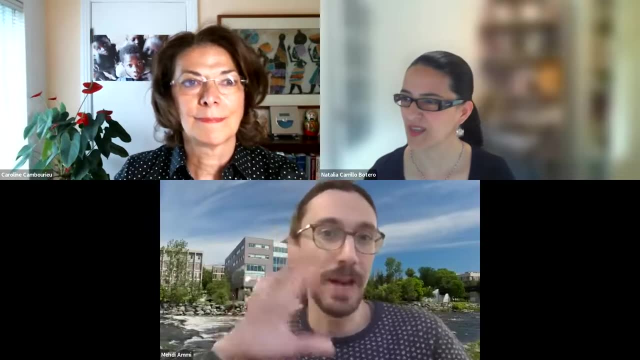 Good, good, good, go ahead, go ahead, go ahead, Perfect, perfect. So many of the investments that benefit public health occur outside the health sector, for example, investments in education, transportation, environment, et cetera. How do we account for these investments? 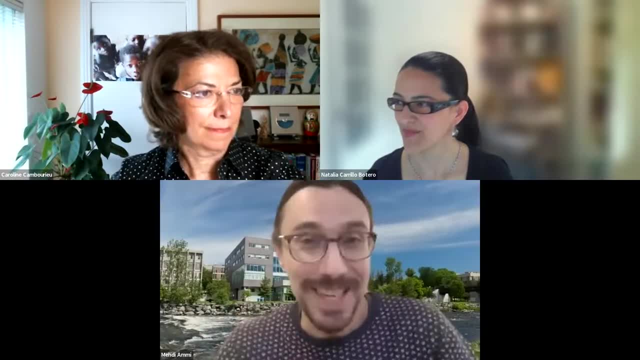 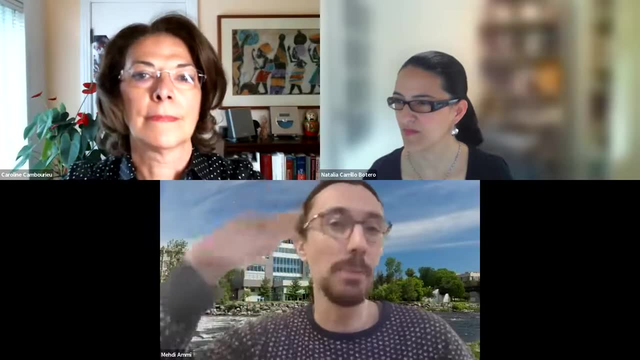 Shouldn't they be considered as well when we look at trends in public health spending? That's just. that's a great question And this is not. this goes back to the point I was trying to make about defining public health. yeah, 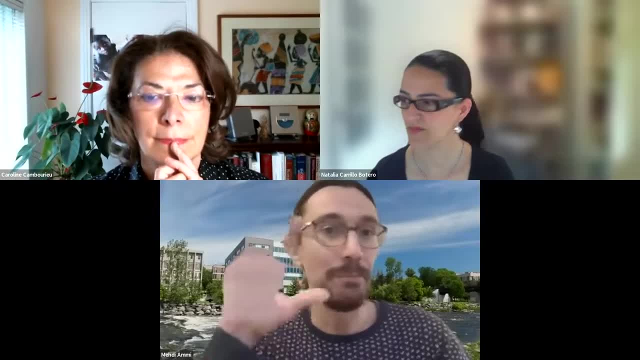 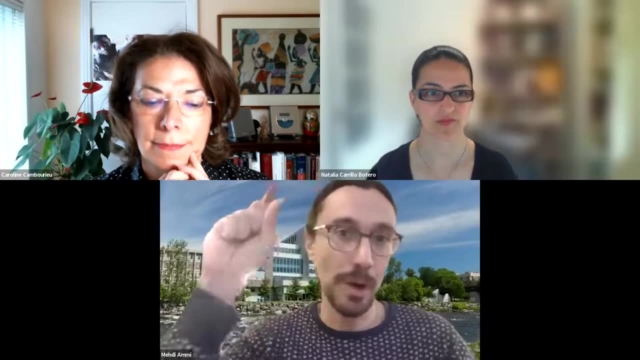 Which it's because public health is. you know, because public health is so broad, you can expand the perimeter almost infinitely, And everything is going to have an effect on the health of populations. So everything is going to be pretty kept. My view, and this is just my personal view- 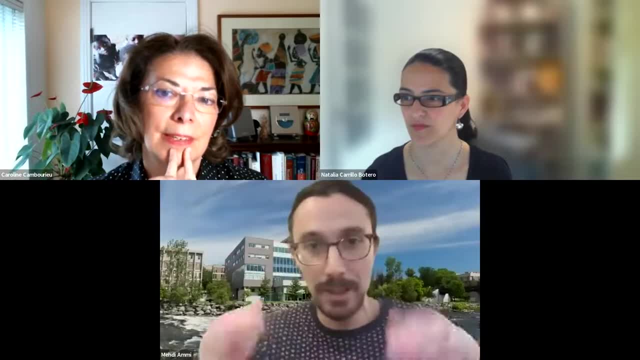 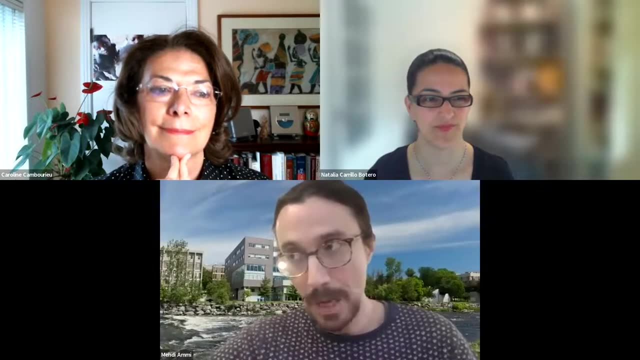 is that it would be counterproductive to go this road, because then attribution becomes extremely difficult. You cannot say: well, I spent so much on public health and I got whatever outcome: increased life expectancy, less avoidable mortality. First part attribution issue. 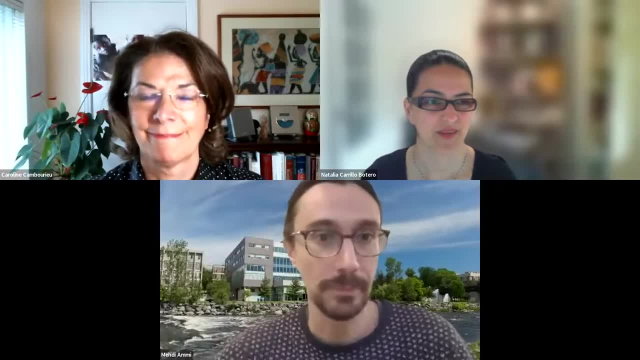 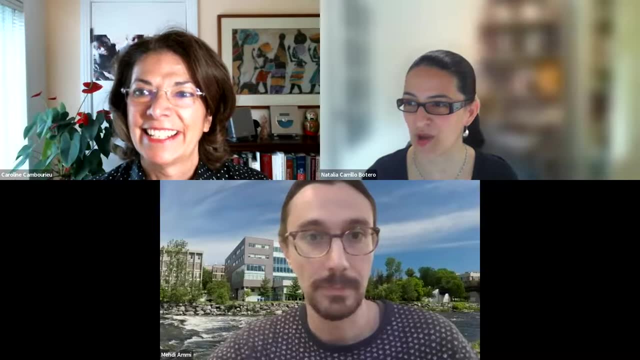 Second part is saying well, this is not good saying well, we're already seeing. but based on how CAI defines public health, there is a large growth across the board, except in Quebec and Nova Scotia. And, as I said, 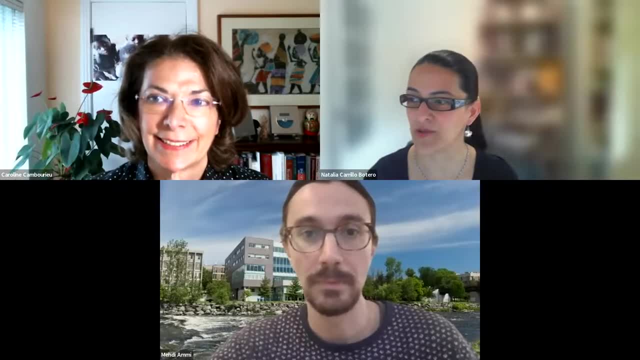 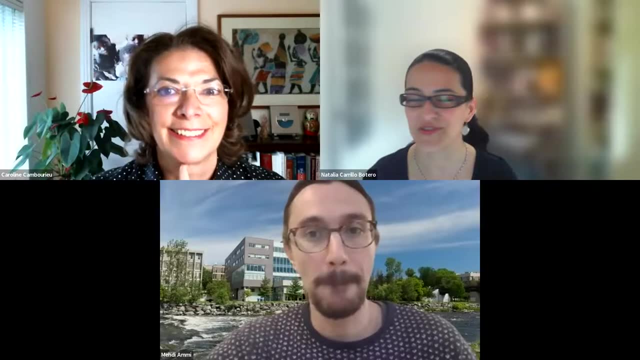 Northwestern territory And if you look at the paper you will see there is a jump Northwestern and you see just flat, flat, flat, jump and then flat again. So something happened at one point and then didn't move. So I guess I will not my. 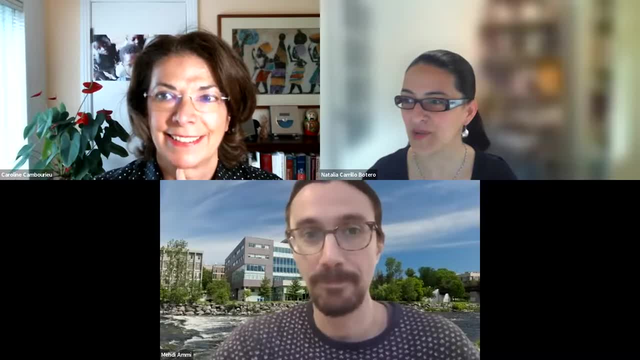 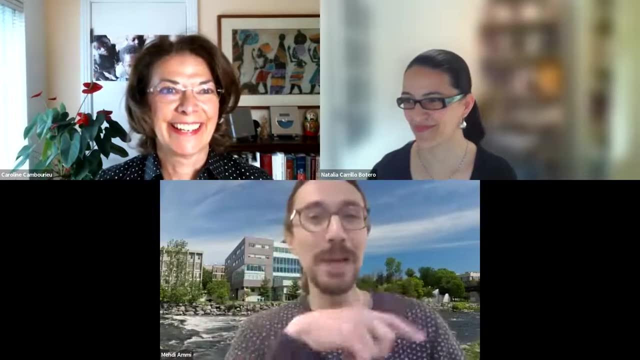 personal view would be. I think it's not the right way to look at it for now. It's better to keep a focus on public health system in the narrow way when you think about expenditure, because if you start to try to tease out, let's say this: 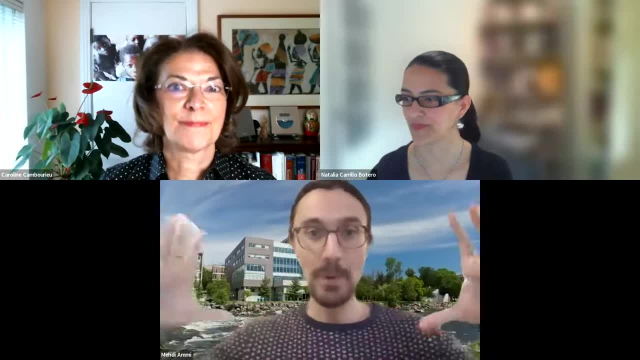 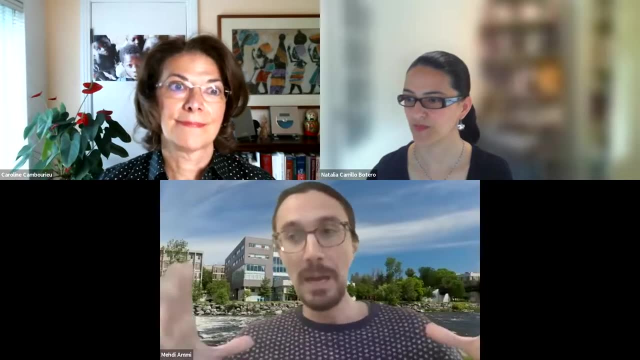 expenditure on, I don't know, pollution control is just also part of public health. you are going to see that the public health expenditure is just going to grow like crazy, And then the value for money of each public health dollar is going to be. 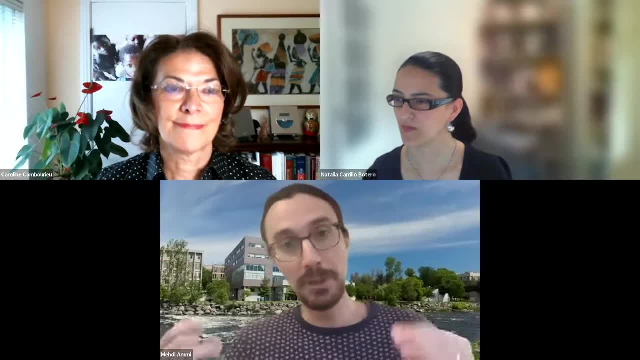 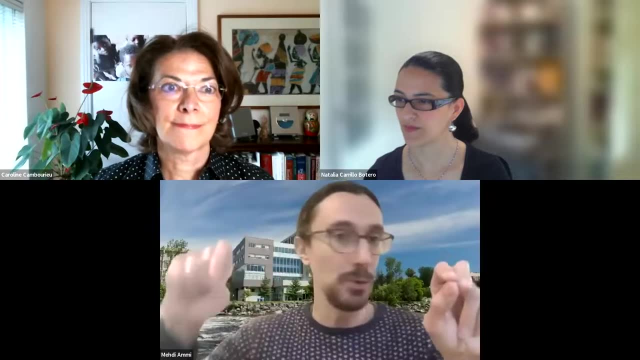 mechanically go down. I don't think this is something that makes sense in my view, but that's just my view. Thank you, Medhi. Natalia, I'll let you go with another question. Okay, good, We have more questions here. 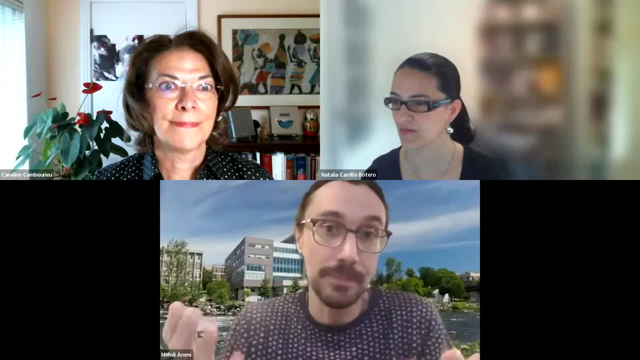 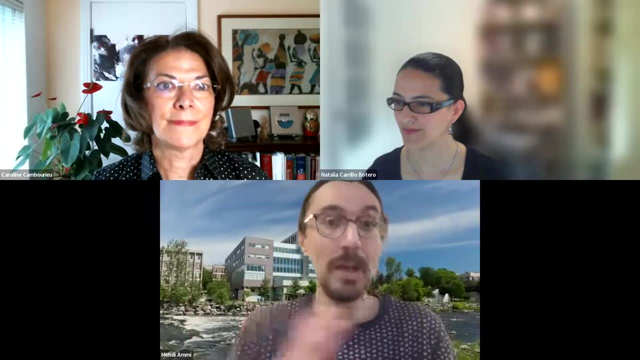 Well, I have one. Sorry, It's up to you. This is a follow up for the first question about the numbers. Thank you for the clarification. Do you have any idea of the portion of the expenditure? What are the features for public health that does come from? 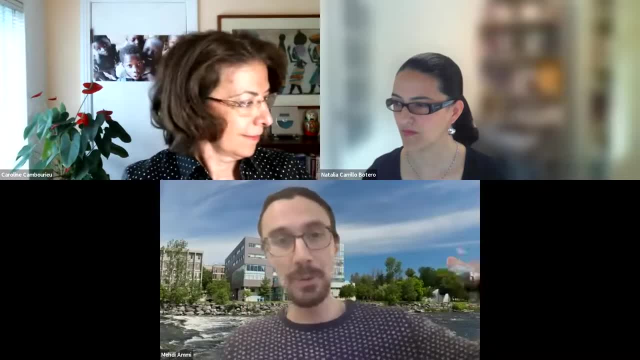 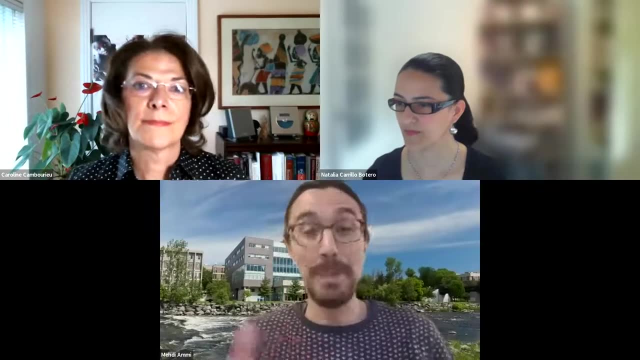 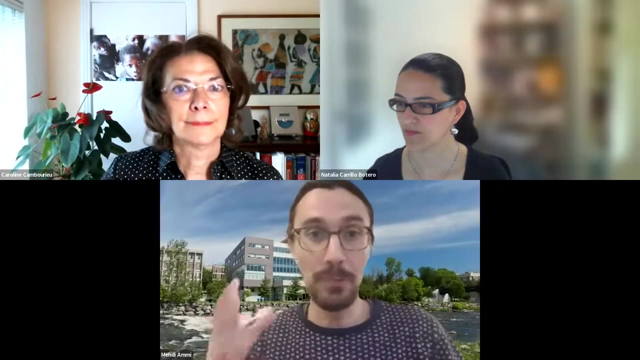 municipal taxes. Yeah, so I will not remember the numbers from the top of my head, But what I can tell you is that this is essentially a story in Ontario where you see that there is like public municipal spending- I mean municipal public health spending, that is. 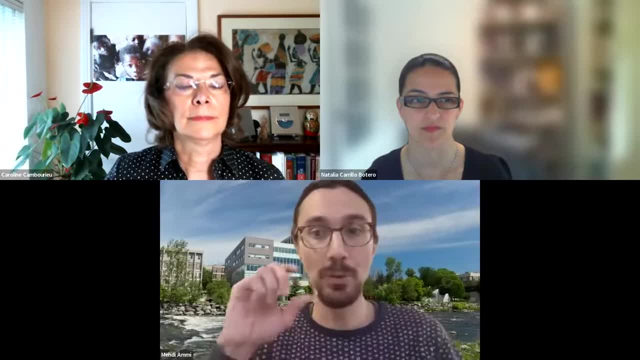 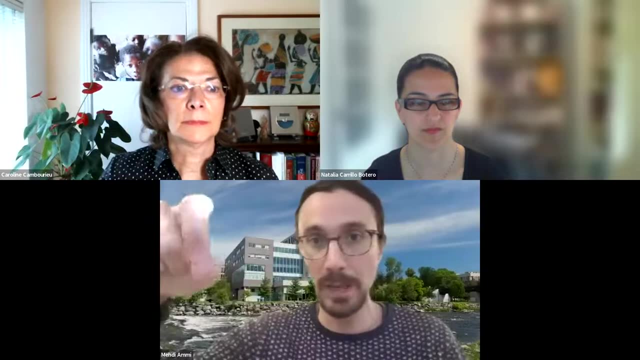 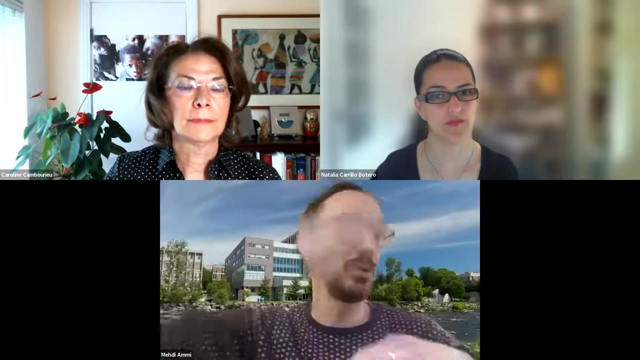 coming from municipal taxes But there has been a peak somewhere in the mid 2000s because there has been some change in the agreement between the province and the municipality in the cost sharing And then it fell down. It's not big And what I remember 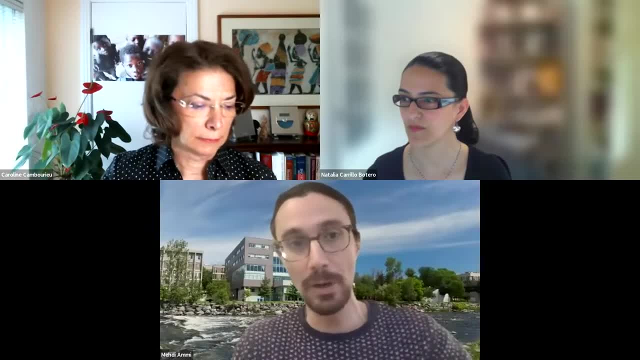 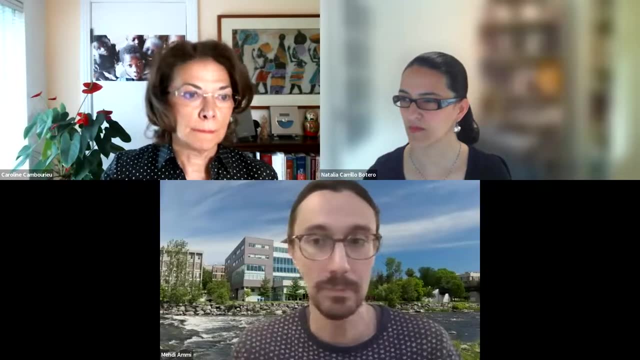 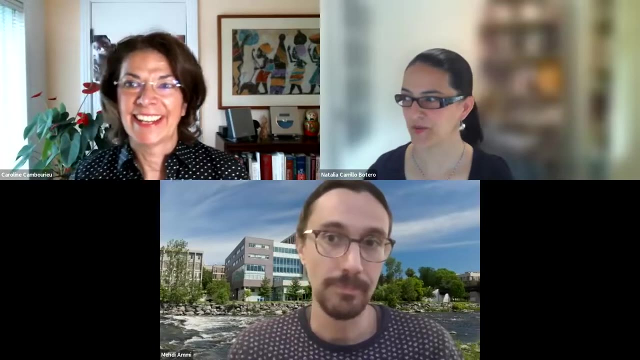 is also seeing that in Manitoba and Saskatchewan- is something that has been slowly rising. So the contribution of municipalities to public health- I don't remember the proportions, something I can definitely look into, But it's small. That's what I can say. It's small when you compare it. 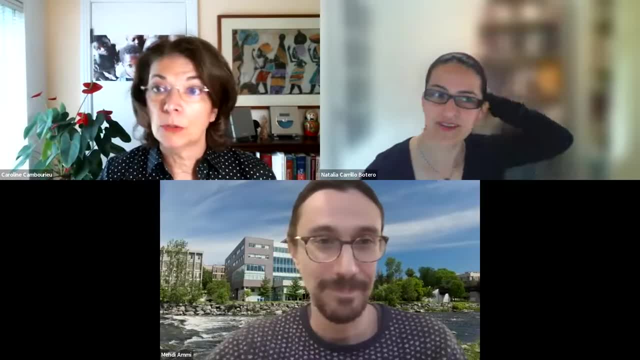 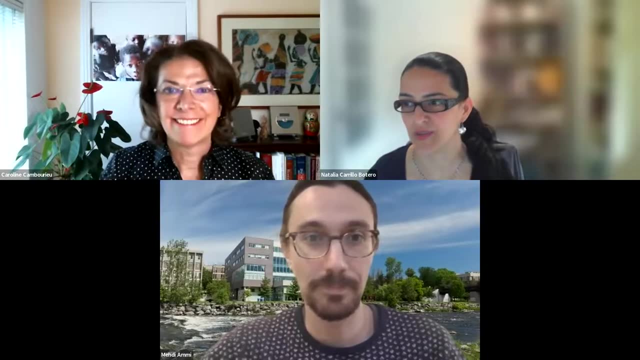 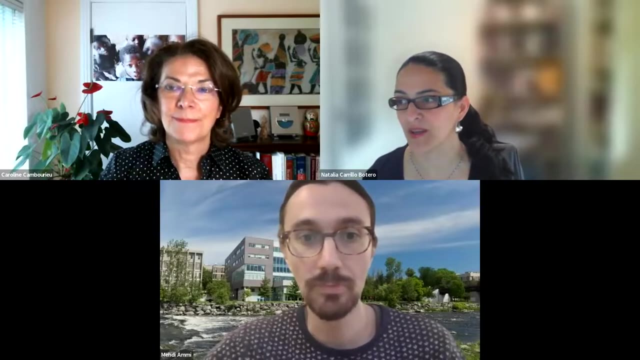 to the province contribution, which is really small, It's really high. And then you have federal, direct, which is some somewhere, let's say moderate. then you have a social worker compensation board for occupational health And then you have municipal. that is just like very at the bottom, except. 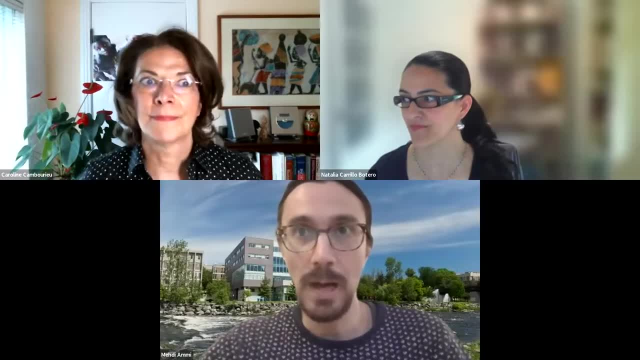 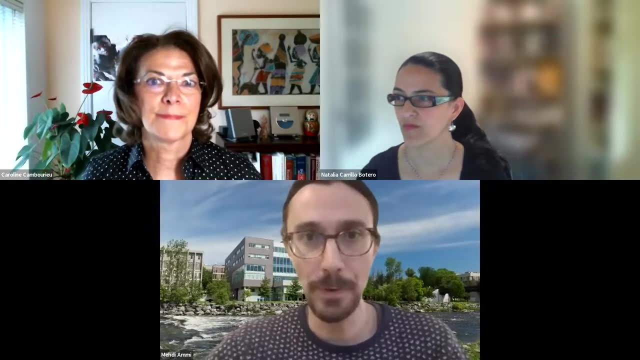 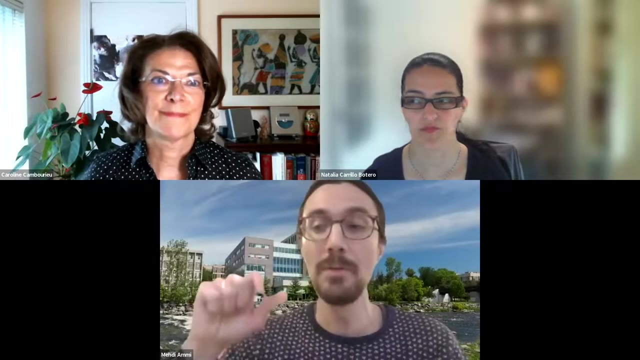 for Ontario, where again there has been, like this moment, where the cost sharing agreement has changed So that Ontario had to use more of municipal taxation to increase the public health, I mean to contribute to the public health. sorry enterprise. And then, when the cost sharing has been really, they walk back. 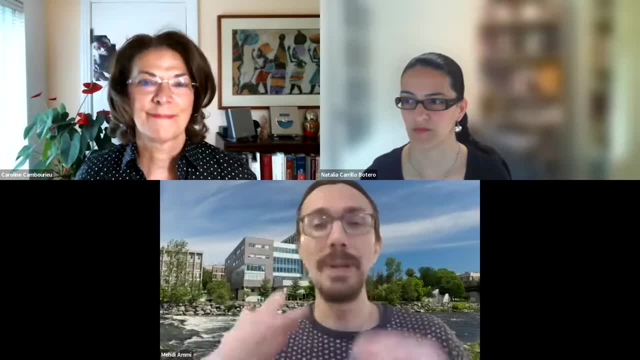 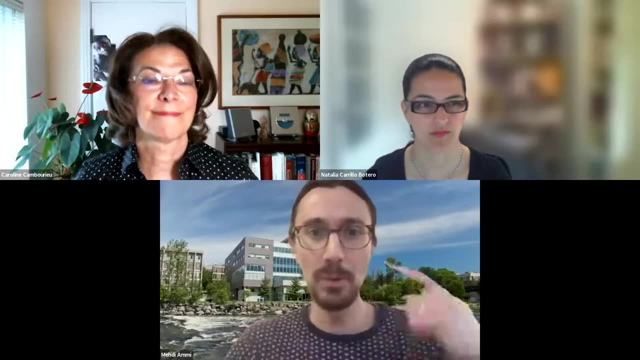 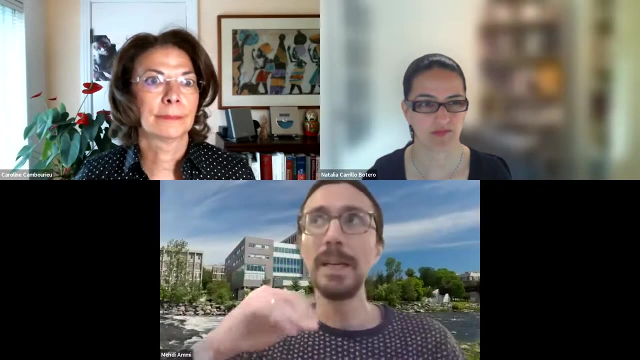 essentially from I don't know, I think, to a 75 province, 25% municipality. then they move to 5050. And then they roll back to 7525 again. Okay, so that's what I can say, Thank you. Should I continue? Go ahead? Yeah, no problem. 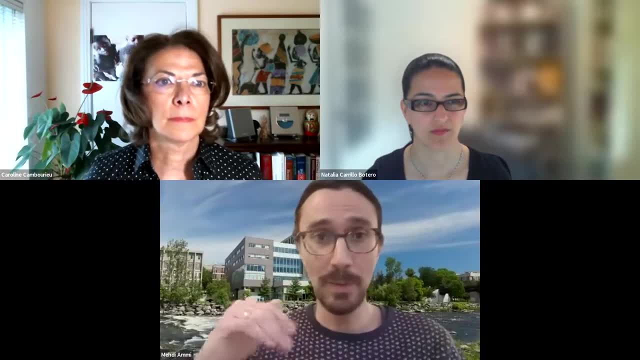 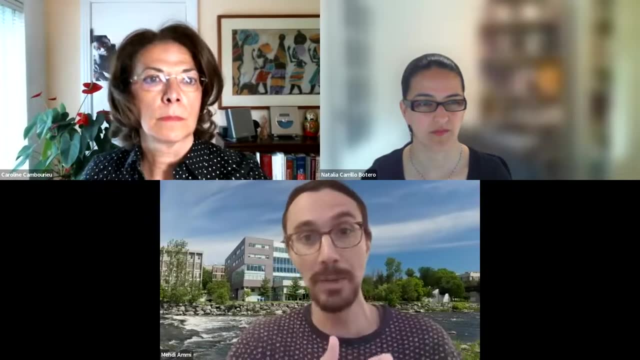 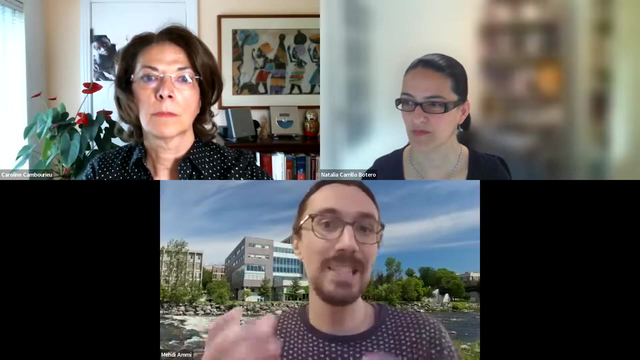 So before I move to a new question, Dr Amir, I wanted to ask you a follow up question related to our previous answer. This is related to social determinants of health expenditure. So there is a follow up question. The participant wants to know if you know of any research or policy. 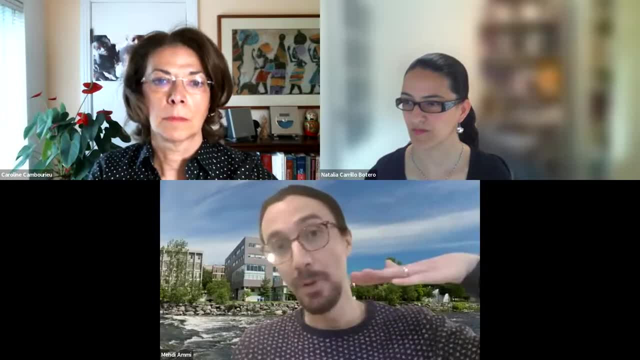 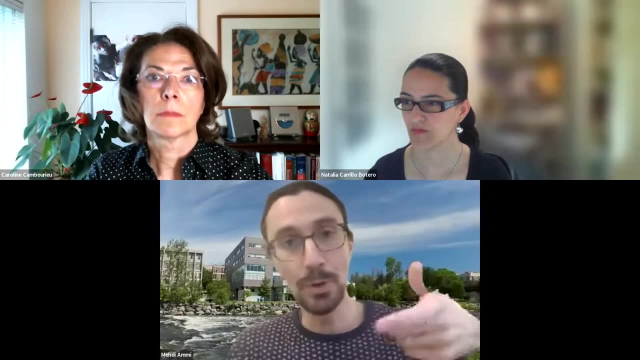 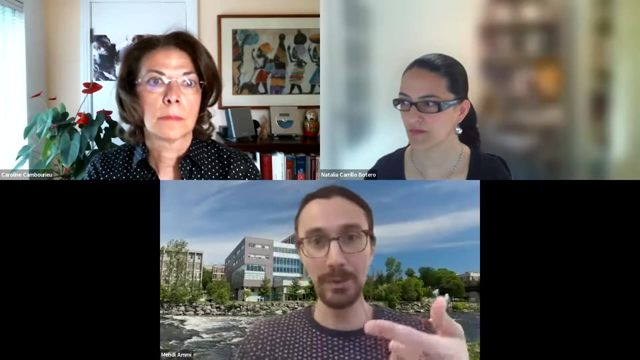 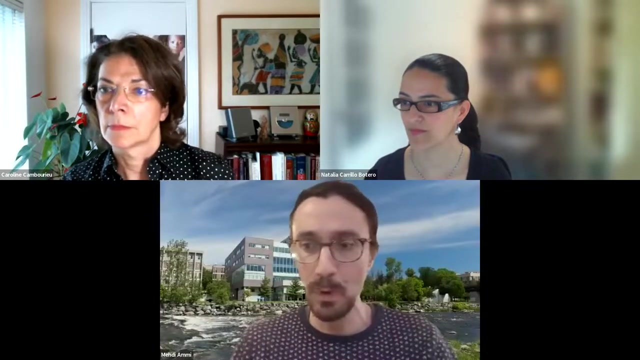 papers that look at social determinants of health expenditure. Has there been any work capturing this type of expenditure, but especially capturing the expenditures on social determinants of health, which, indirectly, are public health expenditures? Are provinces, the provinces, decreasing direct public health expenditures but increasing social determinants of health? 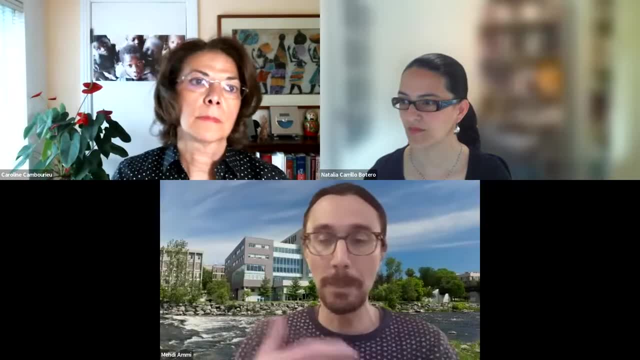 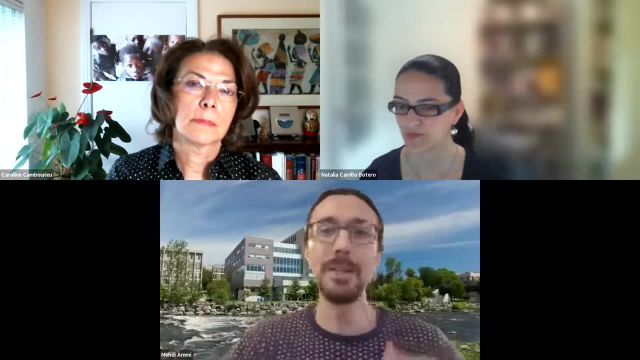 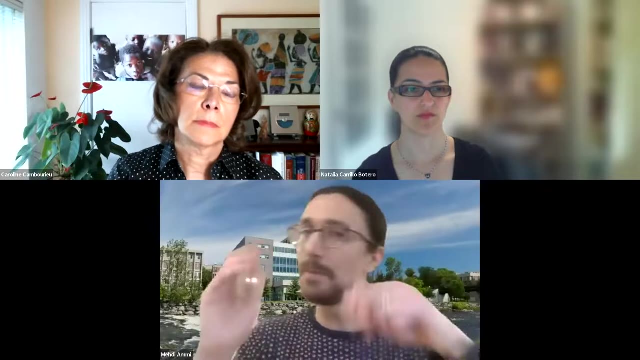 expenditures and ultimately possibly affecting public health outcomes. Yeah, So if you're aware of any sources, the participant is interested in these resources. So I don't remember seeing a lot of this kind of crowding out, because what you're talking about is the crowding out. 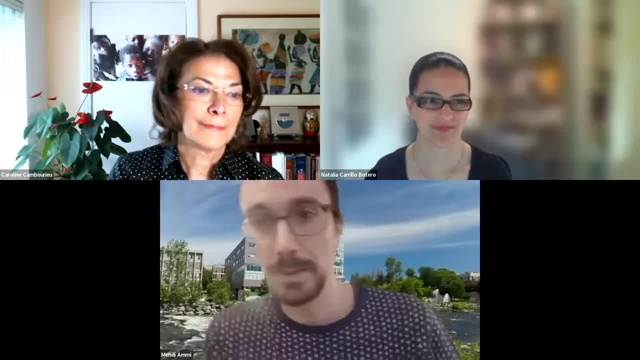 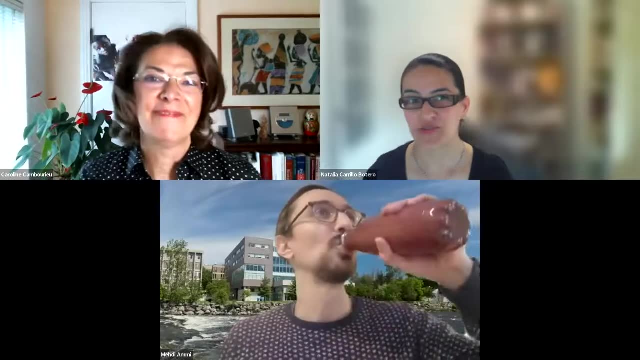 essentially I. so I remember two things: a paper. I can't remember the name of the first author. I hope it's going to come back to me before the end of today, but it's in Canadian Public Policy And what they're. essentially it's a. 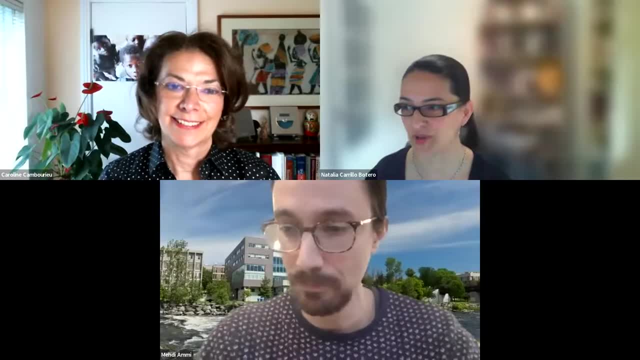 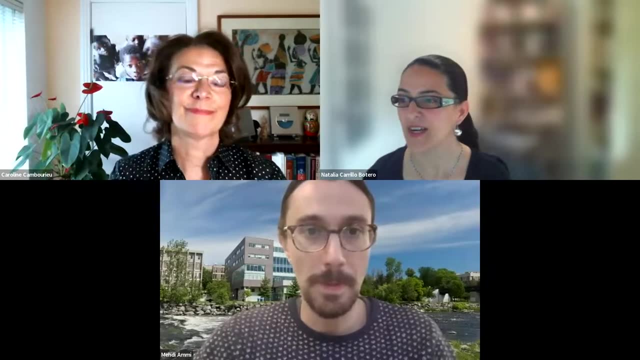 journal. So Canadian Public Policy is a journal. What they are looking is at the crowding out of different spending categories between health spending and, just like other education, infrastructure etc. So we're looking at this kind of. it was not specifically about health, it was more about 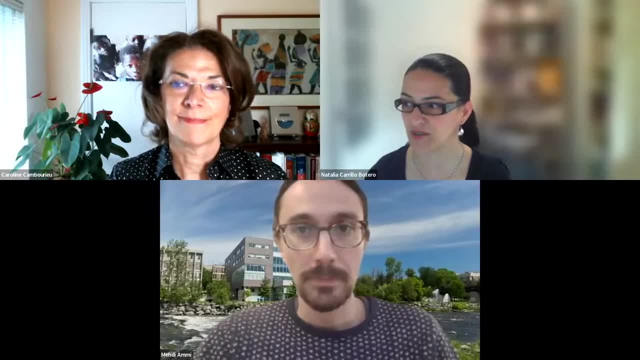 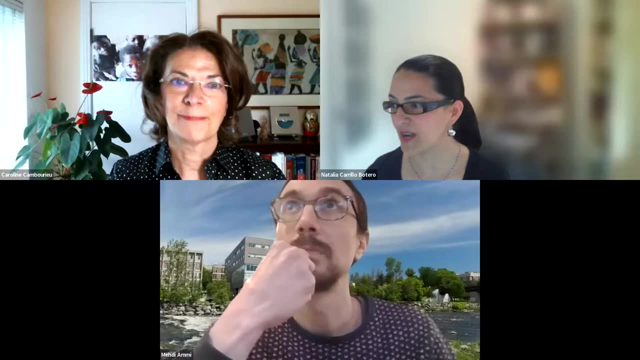 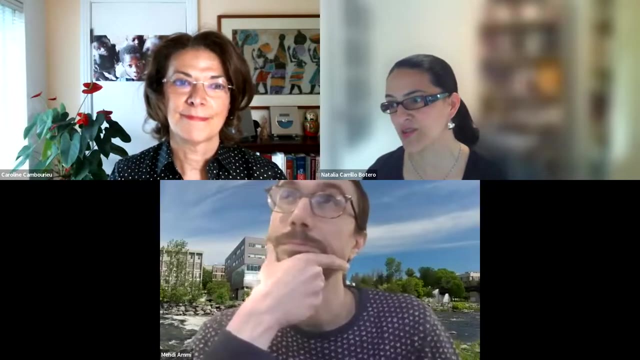 budget choices. But you know, education might be, that's part of a social determinant of health. So infrastructure, if you think about, you know, decent housing, decent access to public transit, that's part of a social determinant of health. So that's one, And there is another one. 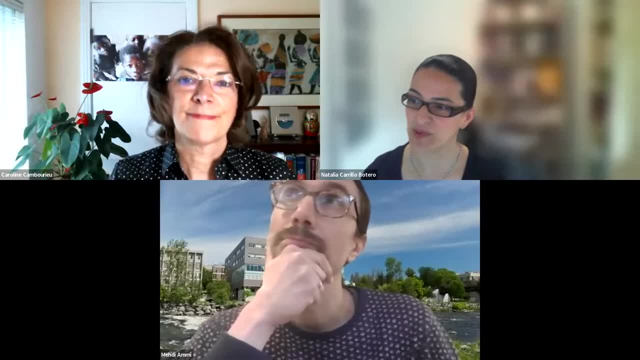 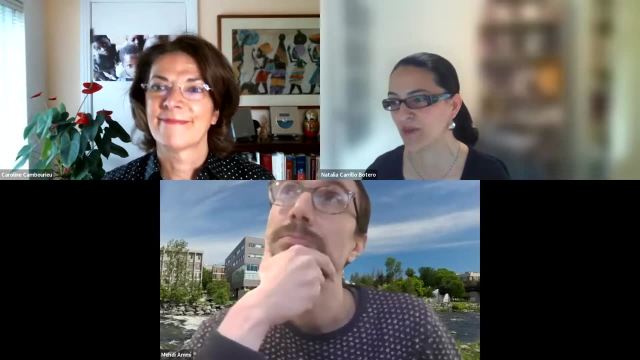 So this one. I remember the first author, Dutton, it's 2018 in the Canadian Medical Association Journal, And there they were comparing social spending, which is broadly defined- This is really a Canadian term, I'm not quite sure. It's family services, for example. 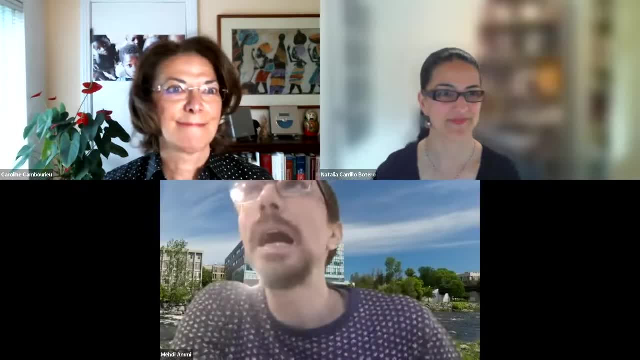 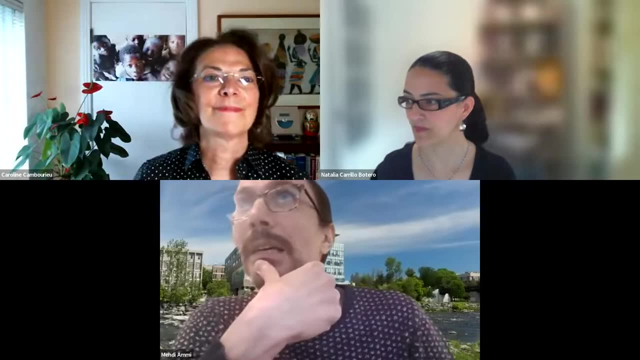 And the health spending in general and they were just looking at mortality and life expectancy And the point we're making. it's a kind of fixed effect model, But the point we were making is that the return on health is higher for social spending compared to health spending in general, So that 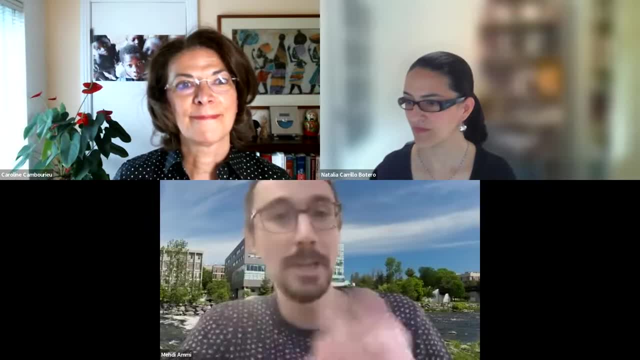 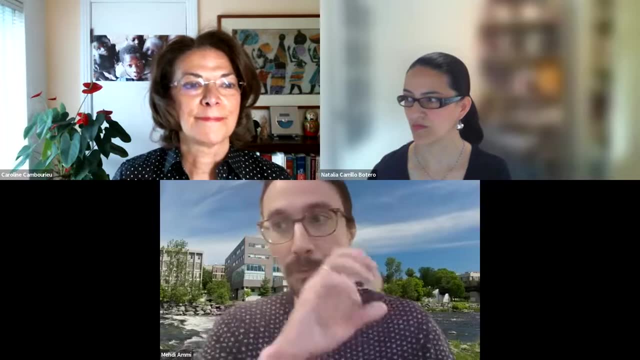 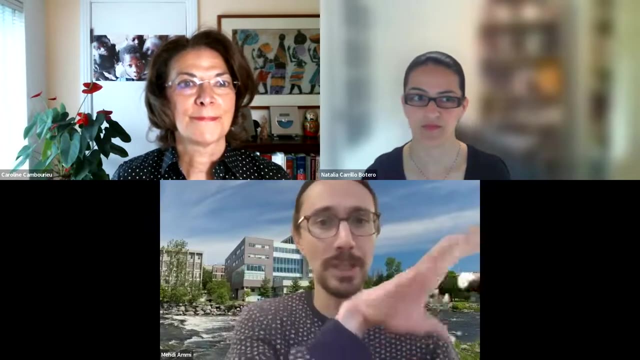 would be the two. Yeah, that's the two that come to mind. Another one, Natalia, on the side. Yes, I have more. Oh, lots of questions, That's good. Yeah, a lot of questions, That's very good. Thank you very much. 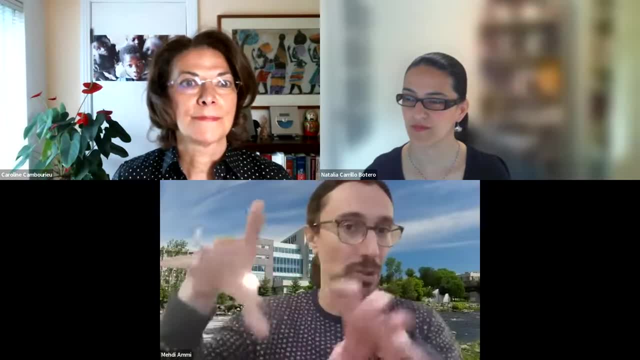 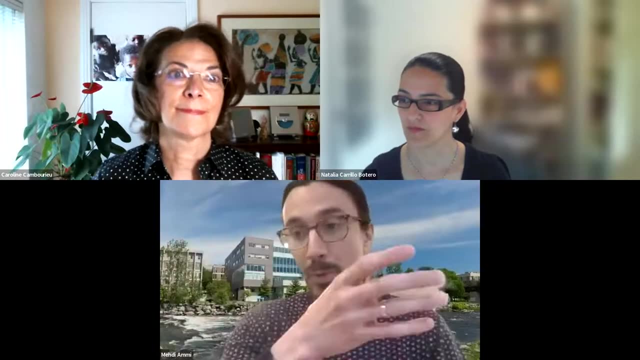 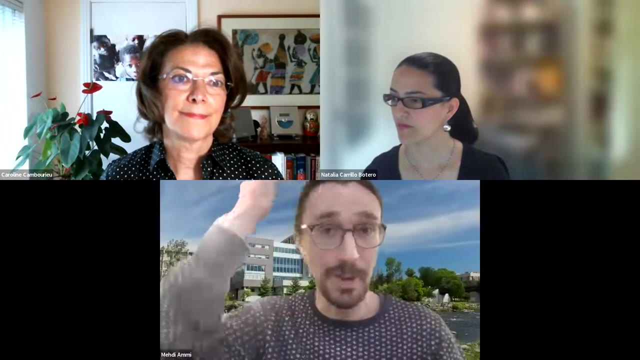 Yeah, I anticipate that we may not be able to answer them all, but we'll try. So for the PPH, I was wondering if you could provide a few examples of expenditures, including the PPH index, that could be clinical in nature versus health promotion. 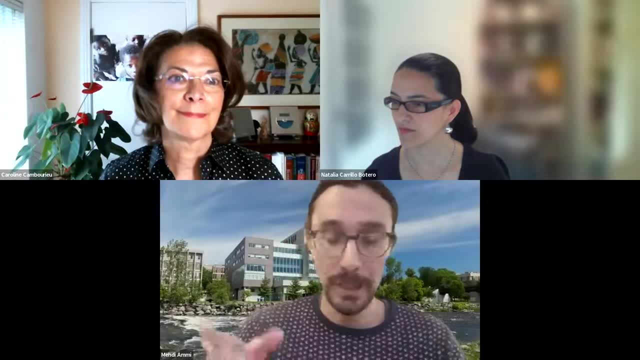 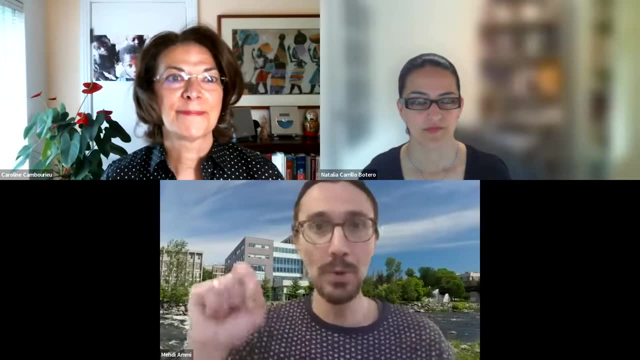 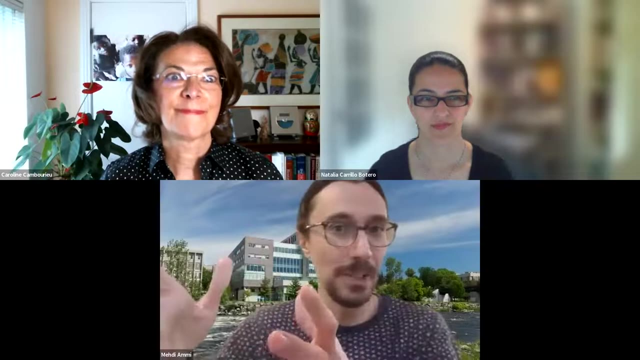 and disease prevention activities, just to get a sense of what might be lumped in there. Yeah, absolutely So. the PPH index is the PPH index, which is the PPH index that is understood as public health, scope of practice or external to it, And the person clarifies: I: 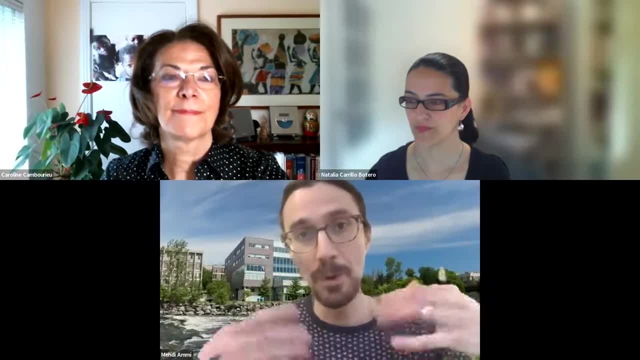 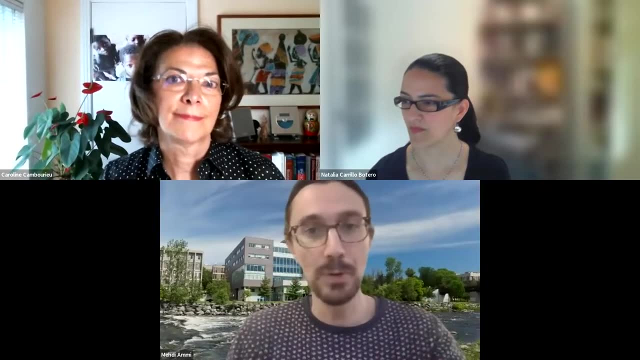 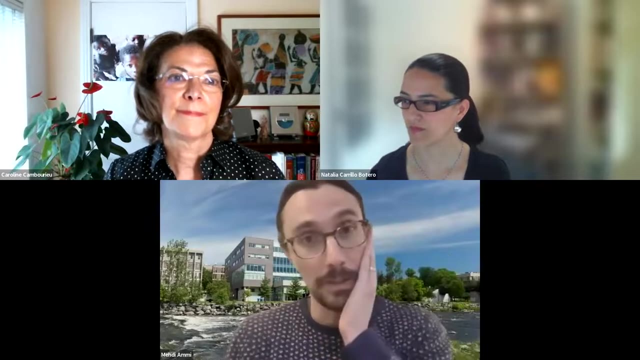 completely understand the variability and the complexity of what is included in that category, The definition of public health being so hard to pin down Like mammograms, that would be something that is public health because it's prevention And that will be in the PPH category. 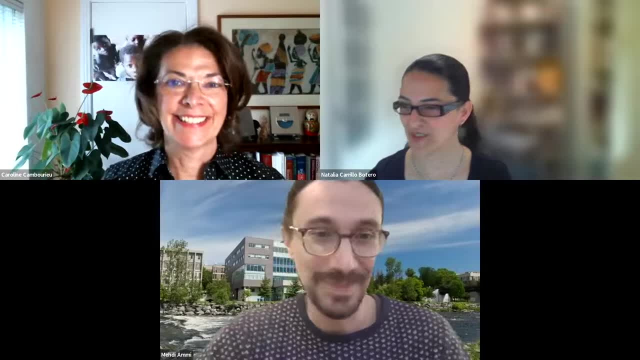 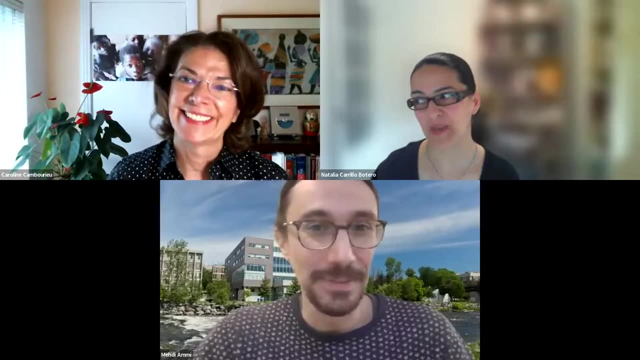 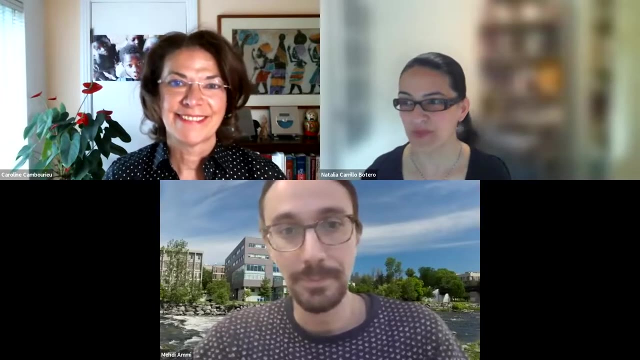 So that's going to be one example of what could be there. I'm sorry I forgot the second part of the question, Natalia, Sorry, sorry, I'm back. Let me just go back to it. It was a long question. 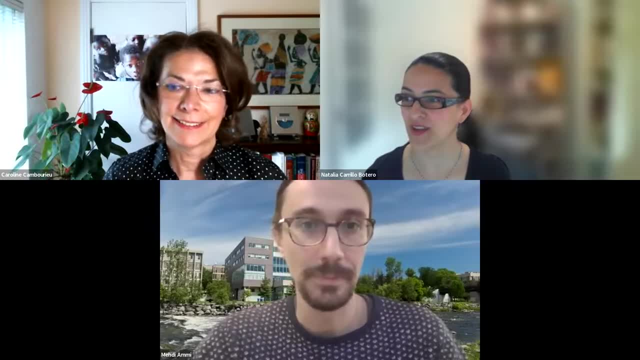 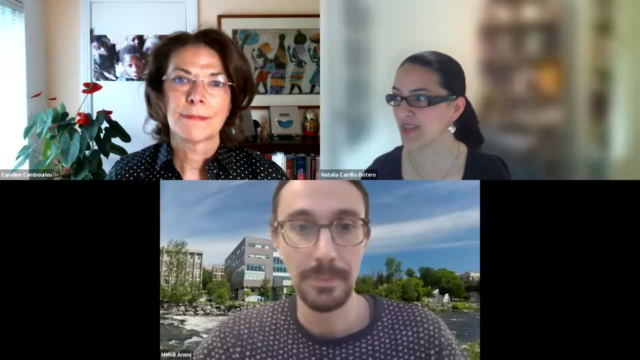 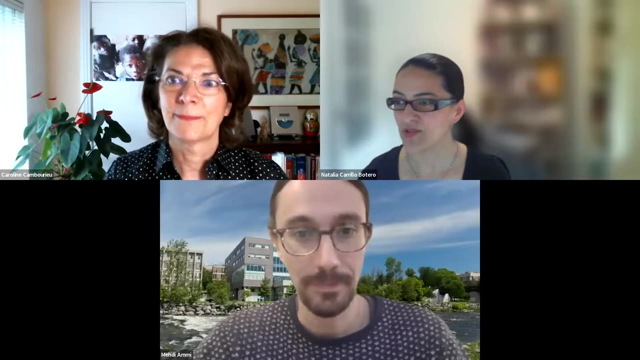 Yeah, exactly That's the end. Sometimes it's difficult to remember all you know. Oh, I seem to have lost it in the chat. I'm sorry. Maybe we could go to the next one. Let's move to another one and give me five seconds to find it again. 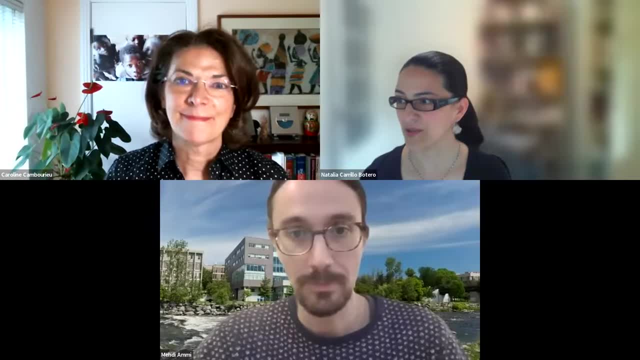 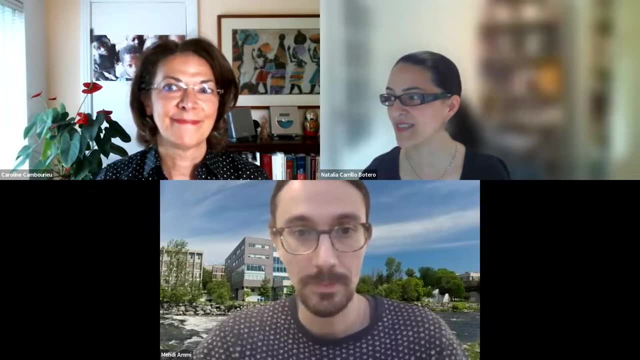 OK, well, I could go with a very well, very quick question. Maybe concern about the indices? What are the advantage or disadvantage of working with public health expenditure indices Instead of dollar value? you know you are using indices in your study. 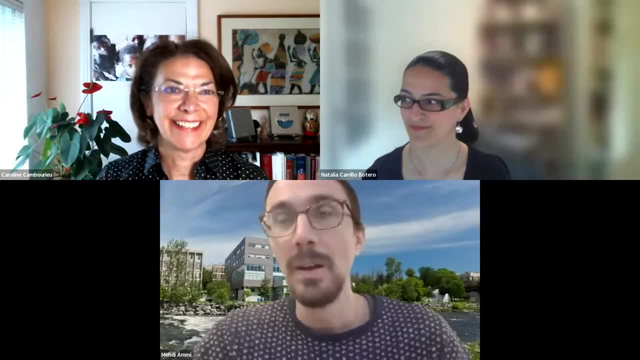 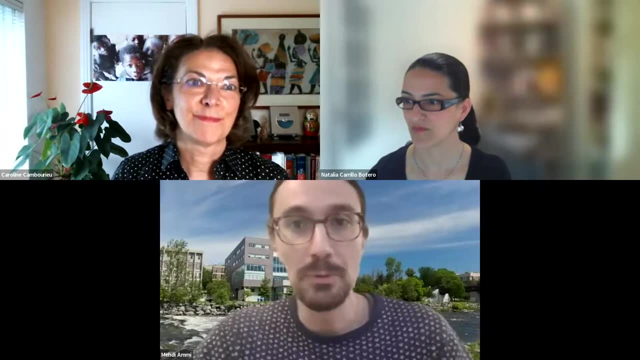 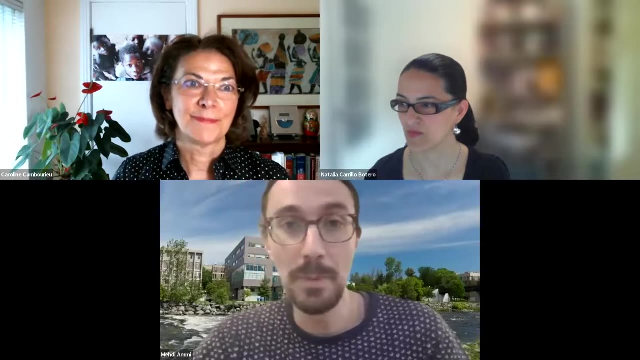 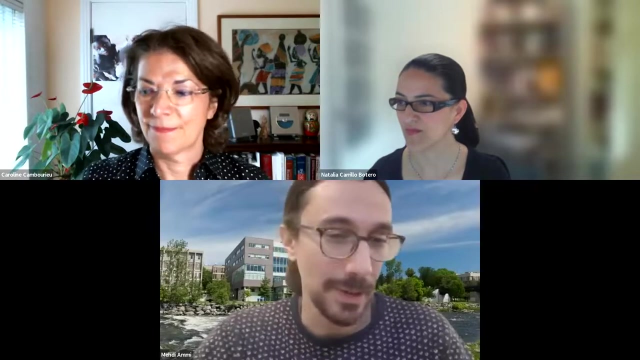 So So we've been trying to come up with a way just providing a message in the simplest possible fashion, because we're focusing on growth, we're thinking getting indices instead of getting the per capita amount would ease the comparison between the two. 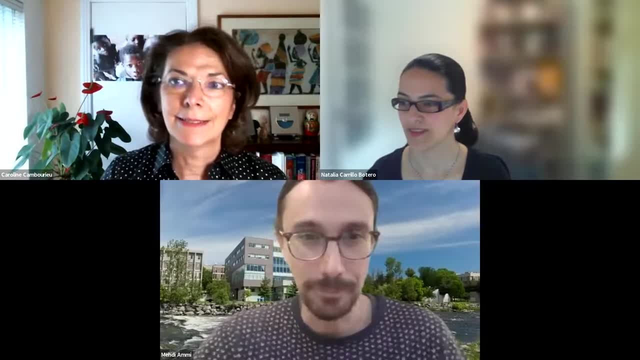 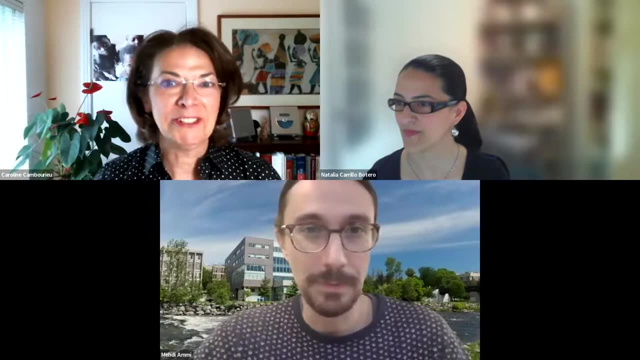 So, if you look at the different categories- because if you look at, you know, for example, in Quebec 2018, it's about $100, something like that- There are $1,000 per capita And it's no, it's $100. It's $100. And it's about 10 or 12 times bigger when you look at physicians, about 15 times bigger when you look at hospitals. And then we just add that, you know, when looking at the different provinces at the same time. 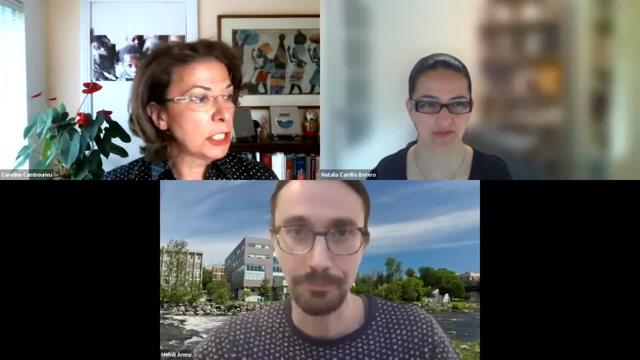 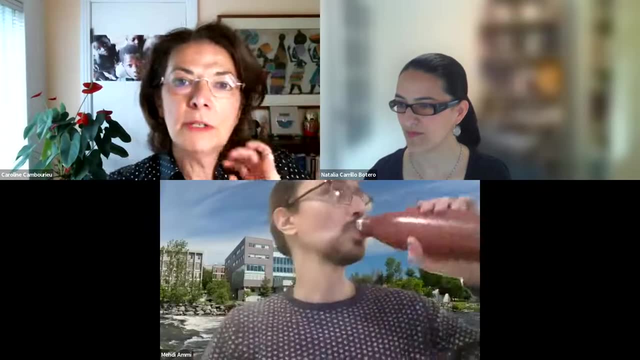 It's easy, It's a bit hard to wrap. One says around that. So the advantage of using the indices is just to try to simplify this information and get a sense of growth. and we see the growth. We just look at the number and we get. we know what we talk about. 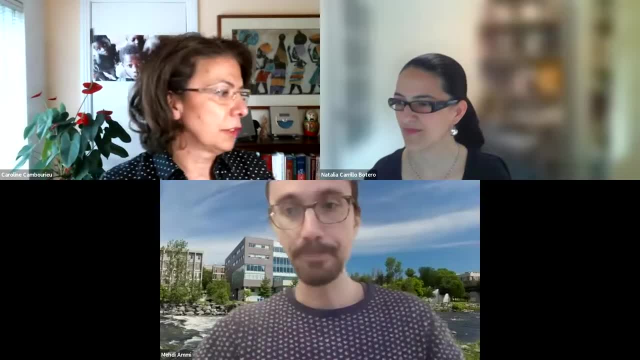 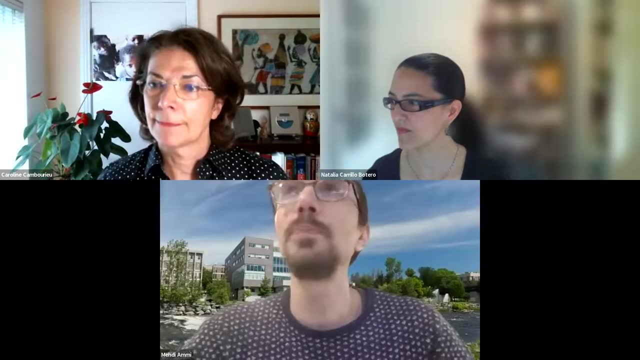 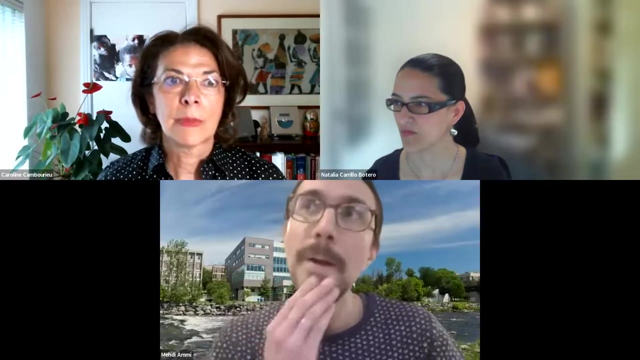 But the disadvantage, the challenge, is that well, we don't. We lose track of how much money is actually spent there, and that might be an important information, especially if you think about you know How much exactly is spent and whether this is this seems small or not. 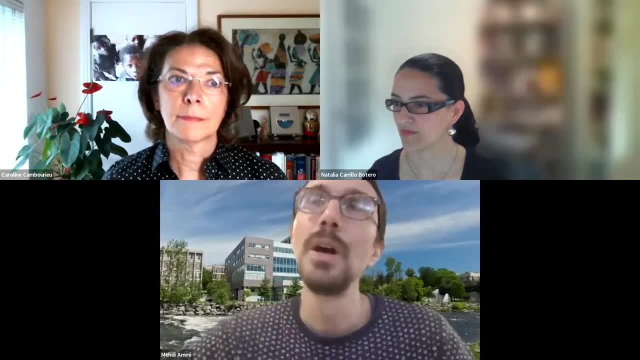 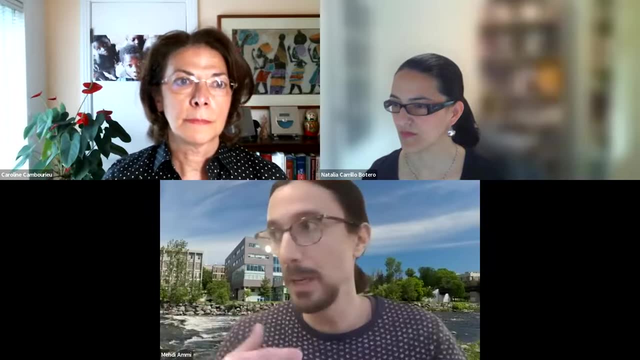 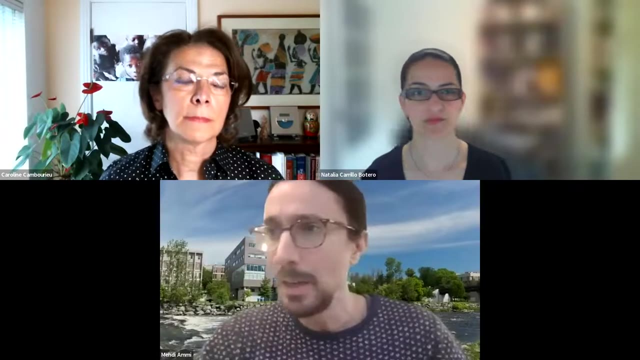 So that would be the kind of balance between the two, But I guess we elected to get to this summarized number but provide the information we want to convey, which is about comparing growth. Okay, thank you, Andrea Natalia. sorry, I was looking. 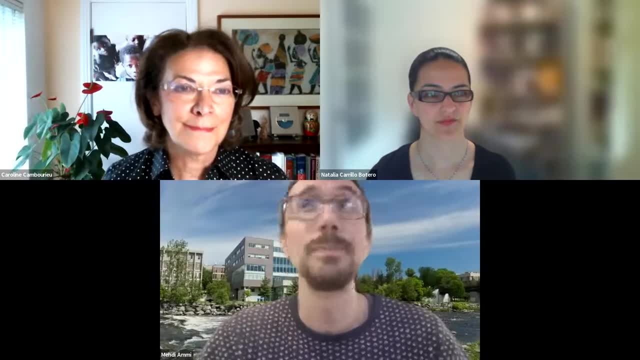 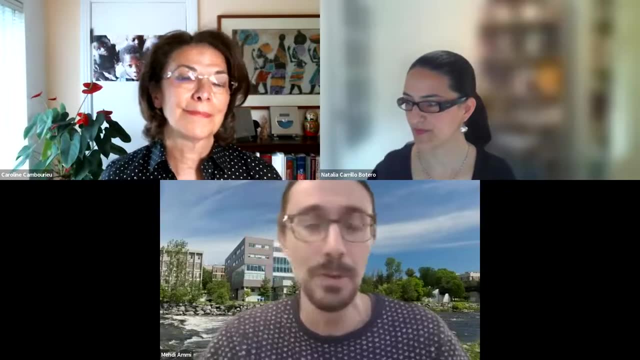 Do you have another question? I have one. Do you have another question? Do you have another question? Should we move on to another question Or do you need to move on? Okay, We have a few more minutes. Two more minutes. 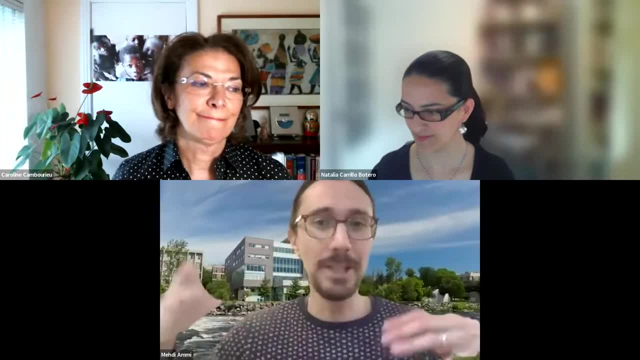 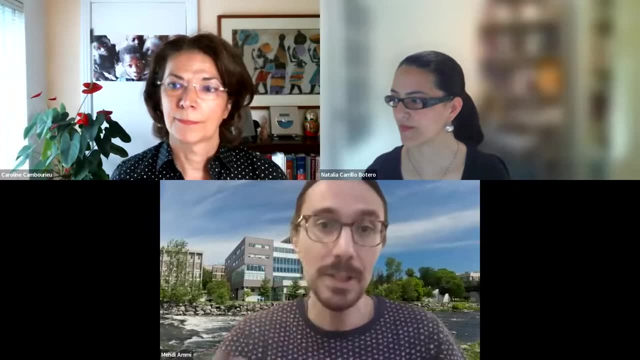 So we won't be make it. We won't make it, But let's try. So is it possible to separate out public health crisis spending, for example in COVID, from other ongoing spending? Wondering, I'm wondering if we will see a COVID bubble versus a sustained spending. 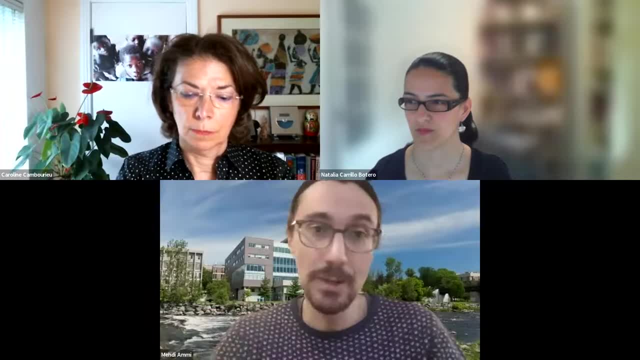 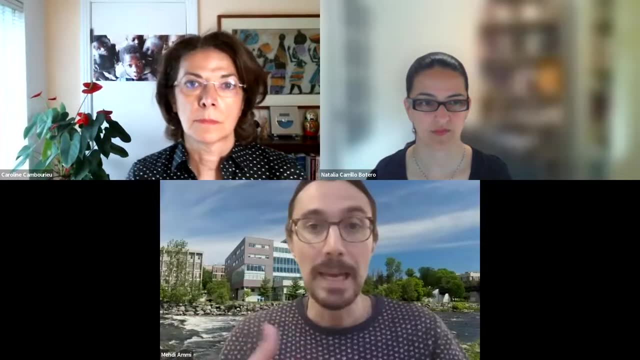 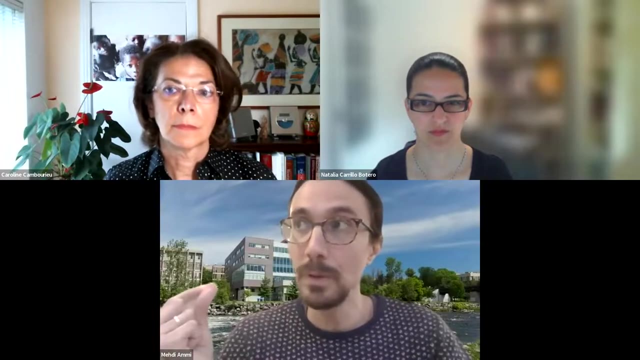 I also wonder if Spending on other things like CERB can be captured as part of COVID spending. Okay, so first part: can we separate public health crisis versus ongoing spending For the past two years? we will be able to do that using CHI data. 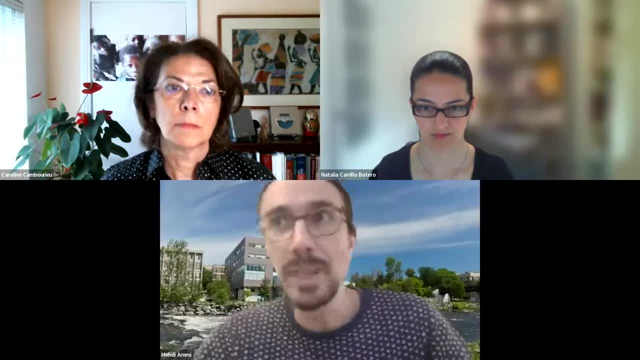 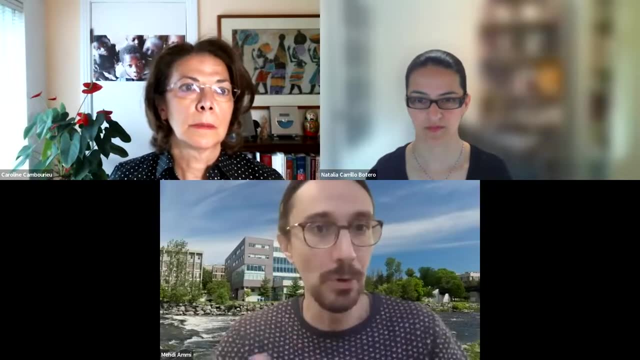 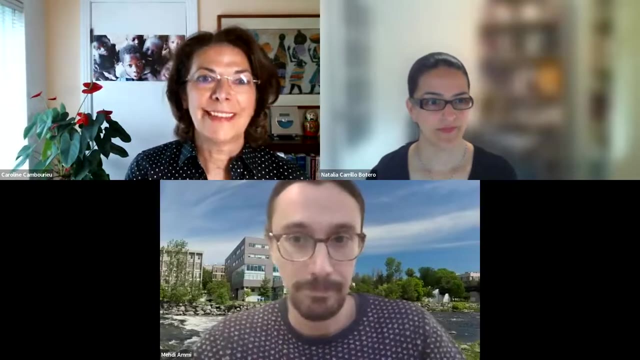 because they created this COVID category. So that is giving us a sense of what is public health, let's say steady state, and what is public health crisis period, Even though it's focused on COVID. The second part is: is CERB part of the COVID spending? 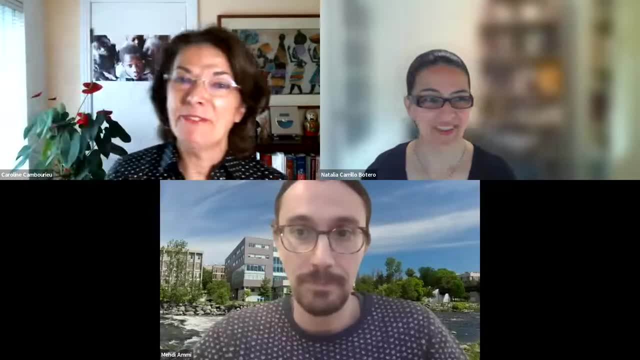 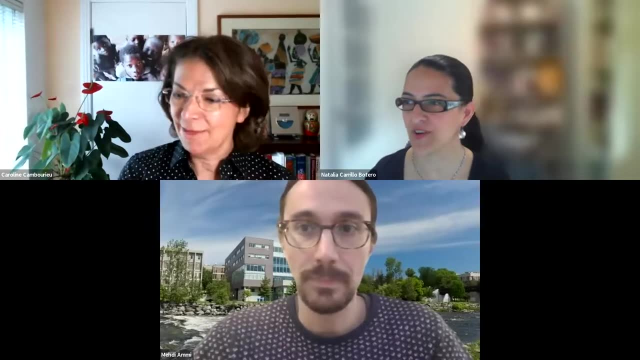 at least from the CHI perspective. No, I don't think so. I think the CERB is just going to be this amount of CERB. this is this kind of financial support that has been provided by the federal government as a kind of relief for individuals. 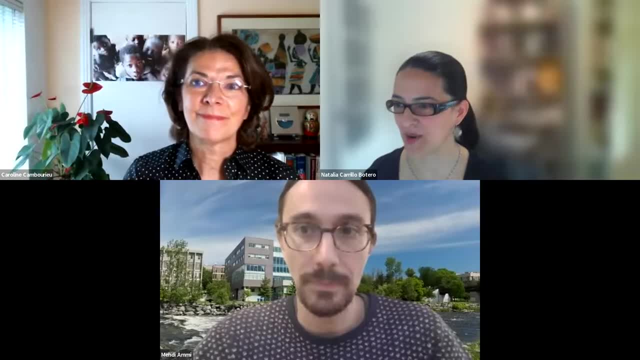 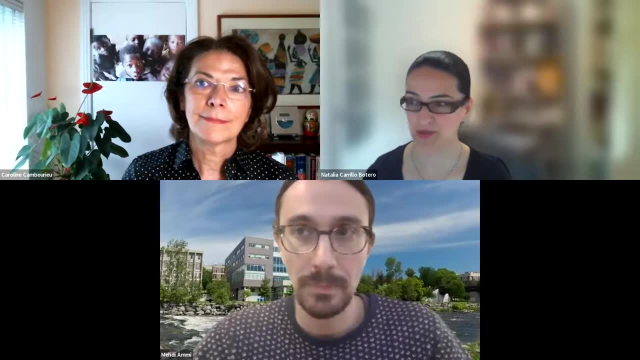 whose income has been affected by the crisis because they lost activity or lost job. So it's not part of the COVID support. but that goes back to the question about what is public health. What is public health Is like? for example, income support part of public health? 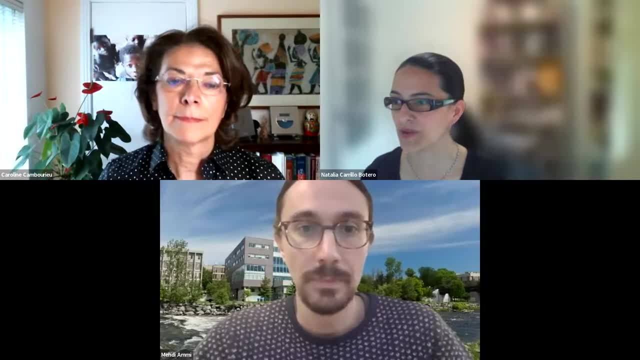 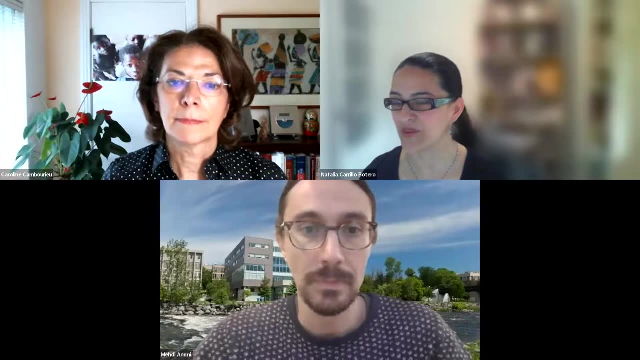 I don't know, And I know that the definition we adopt is not this one, And this is not the definition I want to adopt. I prefer to stick with a more narrow definition, just to make a case, The more if the input is the same. 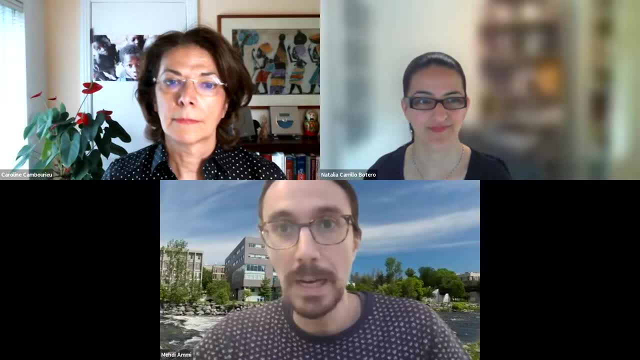 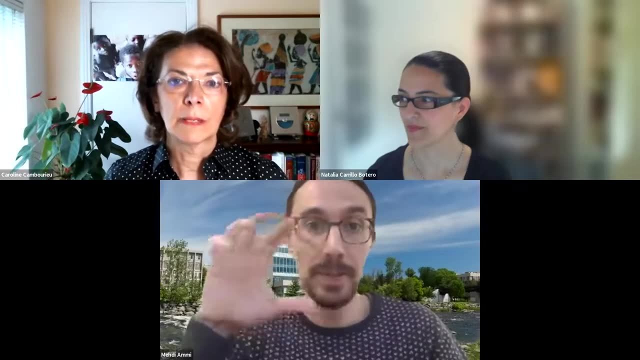 if the output is the same, you put a higher level, you are just going to obtain less per month. So if you just say, well, income support is part of public health, let's see what happens. And my view is that again, I reiterate- 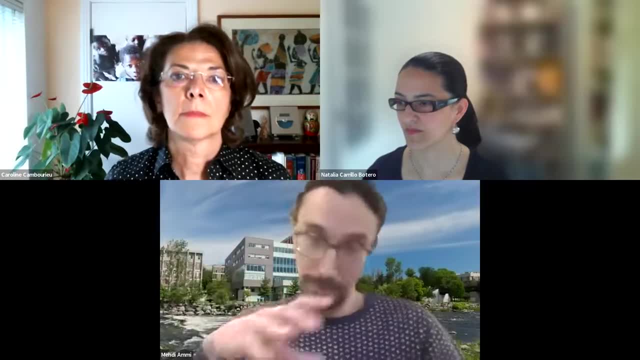 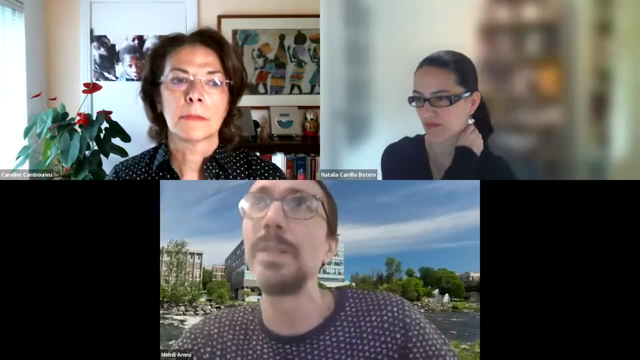 I don't think this is the way to go if we want to promote investing more in public health systems when what we see is that Canada is already the top spender- I mean, it's wrong to say top spender- The country that allocates the highest share. 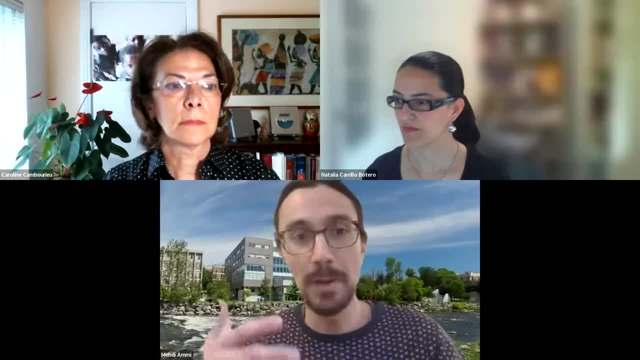 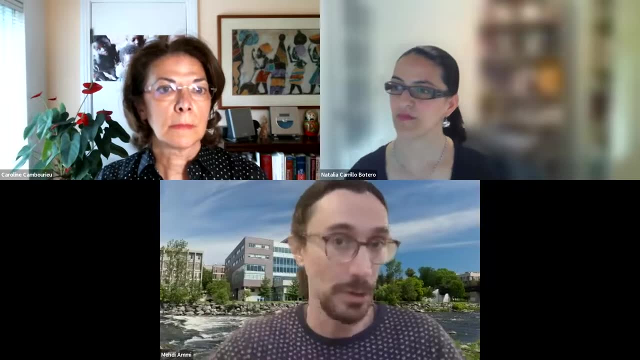 of its health resources to public health, and that seems that, except Quebec and Nova Scotia, there is a large growth across the board. So that's my view. Thank you, Mehdi Natalia. we have time maybe for a last question before we close the webinar. 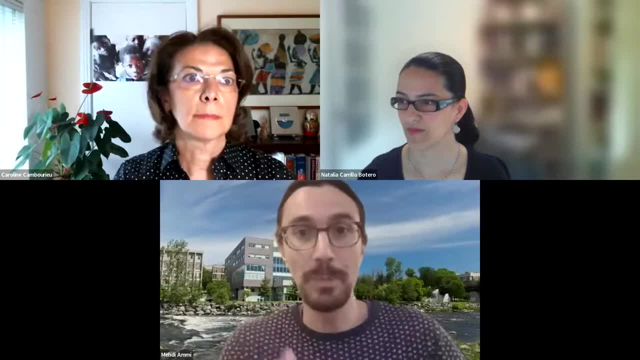 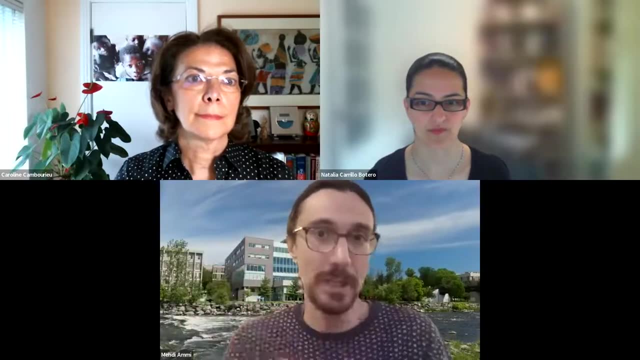 So you can go ahead. Okay, so we have time for one more question. So thank you all. We had so many Yeah thanks. This has been so interesting. So what are the factors driving growth in public health And how do they compare to those for other health? 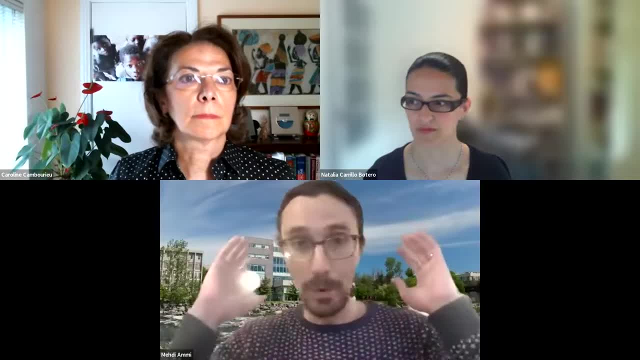 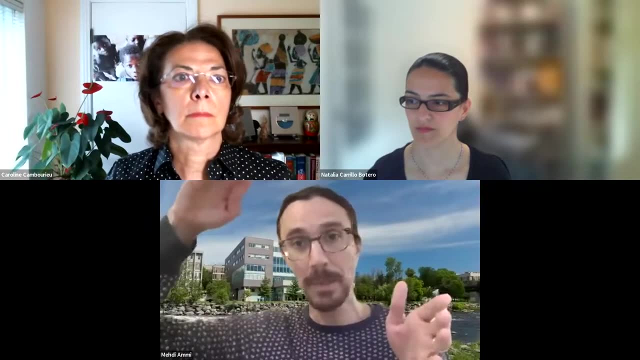 health spending components. Yeah, thank you for this question. That's exactly the other paper we're doing, So that's the paper with Olivier and colleagues. So we are doing exactly this exercise, but we focus on political determinants, so proximity to election. 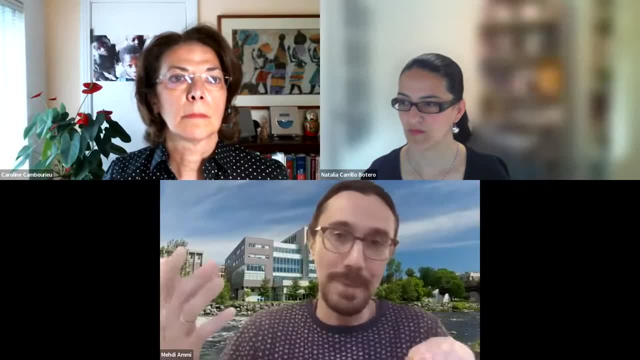 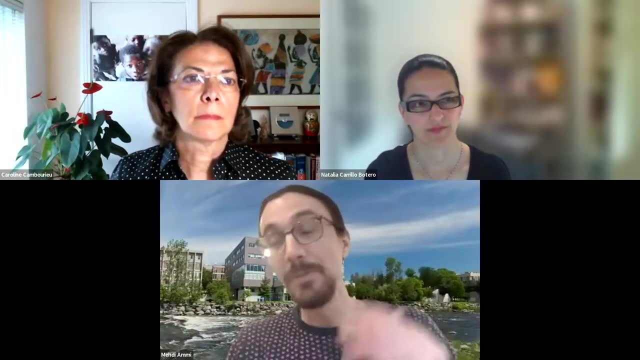 by ideology of the party and fiscal determinants. We know whether there is like austerity, rise in debt charge et cetera, And because this one is closer to the end, I can say a little bit about it. It's going to be again present at a conference. 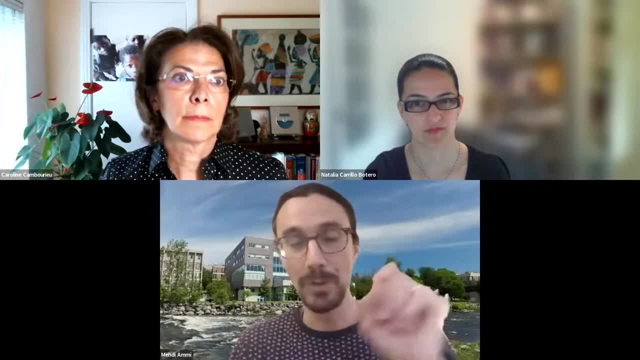 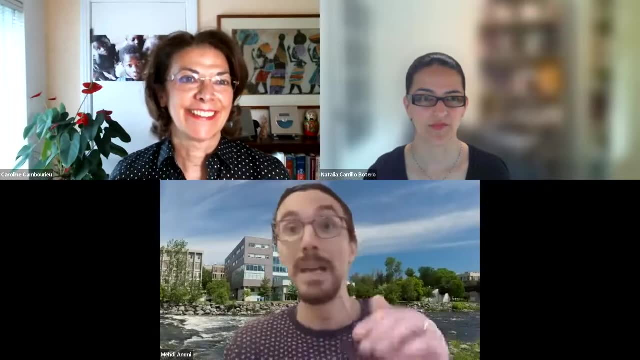 I forgot where. But we don't see a differential treatment of public health and creative spending. So we just say: let's look at public health, Let's look at creative spending from public source And we take the degree of their physicians, hospitals and drugs. 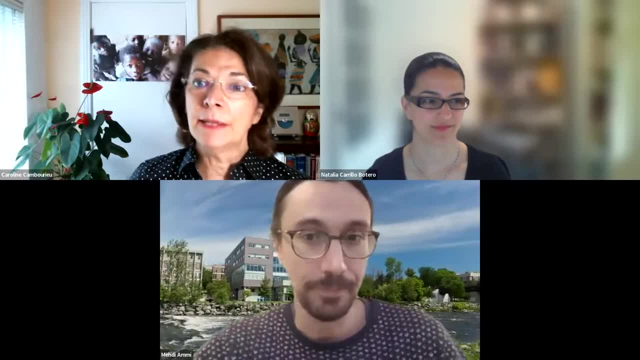 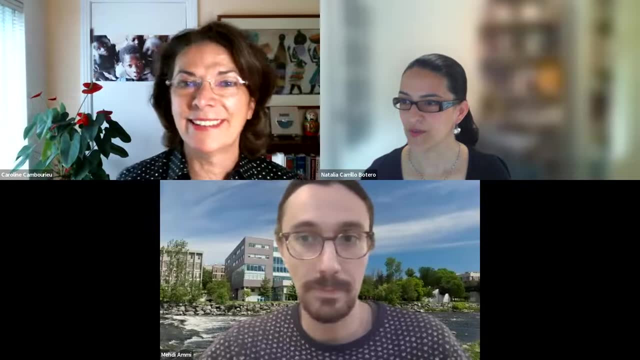 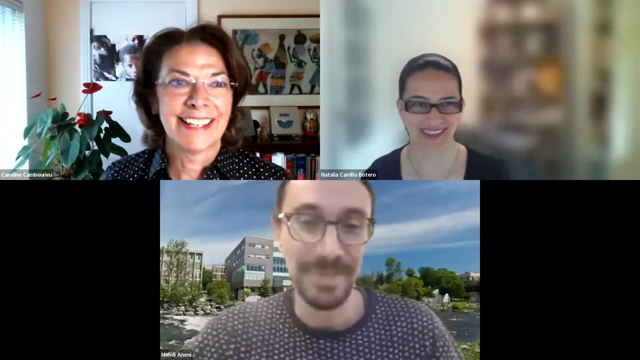 And we're really thinking about public health. because of this quiet policy that is providing results, in the long run There might be less- I mean more sensitive, sorry- to gaming from political. We don't see that at all And we were thinking that especially because that's what. 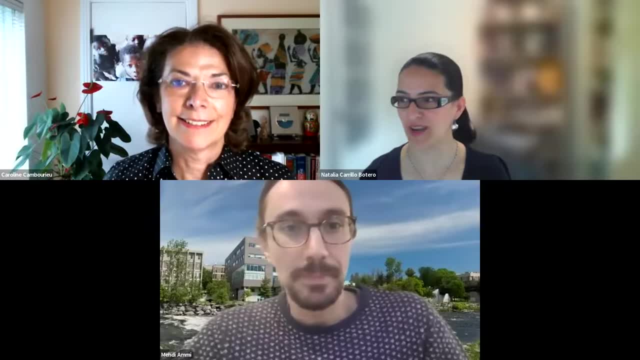 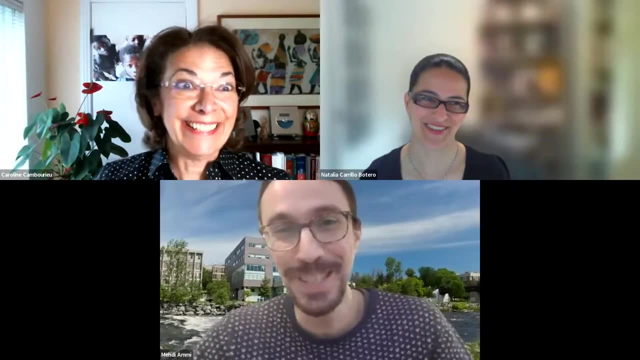 it's a descriptive paper, but the Bernd Rachel paper I mentioned at the beginning of the presentation in health policy we're really saying that in Europe, because of austerity, public health has been cut very hardly. We don't see that in Canada. 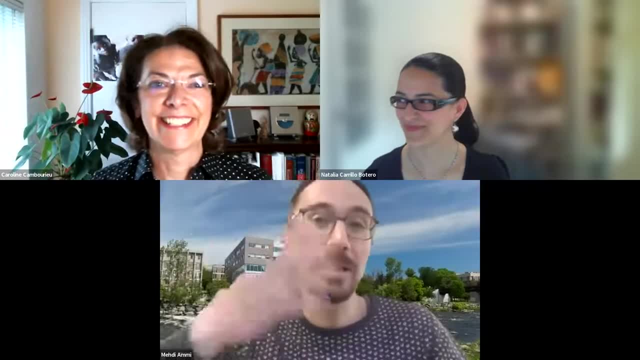 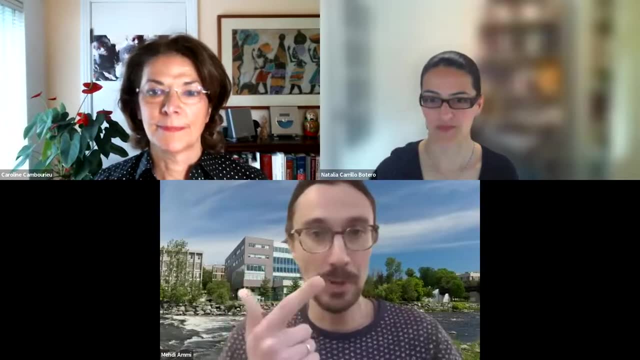 When there is austerity, both public health and creative spending go down, but public health spending go down at a lower rate than creative spending. So we're thinking about that. The thing that we note that is interesting, that speaks to this idea of crowding out, is that if you say: 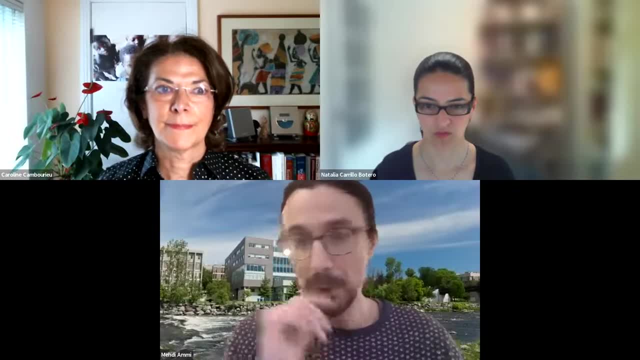 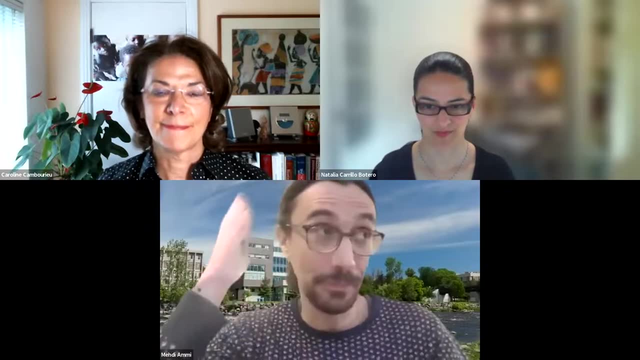 you have a health budget. that is fixed. in this health budget you can allocate part to public health, part to creative And you look how much was committed to creative care in the previous year. This is going to limit the growth of public health in the next year. 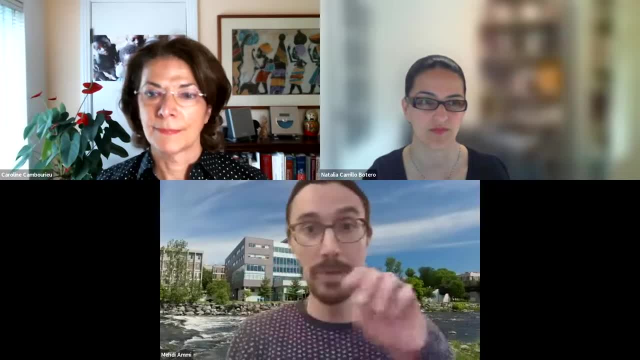 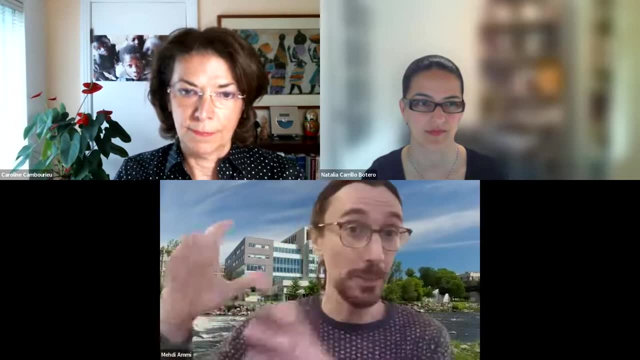 So essentially the key determinant there of public health growth it's not vaccine, It's not so much, but it's not differentially politics or austerity. It is whether a lot of money was already coming, whether a higher share of the health budget was already committed to creative. 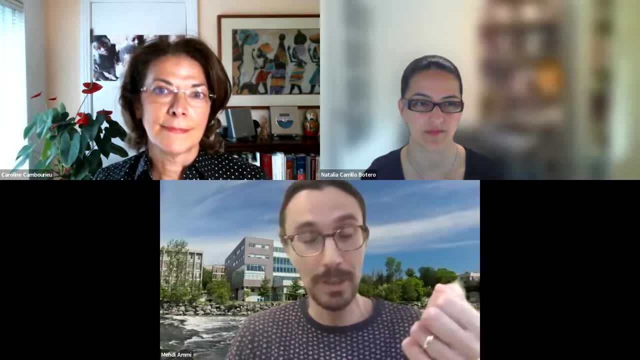 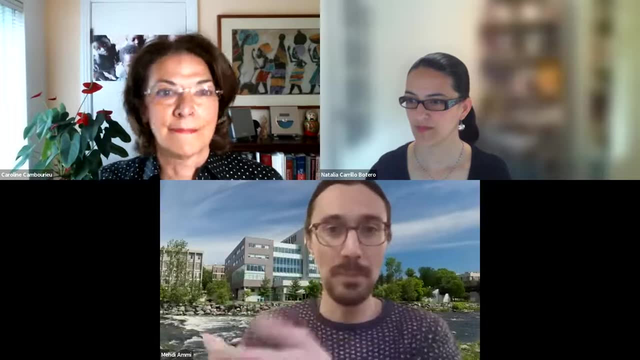 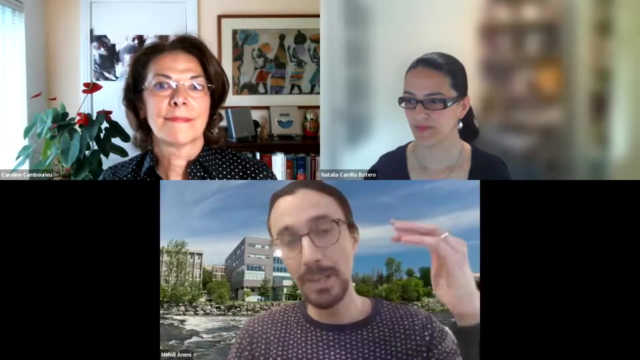 care in the year before. So that just speaks to the potential crowd out of creative care toward versus public health. So it's about time we are already done what we had to do. Thank you very much for all the participants. I will share my screen to go to my last slide. 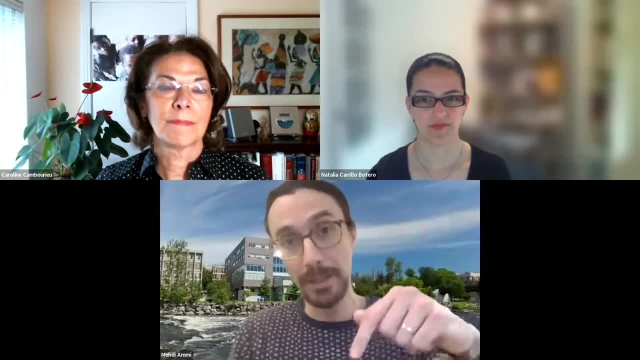 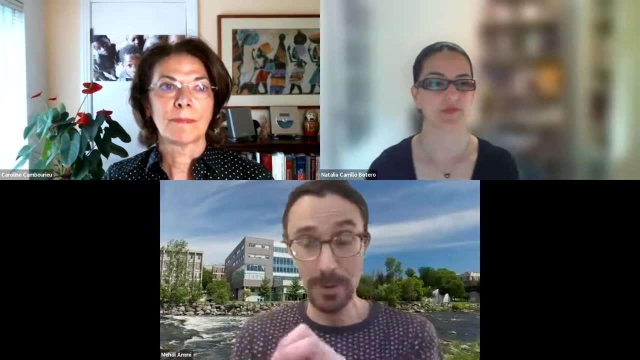 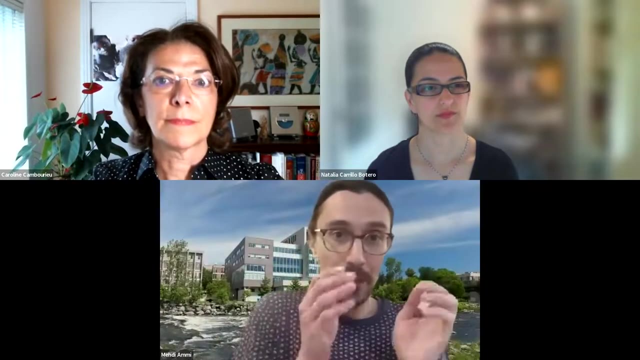 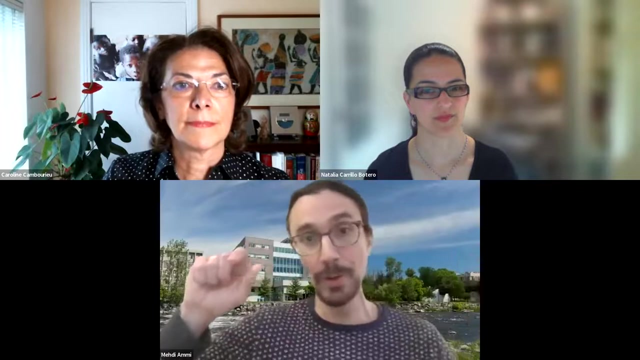 Thank you for the questions. That was great to have this engagement, So. so thank you, Thank you to all of you. In conclusion, I wish first to foremost to thank all of you for your participation, and a special thanks to our inviter speaker, dr. 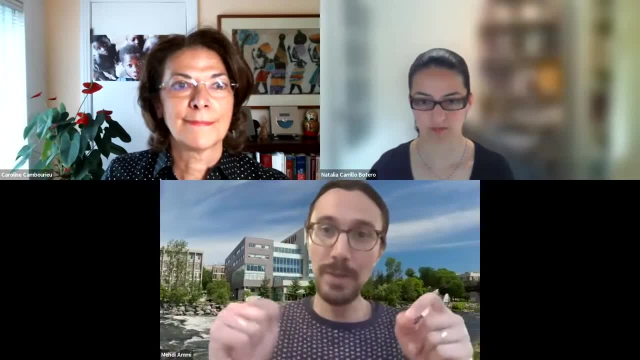 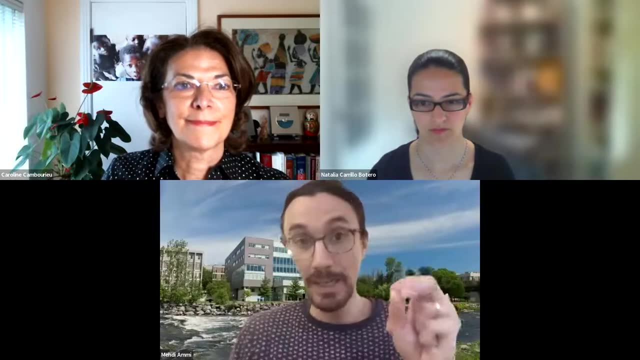 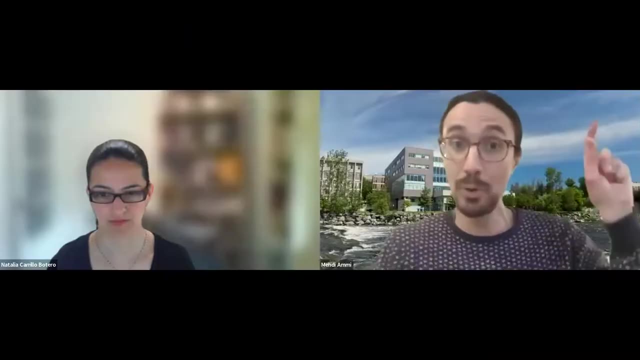 midi and me. for those interested in this topic, i invite you to read the article we talked about. for our part, at the ncchpp, we are hosting webinars on different aspects on of public health and of public health systems in canada, so i invite you to subscribe to our e-bilton to stay informed.